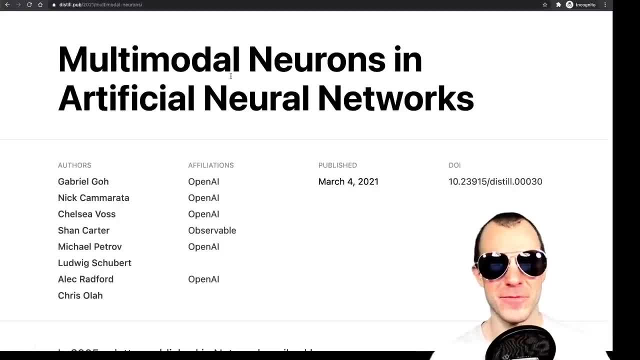 Hi there and welcome back my dear fellow scholars. Today we're going to look at multimodal neurons in artificial neural networks by Gabriel Goh, Nick Camerata, Chelsea Voss, Shan Carter, Michael Petroff, Ludwig Schubert, Alec Radford and Chris Ola. that has appeared in this Distill Pub journal, which I 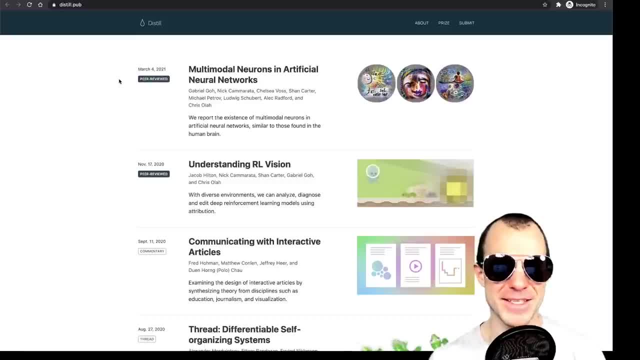 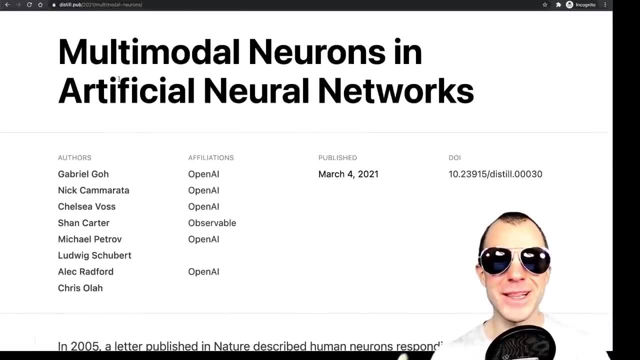 think is a pretty cool journal going beyond the classic PDF publishing. So this paper is an investigation into the new CLIP model by OpenAI and specifically the discovery of what they call multimodal neurons in this model. So this is an investigative work. They work with visualizations. 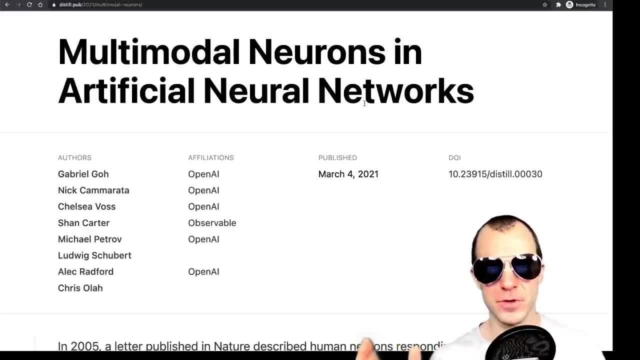 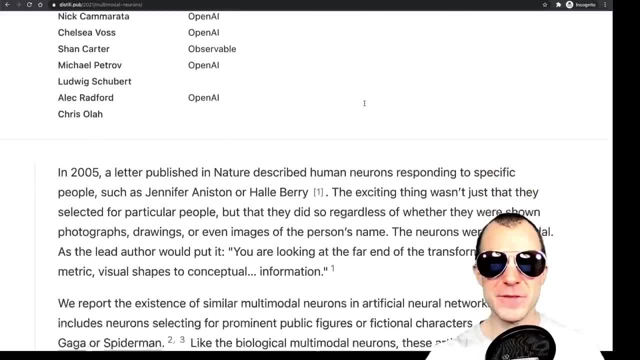 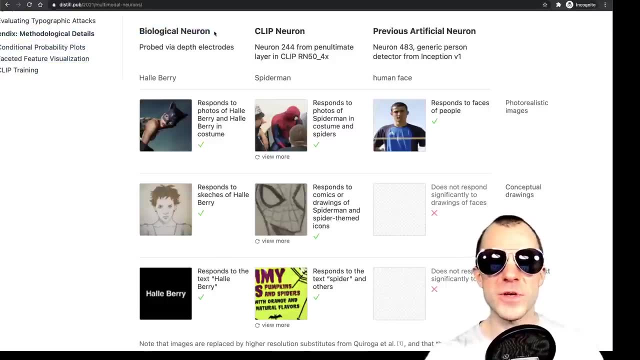 and I've made a video about both the CLIP model as well as the feature visualizations that has appeared previously. So safe to say what they are claiming as the high level claim here is that in biology we sort of expect there to be neurons that respond not to individual patterns or to individual words. 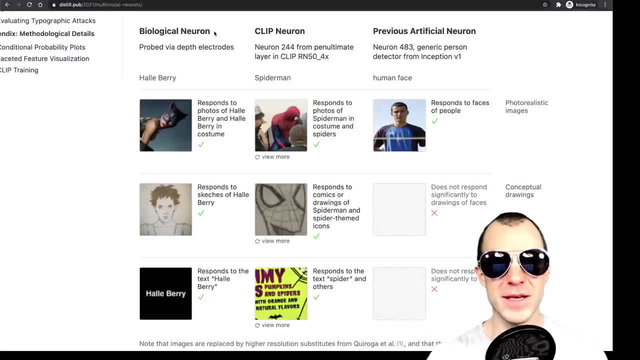 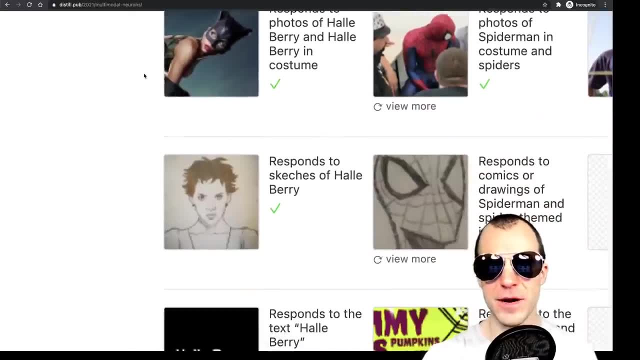 but to concepts. So there could be a concept neuron of Halle Berry, as you can see here, and that neuron would respond to photographs of Halle Berry, to drawings and sketches of Halle Berry and to the image of Halle Berry. So this is an investigation into the new CLIP model by 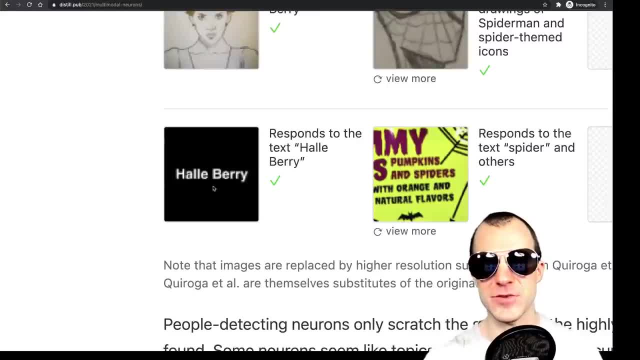 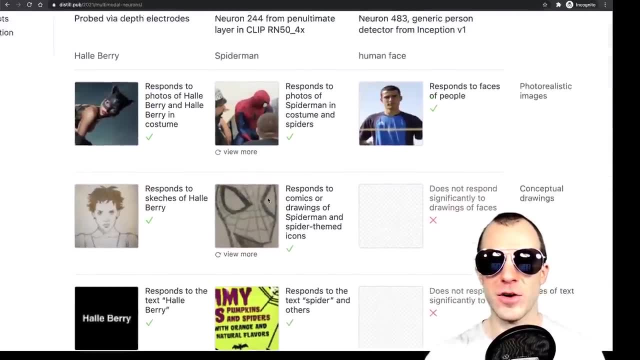 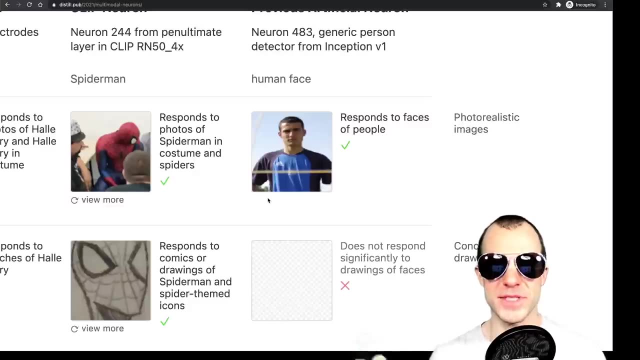 OpenAI And also to text. So if we see the text, the rasterized text, or we hear the word that neuron, that same neuron would fire. Now so far in artificial neural networks we have not seen this kind of multimodal perception. So we have seen neurons responding in general to the same class of images. 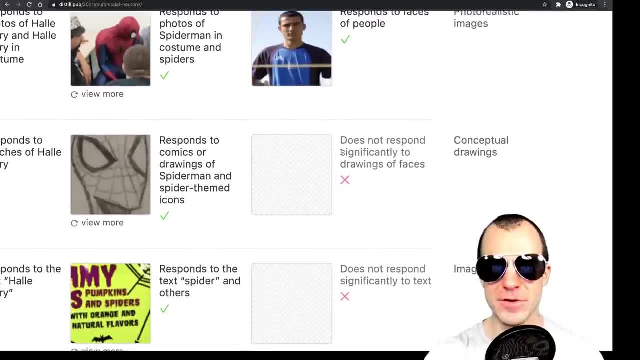 because we train them as image classifiers, But we have not seen that generalize to the environment. So we have seen neurons responding in general to the same class of images because we train them as image classifiers but we have not seen that generalize to the image classifiers. so we are. We have to imagine. 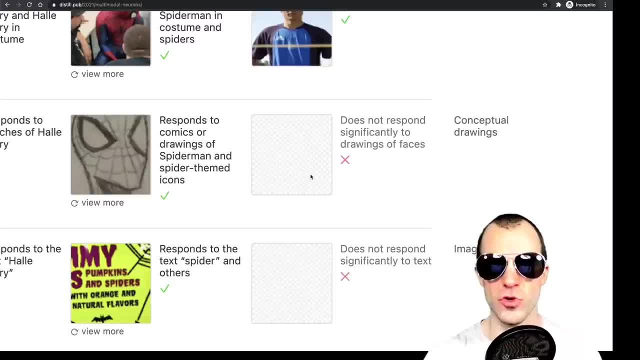 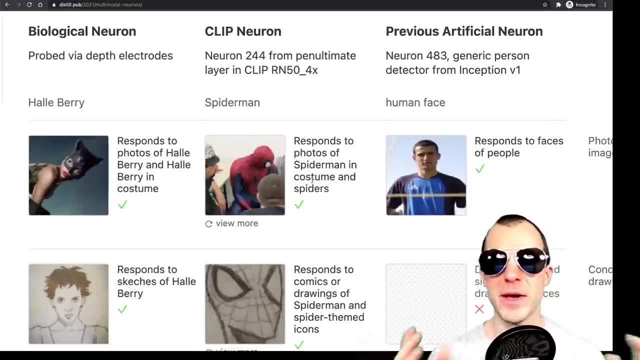 that this is an interesting question for us to figure out how we can do this. So if we look at your child's to other modalities, such as drawings or text, what they find in this clip model right here is that exactly what we expect in humans or, in general, in biological neural networks? 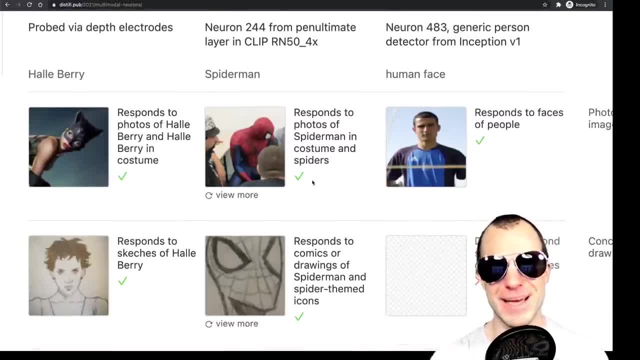 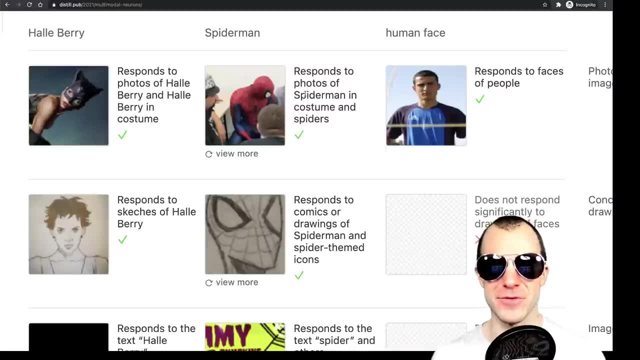 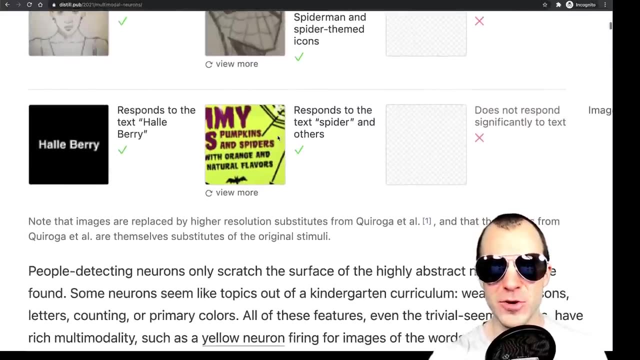 that happens. so they find, for example, a neuron that responds to spider-man, that is, you know, photos of spider-man in the real world or some person in a spider-man costume, drawings of spider-man and also text that says spider. so that would always the neuron would. 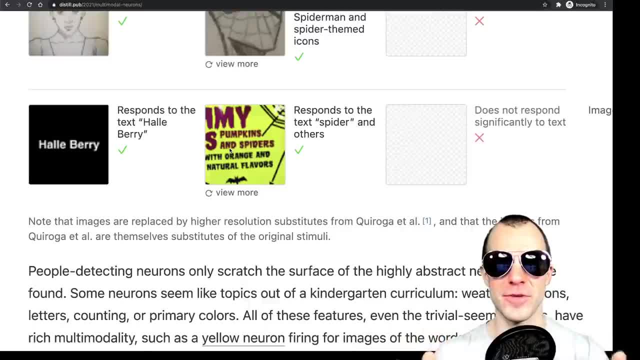 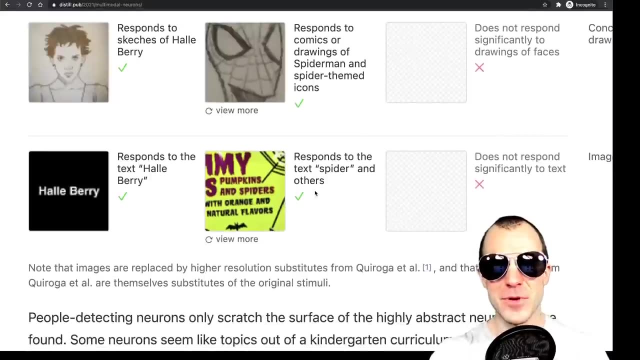 respond to all of these things the same neuron and that is a sort of sign that these models have learned to connect to different modalities together. we've already discussed in the clip video that the, the model sort of learns to do OCR, so it learns to recognize. 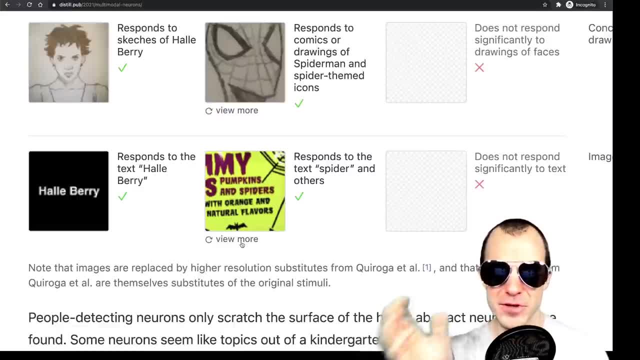 that there are different modalities that are connected to different modalities, because the clip model is fundamentally a model that connects images to text and my claim here is going to be that this addition of text, the model, I think, is very much a text model. so a lot. 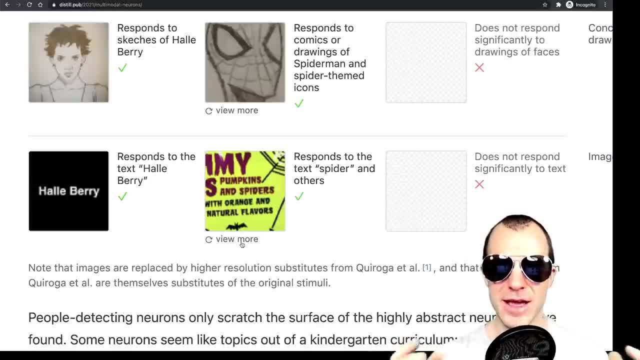 of the connection it makes go via the textual level and a lot of the responses you're going to see here. the visualizations are going to deal with text rather than with images, so here you can see what this neuron responds to. if you want to see what this neuron responds to, you can see. 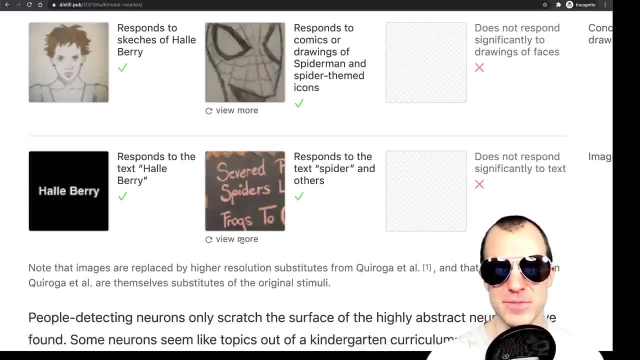 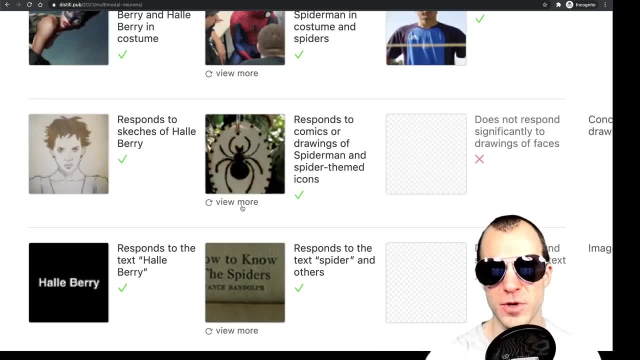 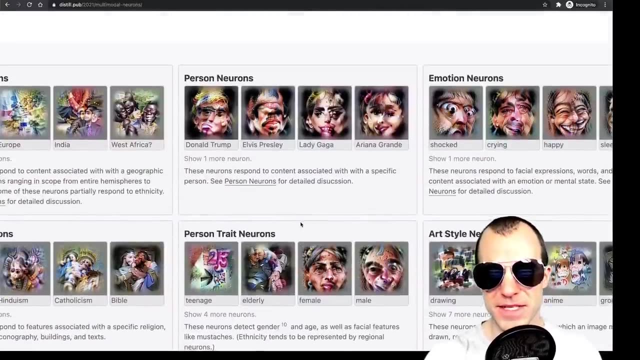 if you thought it was the spider web here. no, there's spider as a text, spider here, spider there, drawings of spider-man. so this neuron would respond to all of these things, which is pretty, pretty cool. so what they do, what they present here, is an overview over the different neurons they find. 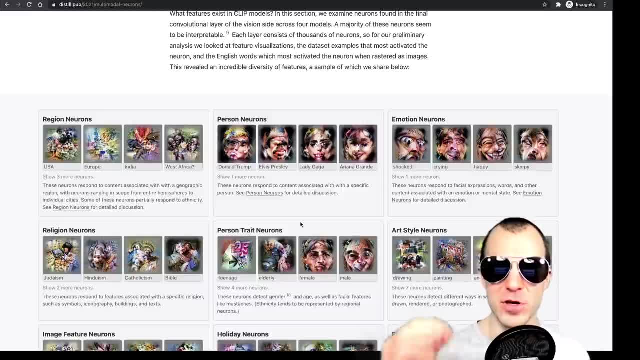 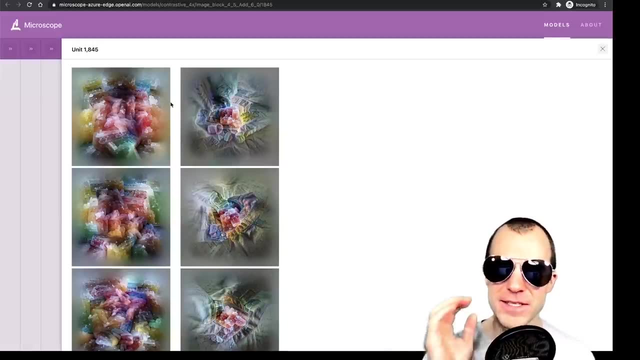 and, as I understand it, what they have done is they've gone through these neurons and they use their feature visualization technique with every single one of them. so I can show you what that looks like. here is the. this is the open AI microscope, and you can find that and this is the exact model they're looking at. so what you can do, 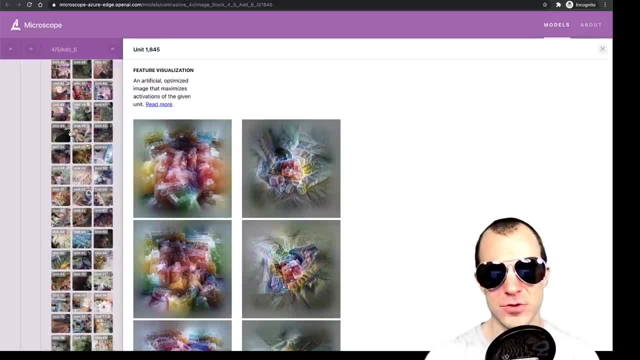 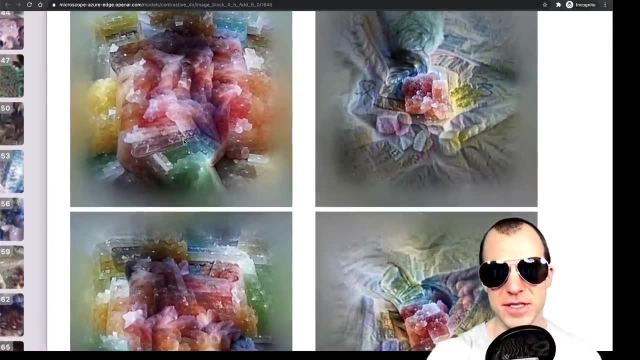 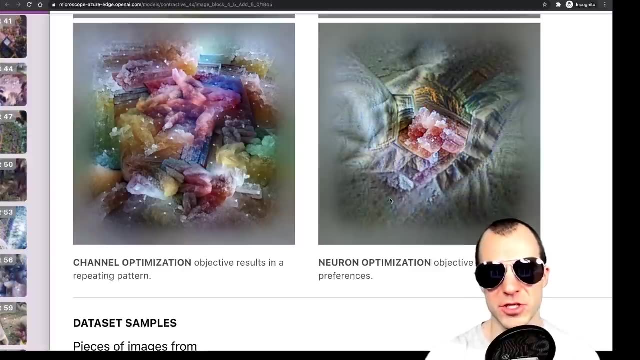 is. you can simply click around in these neurons over here and then these are the visualizations right here. so now the visualizations are twofold. so on the left hand you have channel optimization. on the right hand you have neuron optimization. we've treated them in a previous video if you want to know how they come about. but for now what? 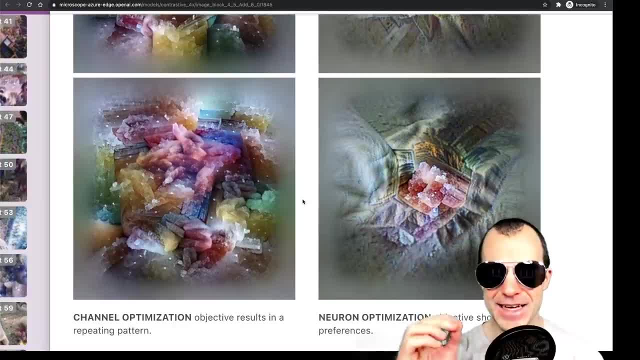 you should know is that these are images that activate that particular neuron or that particular channel. very much so they, these images, activate this particular thing in the neural network, but not other things. so this is a way to see what these neurons respond to heavily. so here you can see on. 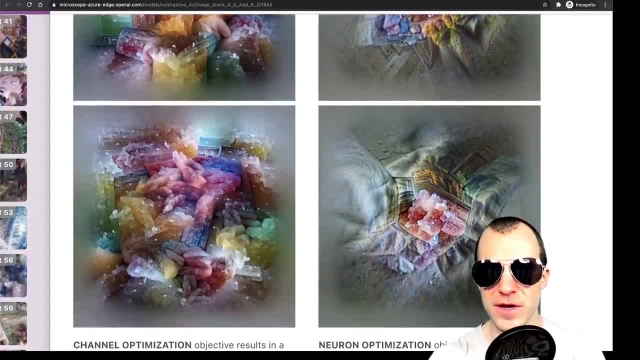 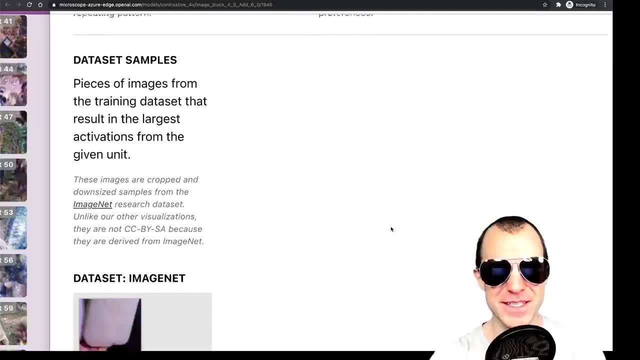 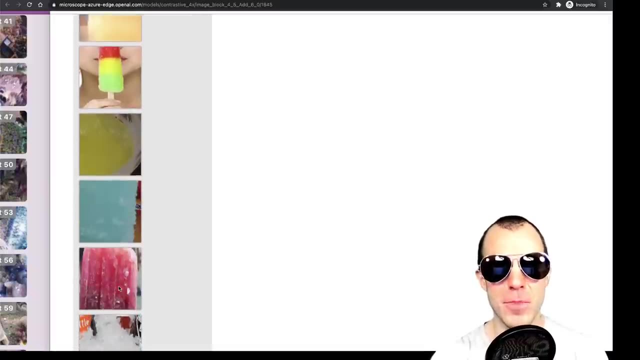 the right hand you often have kind of patternish structures. on the right do you more have kind of in the center, individual things? so maybe it's not really clear what this is. so what they also portray is data samples from the ImageNet data set that activate mostly that particular neuron. so you 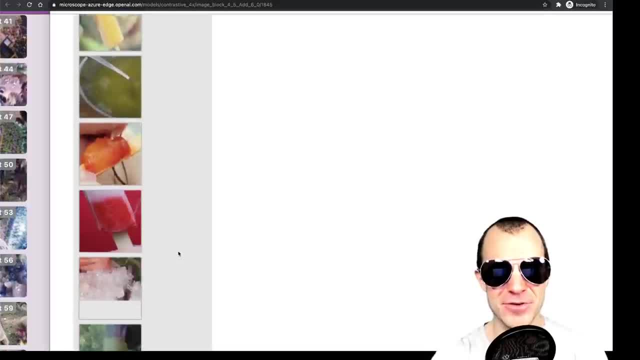 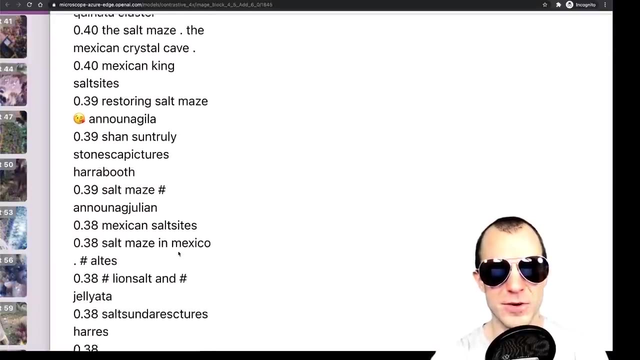 can pretty clearly see that this responds to popsicle ice cream. now they also have a different data set down. here there is a Flickr, creative Commons and very much the same. you see, this is kind of ice and ice cream and at the bottom you have text that goes along with it. so here it's not really ice cream. so this is a bit of a failure case. but 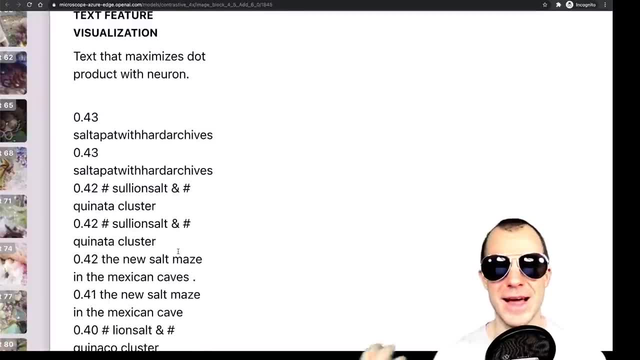 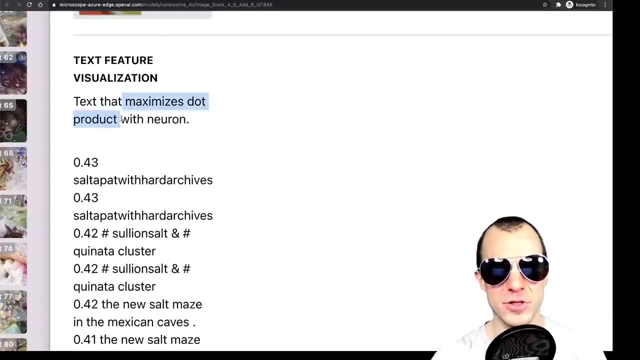 you always have to keep in mind that it could also be because of the lack in power in searching for text. so what they do down here is they have a search algorithm that finds pieces of text that that neuron responds to highly, so text that maximizes the dot product. so in the clip model you have an image part you have. 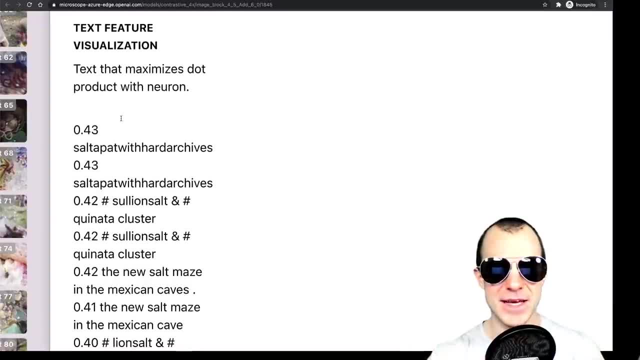 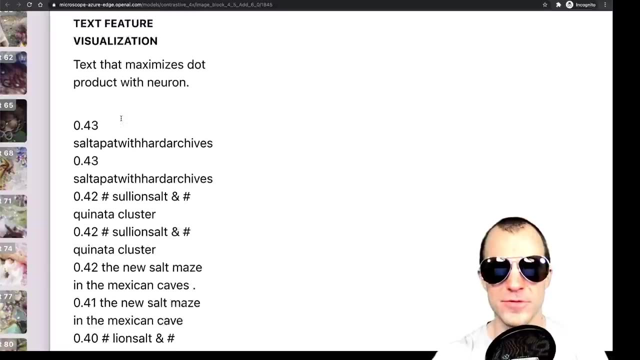 a text part and you have a dot product at the end. so this is text that, when you input it to the text part, maximizes the dot product with that particular neuron. so it's not always going to be, you know, really good text, but very often you can give you a hint in what the neuron thinks. note that this: 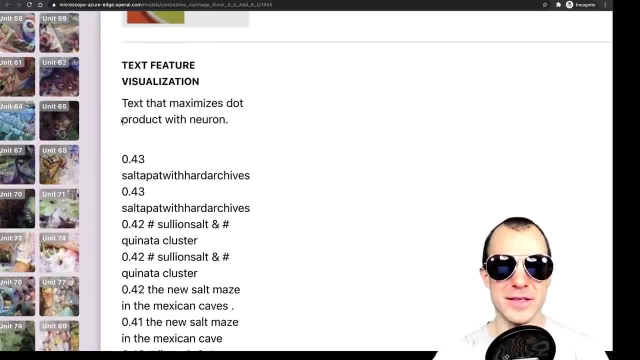 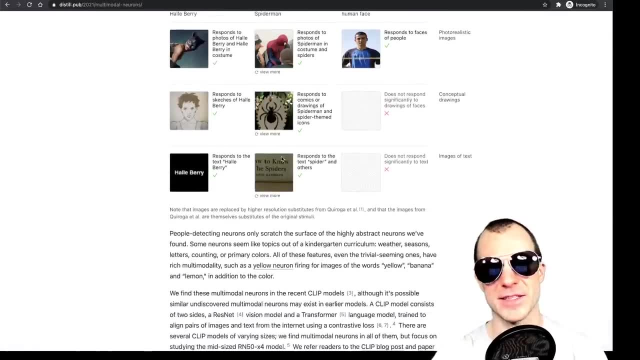 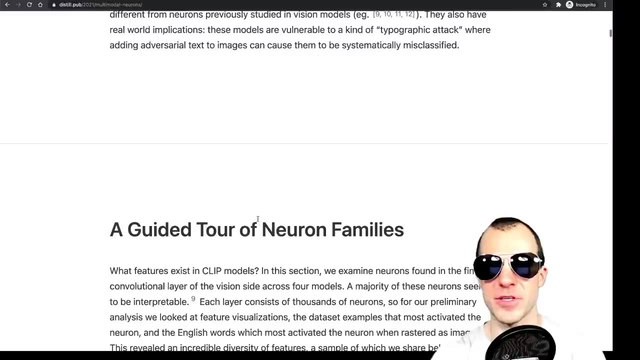 isn't the same text as we're going to see later, like the text that you saw in Spider-Man, because the text you saw in Spider-Man that was rendered text. so they do a lot of investigation into rendered text because the clip model is quite good at responding to rendered text in the image side. all right, so they find they. 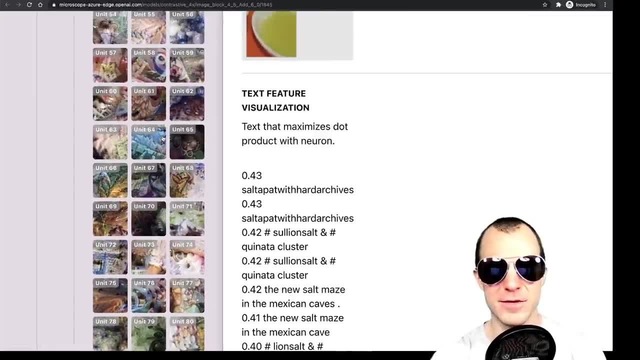 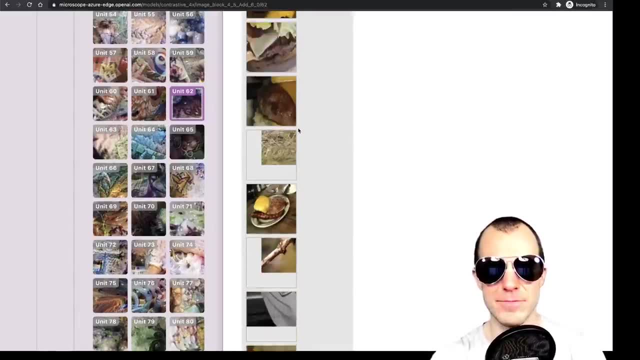 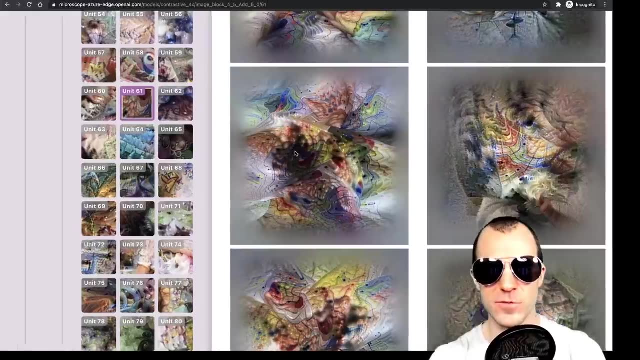 look at these neurons. literally I think they just click here on the left, boom, and you look at them. so this seems to be like a hamburger neuron and it is I. I. I did this for hours and I'll show you later what I found. this is absolutely. 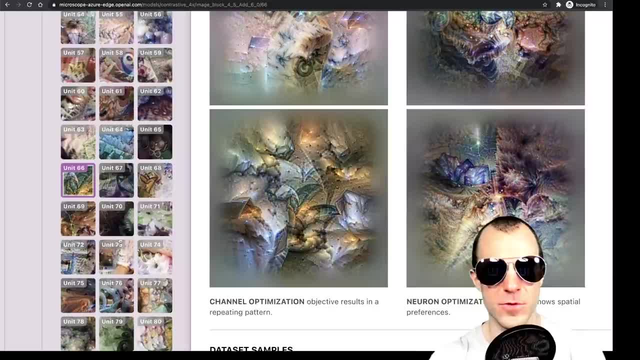 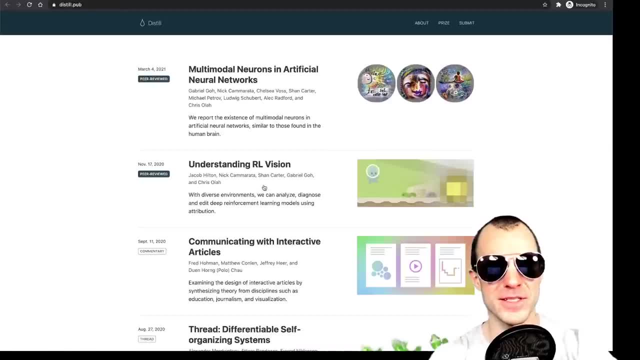 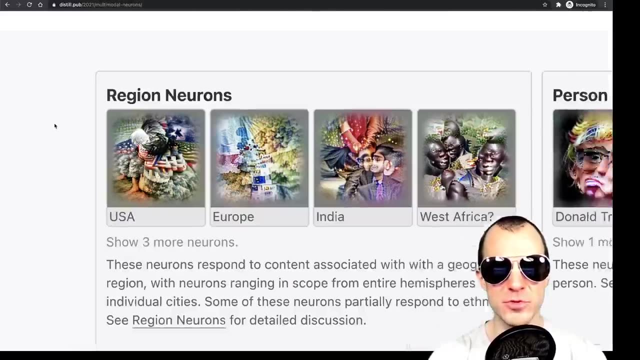 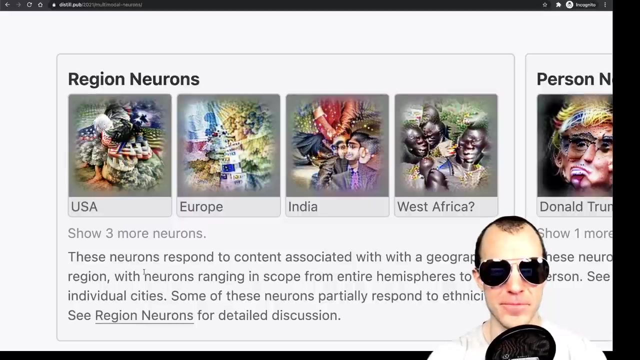 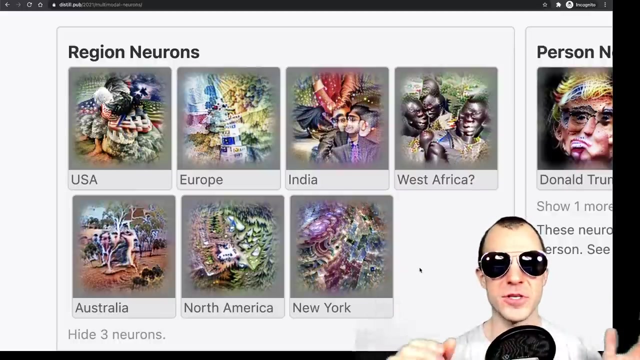 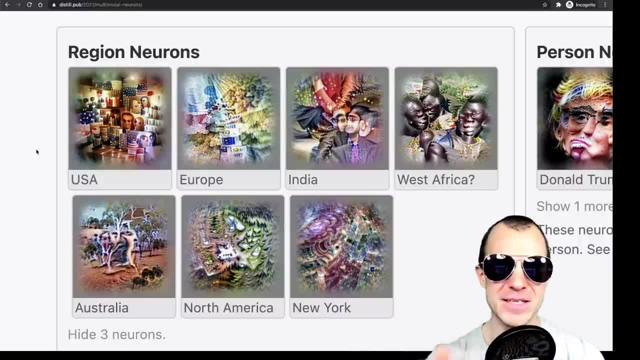 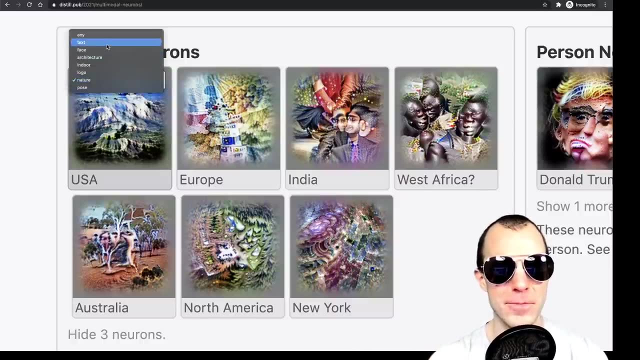 the same neuron. These are images that are made such that they represent indoor scenes, And there is an appendix. if you want to know how that's done, They can trim it to only produce nature pictures that this particular neuron responds to. So here you can get a much better insight. 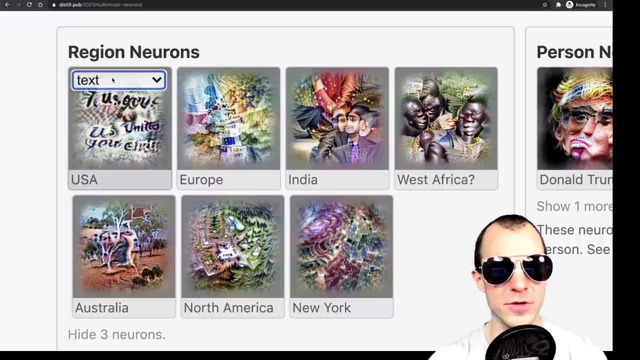 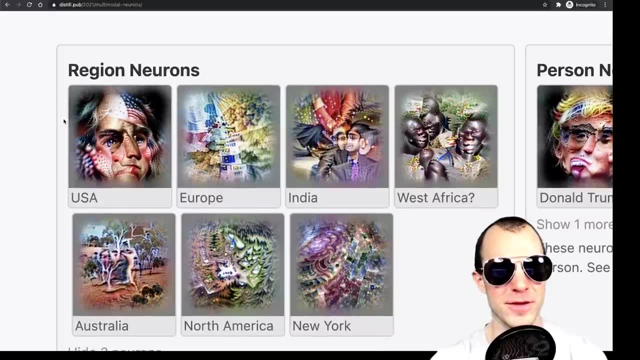 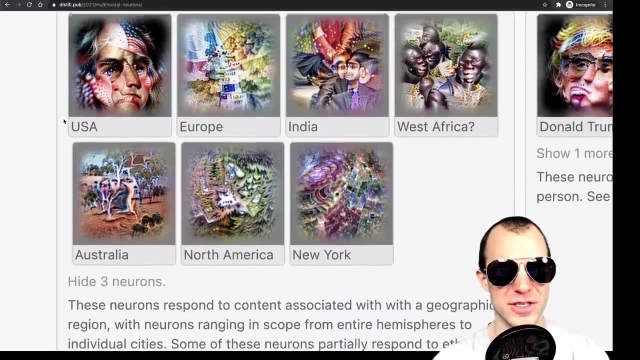 into what? into what the neuron looks at, For example, in if you create faces for the USA. this is, I don't know. I call this one. I call this one Benjamin Washington because it's a sort of a blend of Ben Franklin and George Washington, But in general it's pretty. 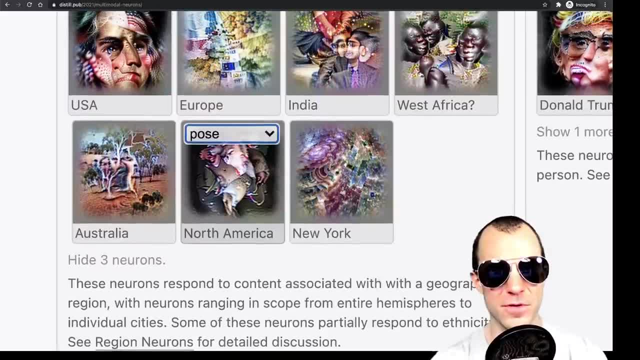 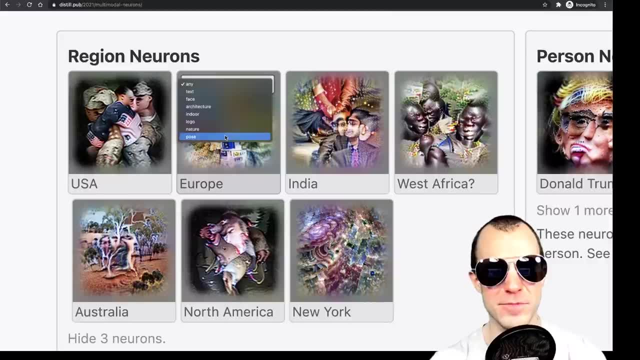 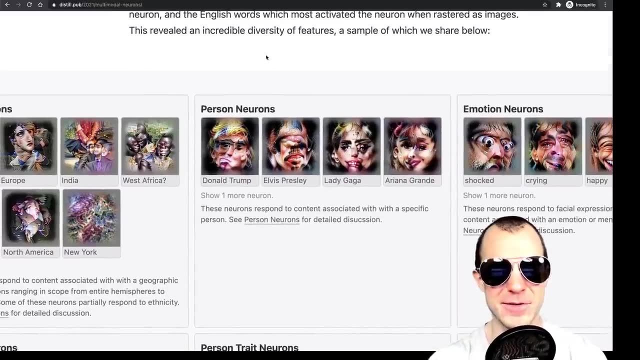 cool. So you can even- Yeah, nature you can do pose for North America, pose for the US. I think that's kind of a GI pose for Europe. I don't know what that is, But it doesn't always, you know, work out super well. But they find 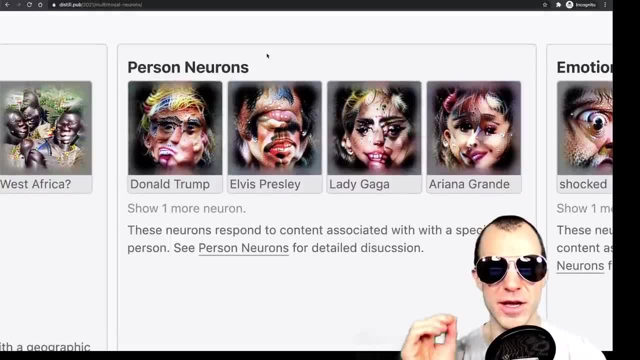 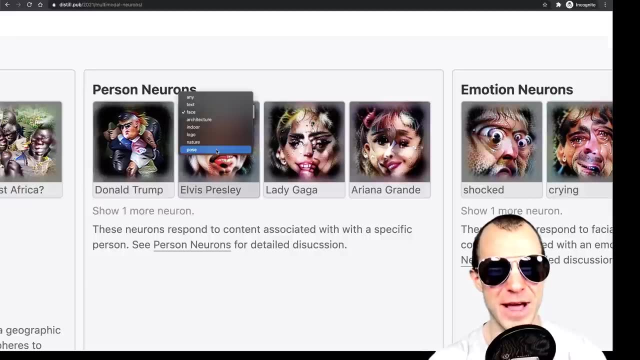 person neurons, So neurons that respond to individual people. be that faces, be that text. So this is Donald Trump, be that poses. Yeah, Elvis is also pretty cool. I've actually found- I don't know if I found the Elvis neuron myself or if I found a different one- 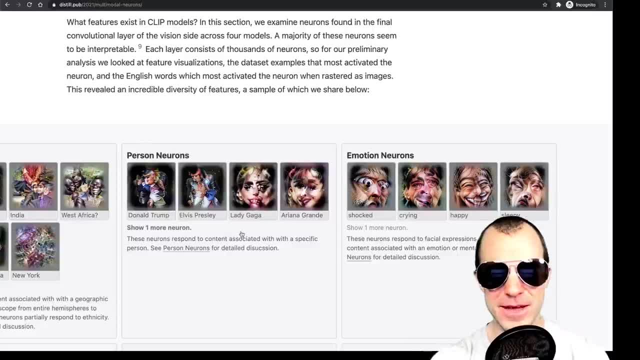 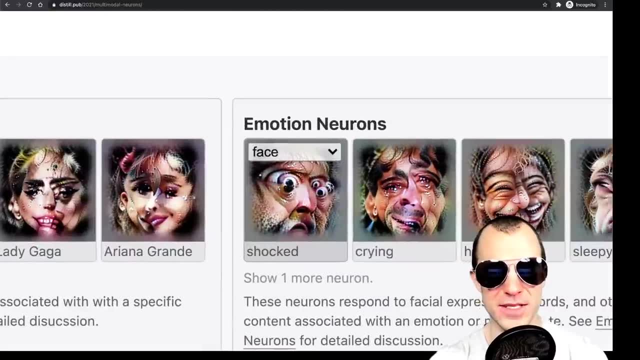 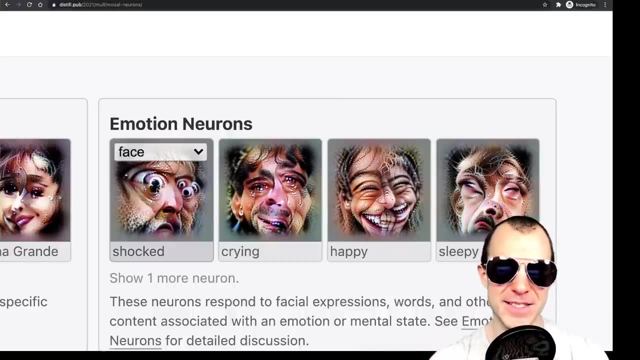 Um, yeah, so they also have emotion neurons, Which is also pretty cool, where they so they find neurons that respond to particular emotions. So when they tell these neurons, when they make a faceted reconstruction and tell, please give me a face, this is what comes out And that you know. it's just shocking. 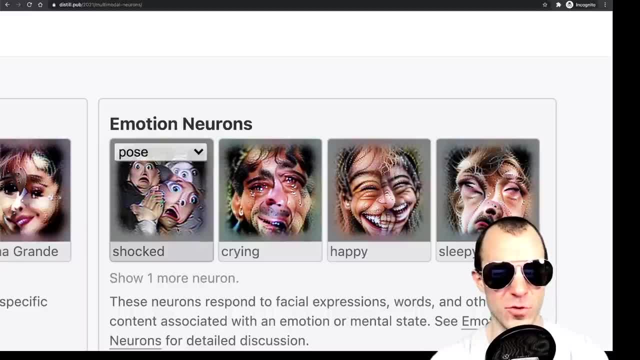 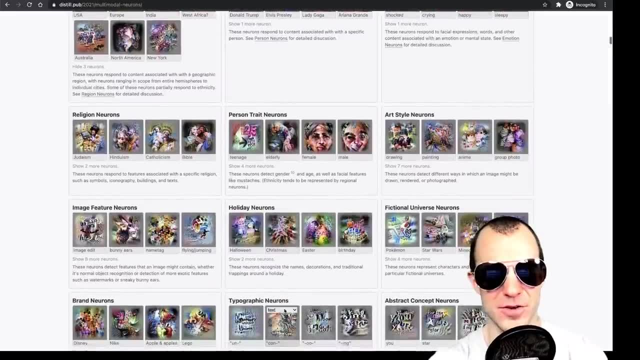 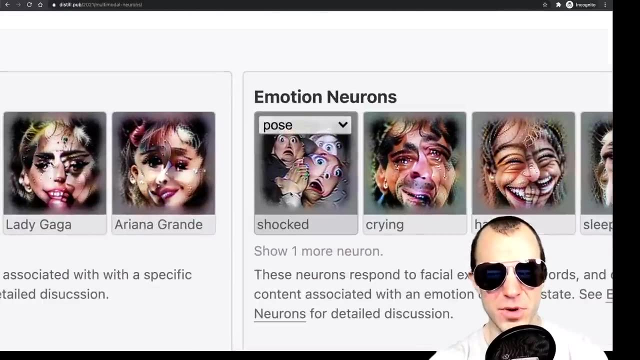 when you do something like a pose for shocked. this, I think we're only scratching the surface here. Um, honestly, but you can see the claim here. The claim is that the same neuron responds to this picture And to this picture. this is supposed to be text. you can only guide it. you can, you know, force it to this picture. 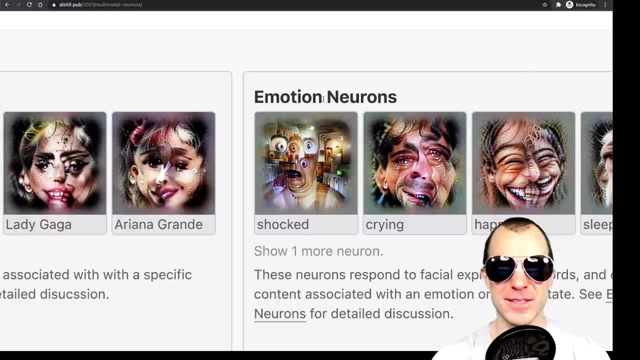 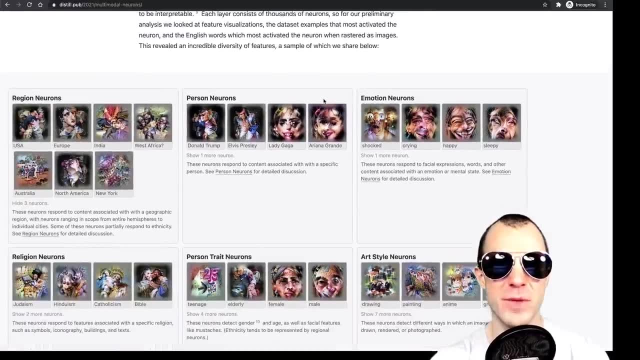 indoor to this picture. So the same neuron will respond to all of these And they call that multi modal neuron because it represents a concept, the concept of being shocked, rather than in a particular fine grained pattern, which was always the kind of problem so far with these neural networks, that the 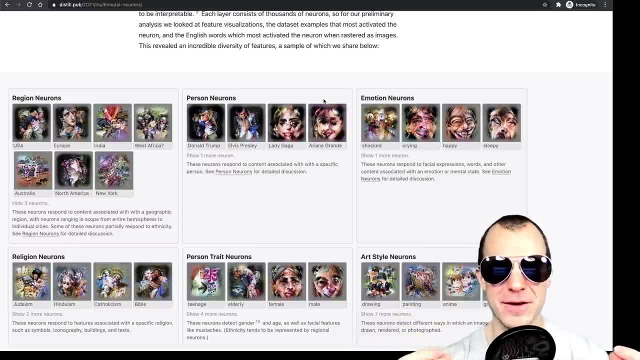 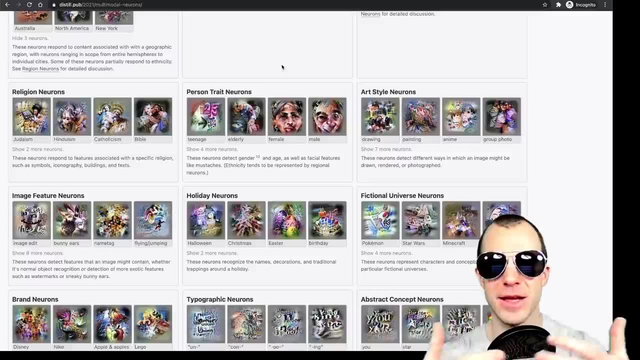 they were more looking at, you know, low level patterns than high level concepts. it seems, with clip, with, by combining modalities like images and text and by not forcing this constraint, like in a classifier, into 1000 predefined classes, we can gain much more. we can go up the hierarchy of features So they have art. 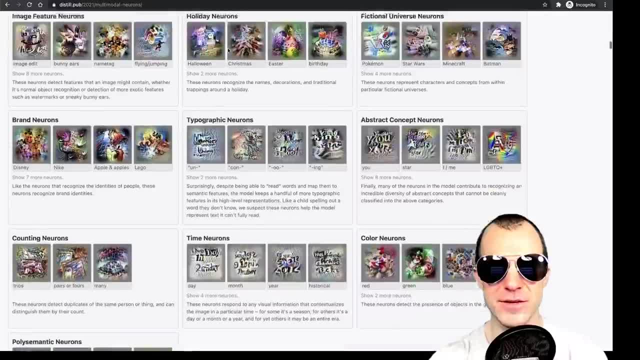 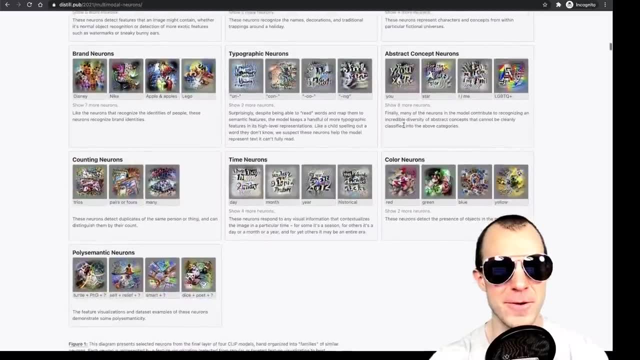 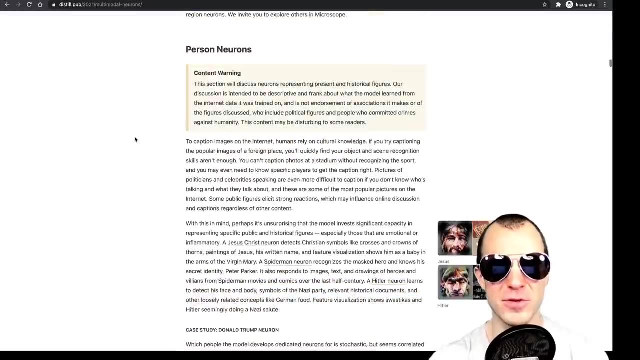 style. they have holiday neurons, religion neurons, person trait neurons, abstract concept neurons, the star- I found the star. I Yeah, I remember time neurons, counting neurons, pairs of force. they are not always so super good, but it clearly goes into the good direction. So here they highlight. 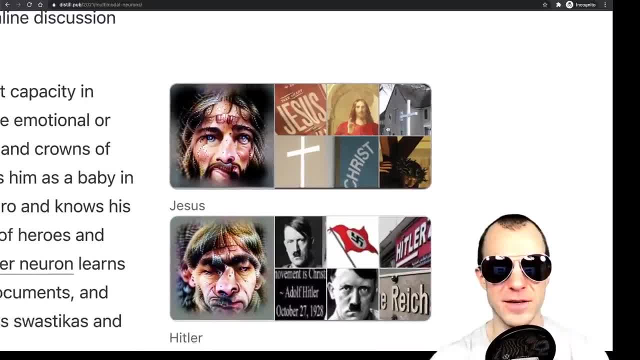 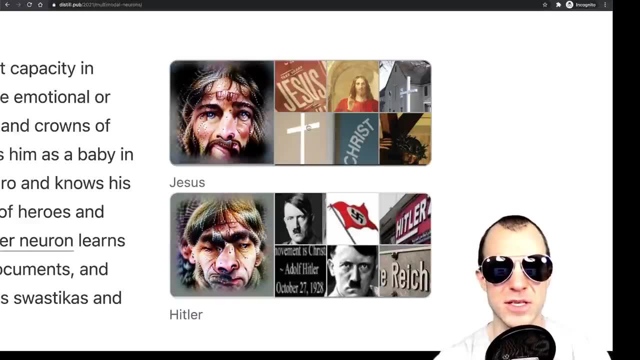 specific things. First, person neurons. So they find neurons that respond, for example, to Jesus Christ. So they would respond to all of these images here on the right you see their crosses, Jesus Christ and so on: depictions of Jesus, drawings of Jesus, And when you ask the model to generate you a image, that 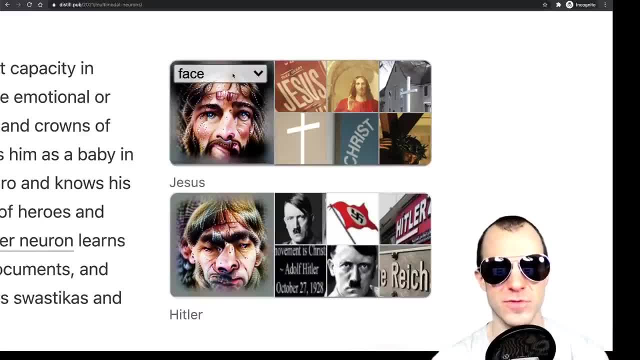 reconstructs this neurons activation and you can force it, or you guide it to make a face. This turns out to be a. and you can force it or you guide it to make a face. This turns out to be a. If you got it to make a pose. 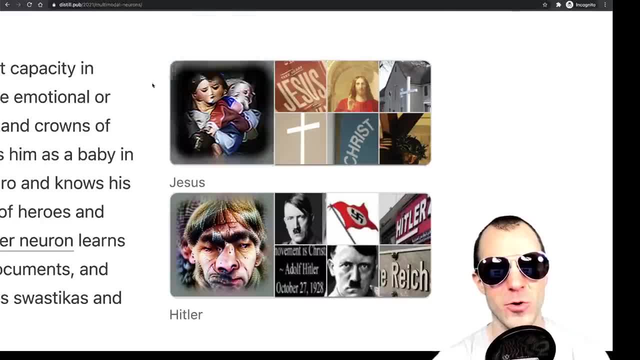 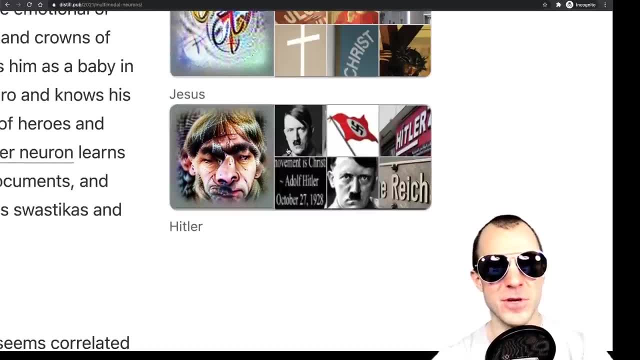 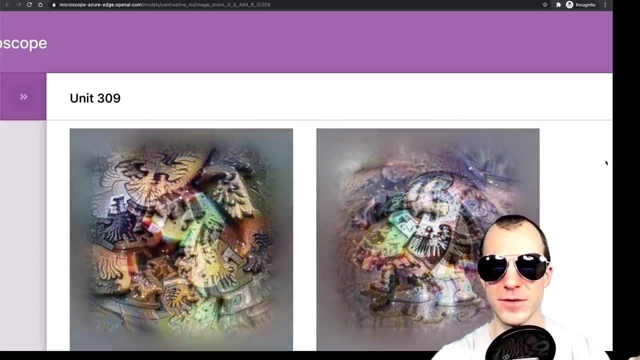 this turns out logo. obviously they also have Hitler right here, which is also pretty cool, though I have. If you click on these things, you'll get actually to the microscope thing And this is the one for for Hitler. And you know, I'm I'm not entirely sure that this is the case, like I can see. 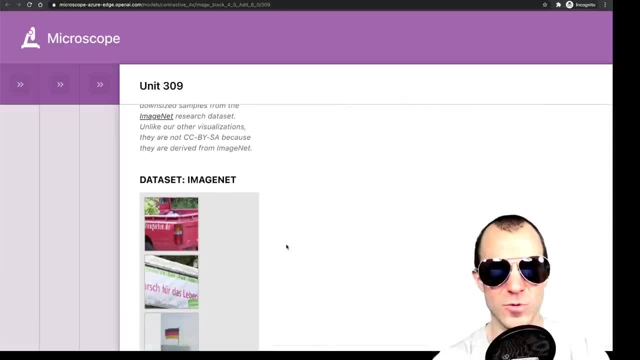 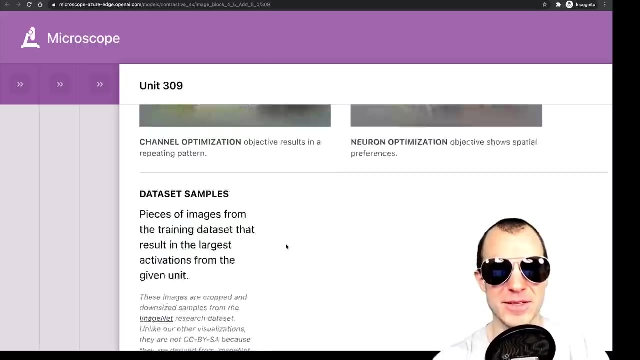 you know the kind of mustache stuff thing. but if you look at what in the data set activates this one, It's. it is a bunch of swastikas, but it is also just a bunch of kind of German political stuff. But yeah, I mean the concept, the concept here, even if it's not Hitler. 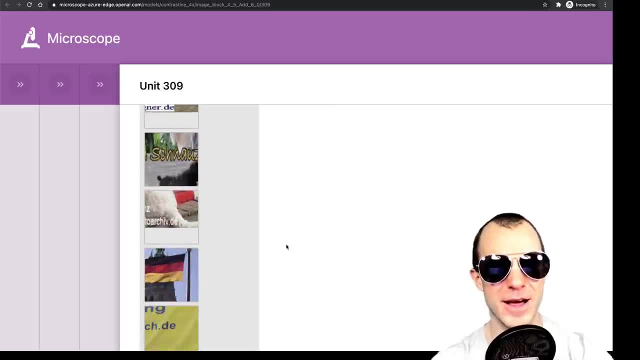 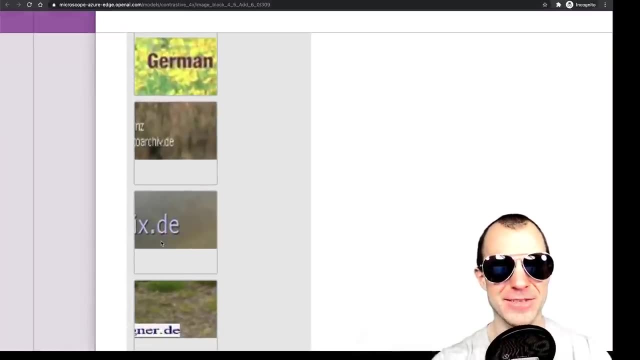 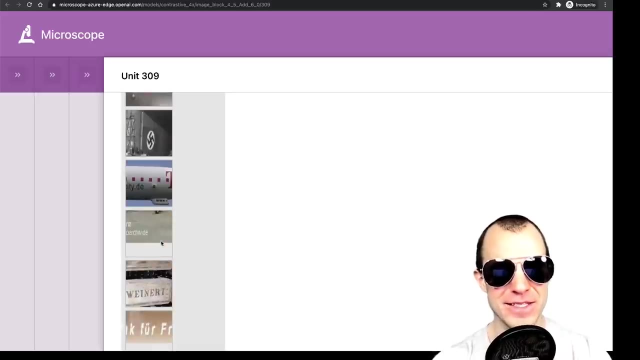 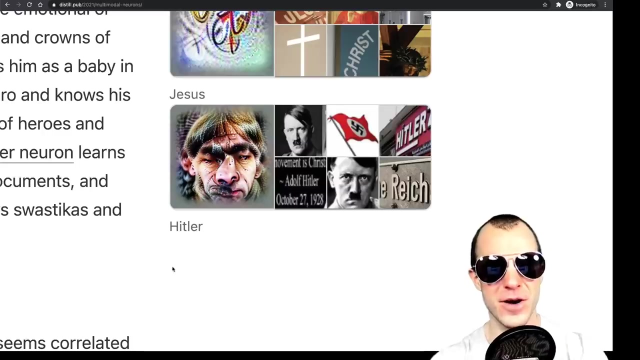 directly. it's pretty, pretty cool. I also found that domain endings rendered as images will activate the same neuron as the flag of that country and activate the same neuron as, like the architecture of that country. It is super duper interesting. All right, so they have these. 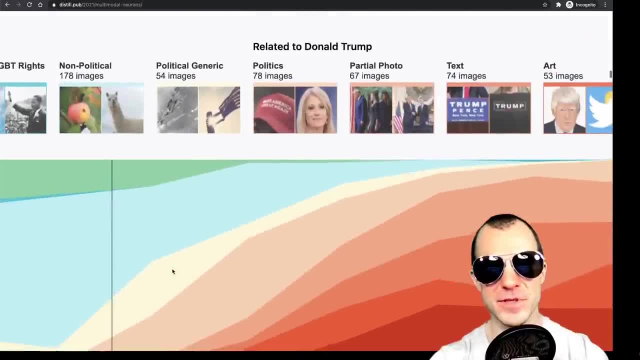 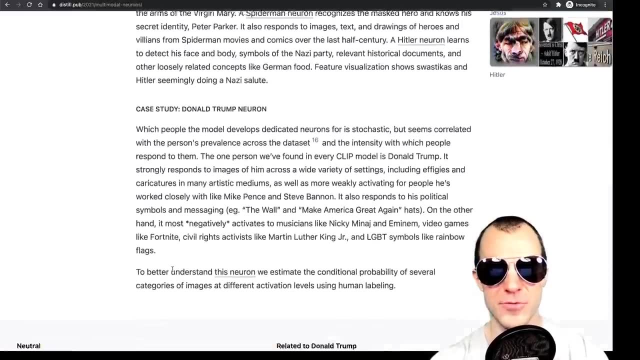 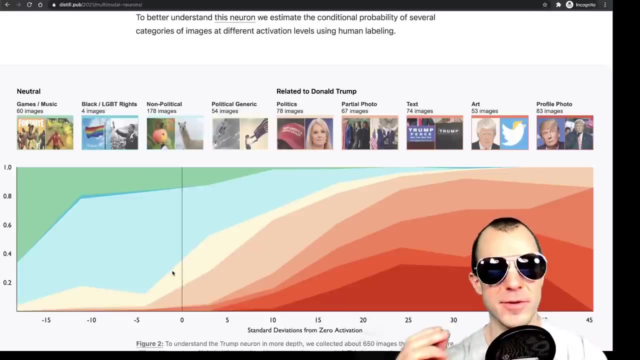 person neurons, which is already cool And they have. so they found these. they do a case study here for the Donald Trump neuron. So the Donald Trump neuron recognizes Donald Trump, and then they want to see what images in the data set activate this neuron by how much. so they make the claim here that if you, for example, 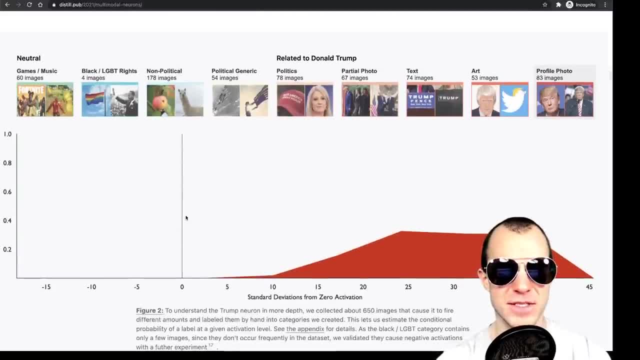 choose profile pictures of Donald Trump and you see here is the zero line And here is the standard deviations from zero activation. So pictures of Donald Trump activate this neuron like 30 times more than it is activated over the whole data set, which makes sense if that neuron 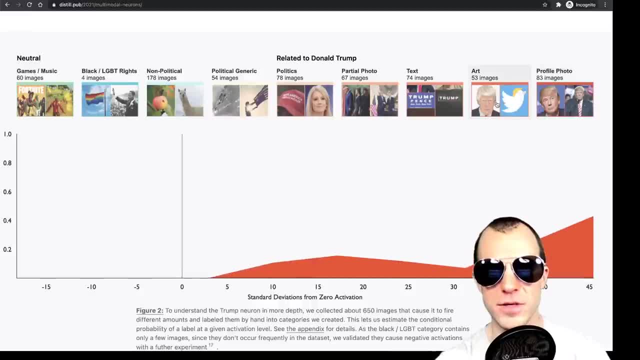 responds to Donald Trump, but it also responds to art images containing Donald Trump. By the way, these are all images of Donald Trump. So if you look at the data set, you can see that the these are classified by the authors here. they've gone through the images and they've classified. 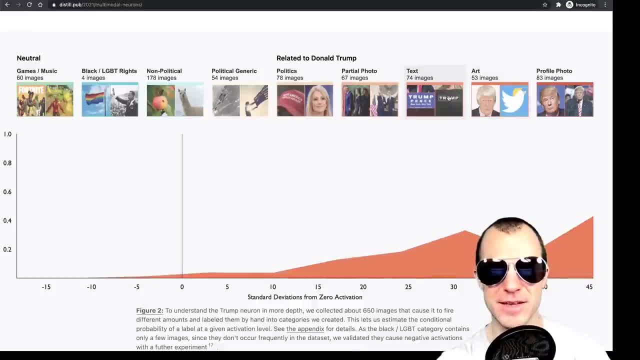 them into these categories. Text containing Donald Trump's name, the model also strongly responds with the same neuron, right? That's the. that's the crazy part. So a picture with text in it that says Trump activates the same neuron as a profile picture of Trump activates the same neuron. as a profile picture of Donald Trump. So that's the crazy part. So a picture with text in it that says Donald Trump activates the same neuron as a profile picture of Donald Trump. So that's the crazy part. So a picture with text in it that says: 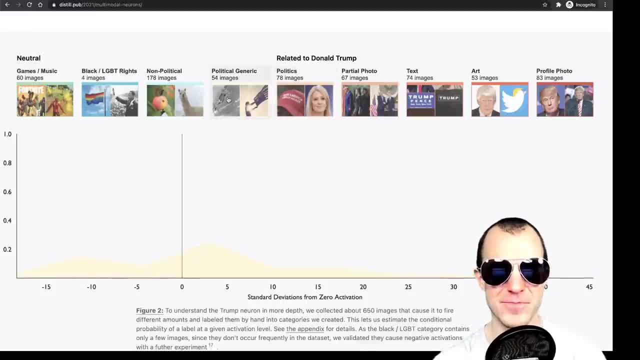 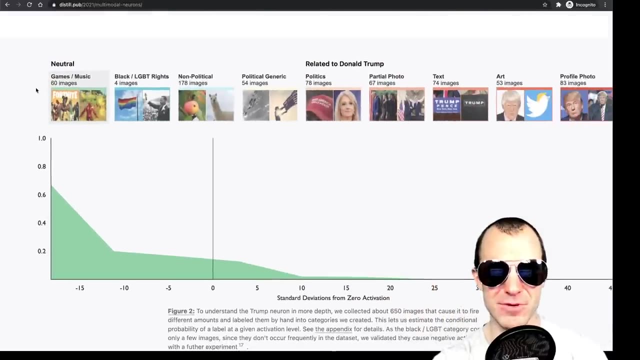 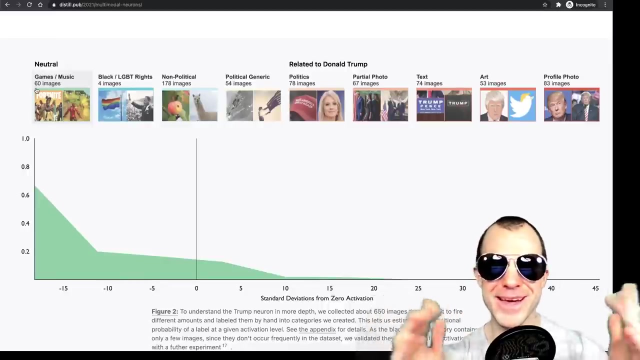 a Maga hat and activates sometimes the same neuron as political images and activates So the. if you look at games and music and so on, that is very, that neuron is very deactivated. So not only is it zero, it's actually negative, which the authors interpreted as sort of being being counter to. 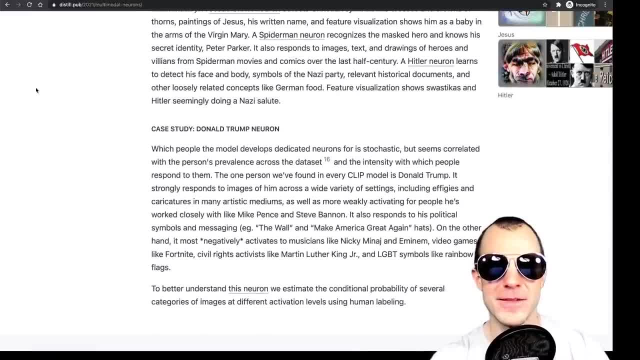 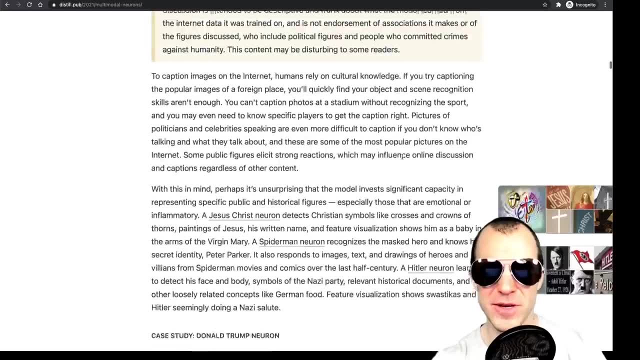 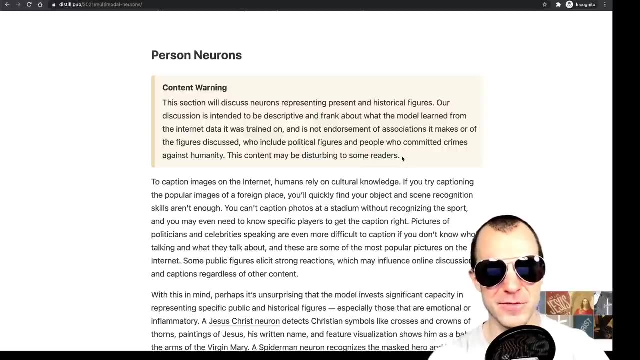 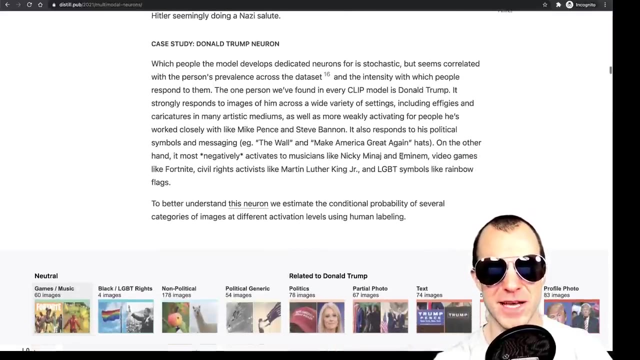 that in the space of all concepts They do. so This paper is is full of this kind of content, warnings it might be disturbing and so on, which you know you can, you can do. but I also find I also find the rest of the paper is kind of a fairly large hedge against certain things and it gets political at times, for example when they want to, when they want to claim that. 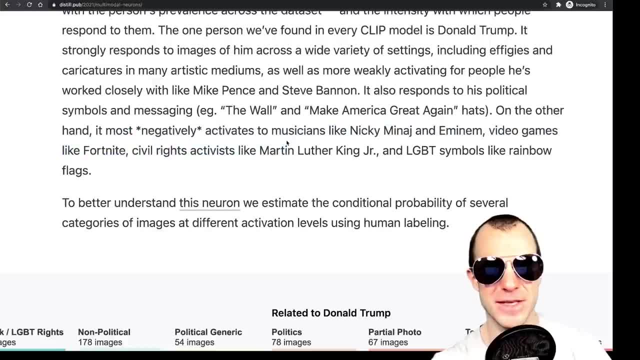 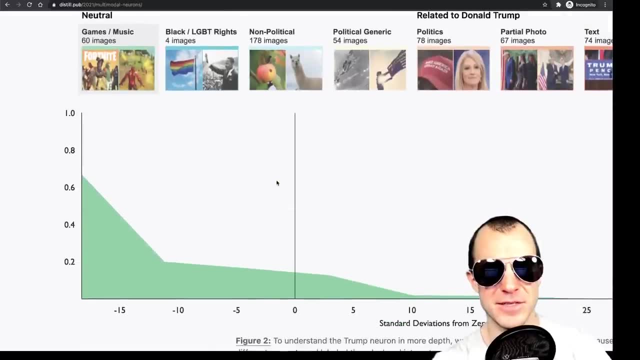 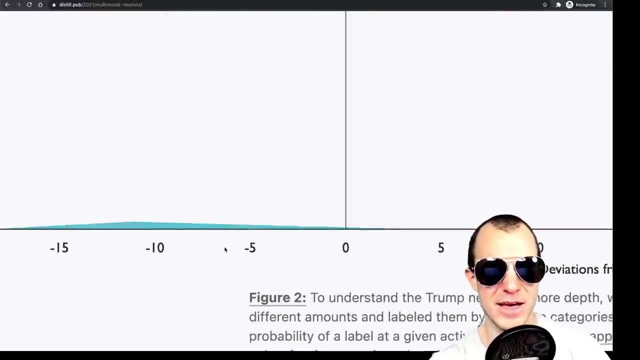 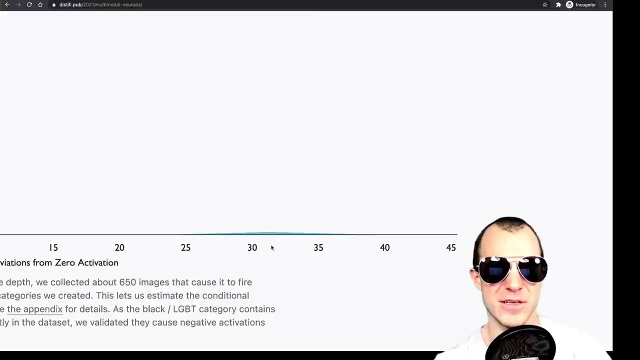 So here, on the other hand, it most negatively activates to musicians like Nicki Minaj and Eminem, video games like Fortnite, civil rights activists like Martin Luther King Jr and LGBT symbols like rainbow flags. So the games and the Fortnite here, yes, we can see that. But if you click on this- and they have four images of this- you can see that it's activated at relatively low magnet, like negative magnitudes, which is correct. but then it is also almost equally activated over here at high magnitudes, So like 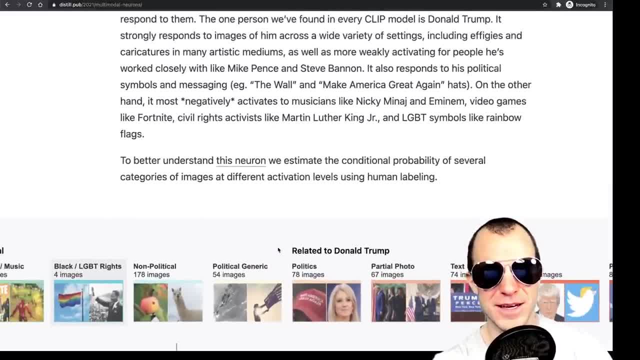 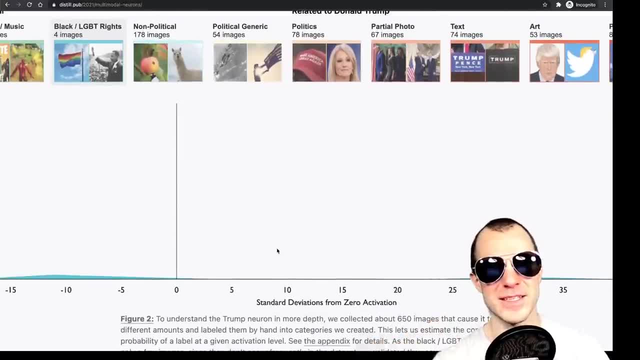 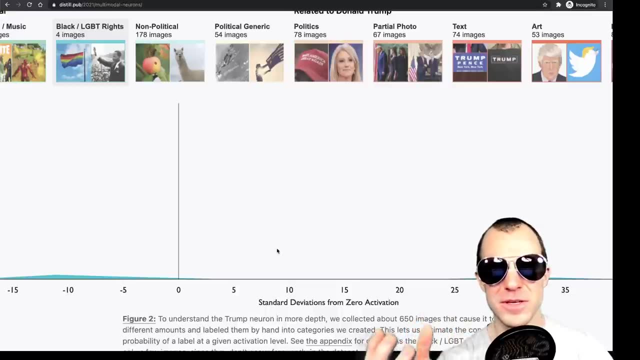 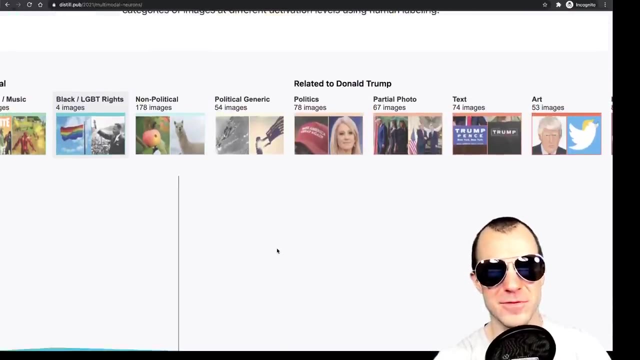 I see the point you're trying to make, But I mean if, if you are in the political sphere, this is not, you have to, you have to not interpret this as meaning that these things are kind of aligned, but you have to interpret it as these things will appear together often, which you know one can. one can definitely understand in this case. 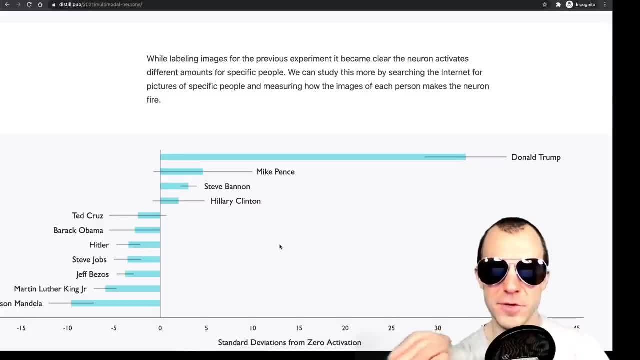 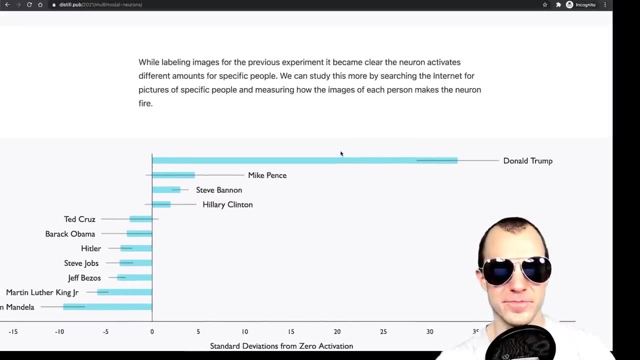 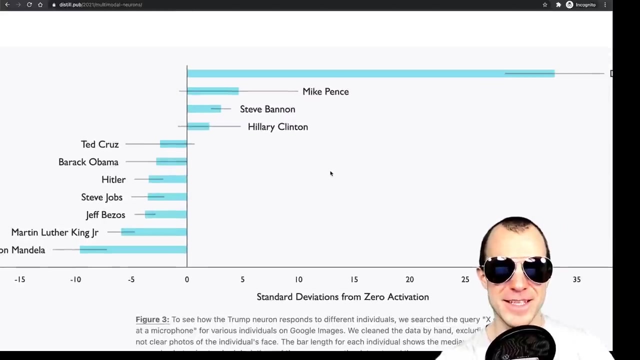 So here they search for profile pictures of other people, including Donald Trump himself, And they plot how much these profile pictures of other people activate the Trump neuron And you can see that, for example, well, yeah, Pence activates this neuron by quite a bit, I think. yeah, the selection here is, you know, up to the authors of course, but it's, it's fairly interesting to see that. 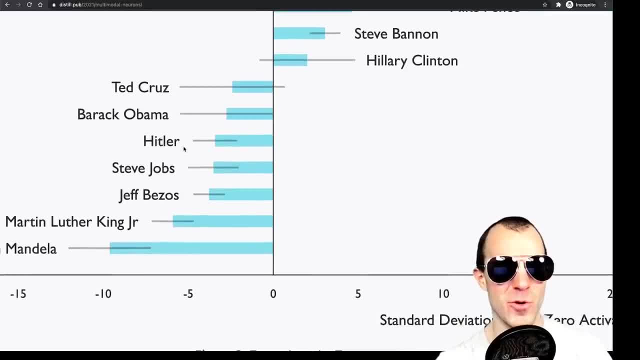 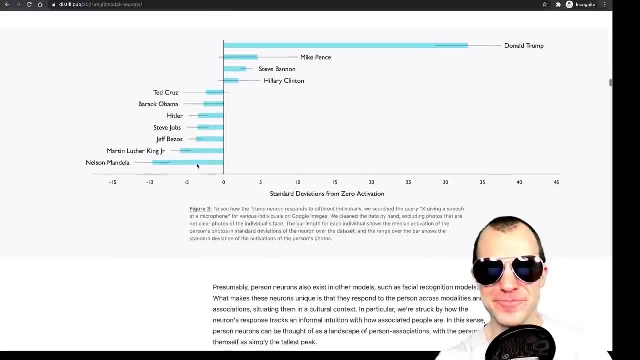 Clinton, Cruz and Obama activated more than Hitler And almost as much as Steve Jobs, for some reason. So I'm not I'm not entirely sure what you can make of this, But it's definitely interesting to in on this side, like to observe the multimodality of pictures, just the fact that text drawings symbols of that campaign and you can see that they kind of activate the Trump neuron. I mean, that's part of it. 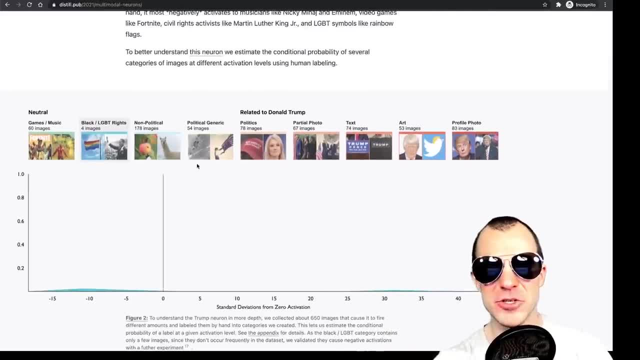 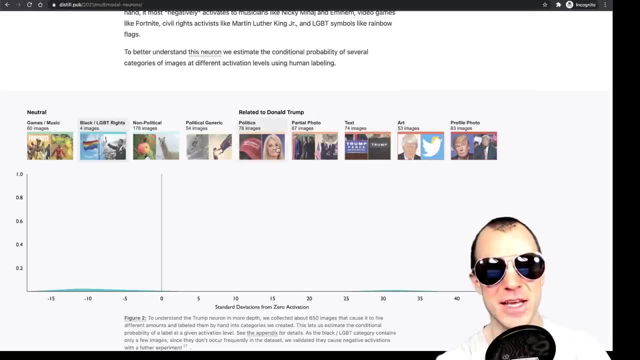 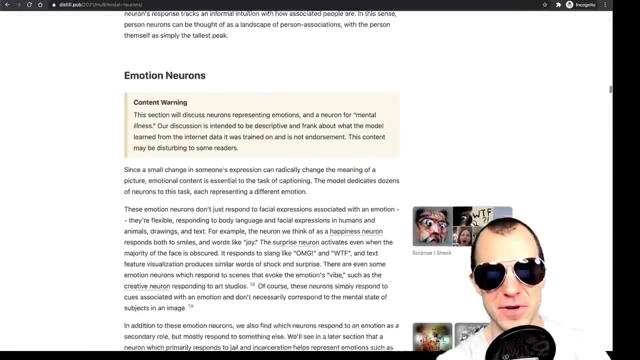 you can make of this, But it's definitely interesting to in on this side, like to observe the multimodality of pictures. just the fact that text, drawings, symbols of that campaign and profile pictures will all activate the same neuron. that is fairly impressive. They go on. 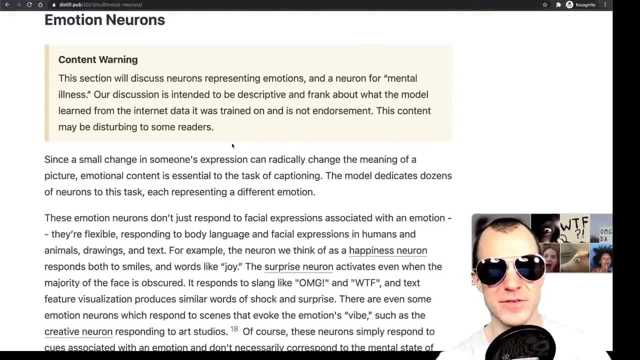 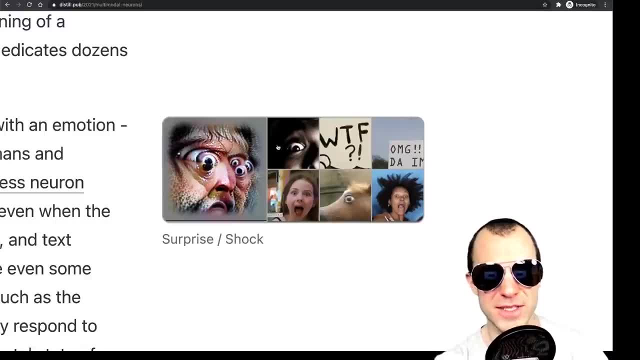 and they identify emotion neurons. So again, there's a content warning, by the way, also here. So here they identify a neuron that responds to surprise or shock, And you can see that all of these pictures on the right will activate that neuron. So there are faces being shocked there. 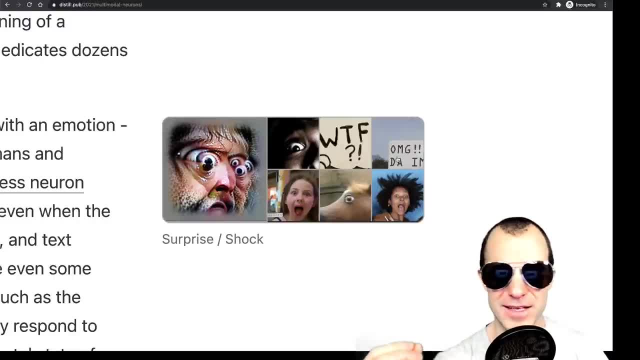 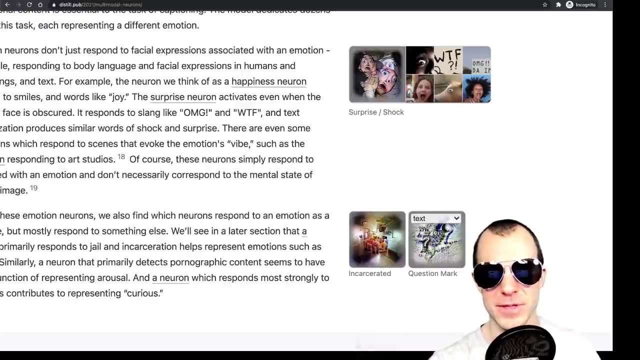 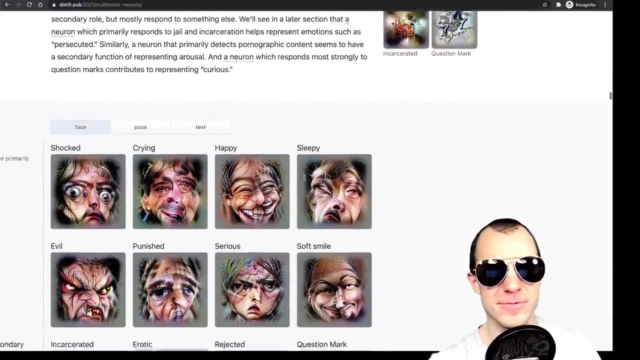 are horses being shocked And there is rendered text saying like WTF, OMG, and so on Again. if you, I think we've, we've gone through this- this is the shocked one. There are also secondary neurons that help, Let's say, help the primary emotion neurons. So here you can see an overview over the different 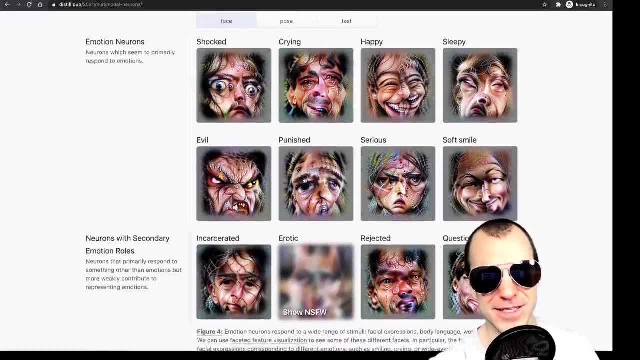 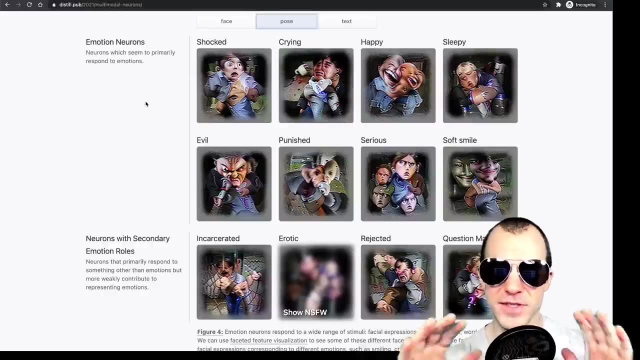 emotion neurons they have found And it is pretty stunning. So here they asked them obviously to create a face. when they constrain them- not constrain, they guide them towards making poses. By the way, the way you guide them is they train linear probe classifiers on separate data sets. So 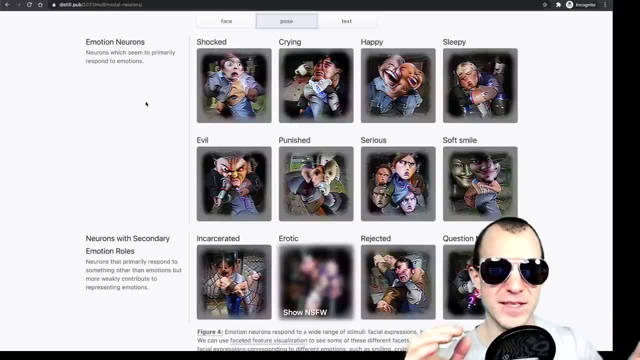 they would train a classifier on a face, data set to distinguish all faces from all non faces, And then that use that classifier to sort of guide this reconstruction process. That's how you can sort of choose to end up with a face or with a pose, or with a piece of text. So, as you can see it's. 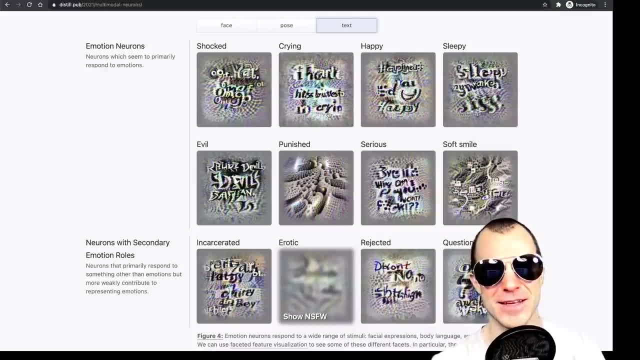 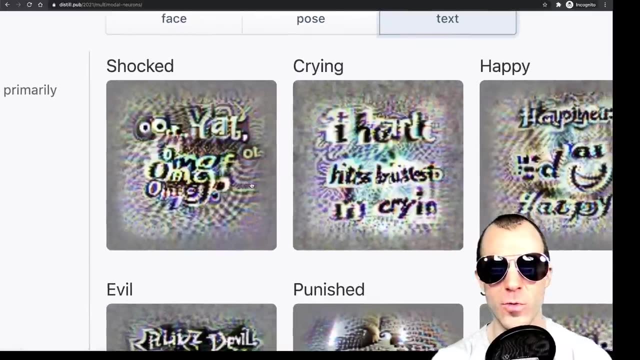 pretty, pretty cool that even the text that comes out of this reconstruction process, these aren't real images, right, These are kind of reconstructed to activate those neurons, Like for evil. you can see that there's devil and Satan. For shocked, it's like OMG. For crap. for happy, it's, it's happy. 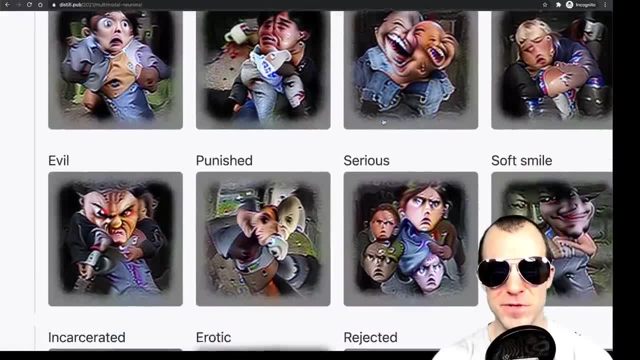 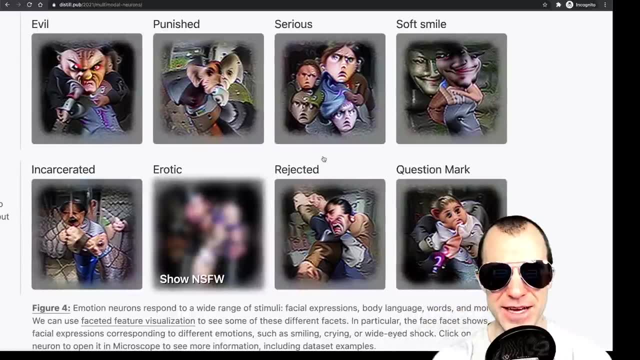 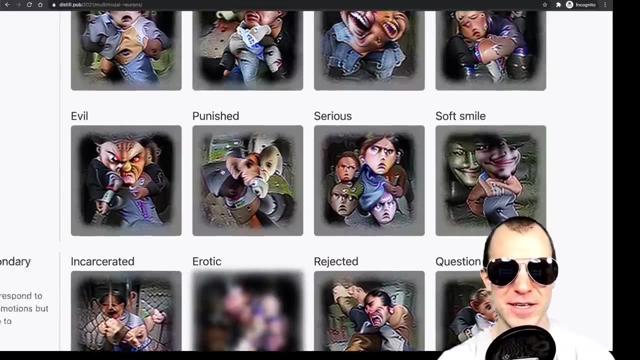 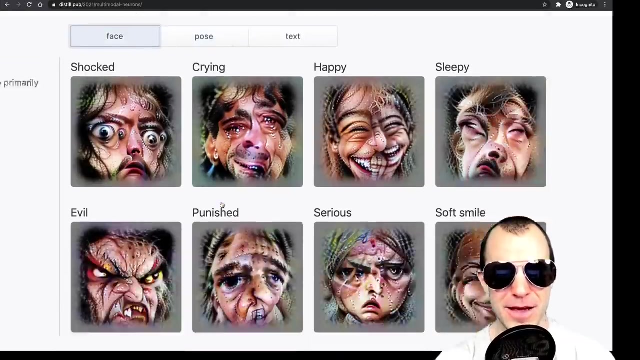 If you look at the poses for happy, for serious evil is particularly cool. incarcerated, rejected- This is. I think this is absolutely cool. There is the NSFW, there is erotic, there are erotic neurons And if I click on this, it will show. now, If you click on this, absolutely nothing. not safe for work will. 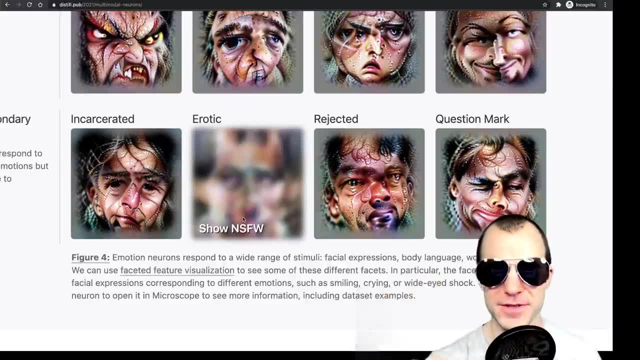 happen. I promise I don't promise, but you know I I've tried it, It's fine. I will not click on it Because if this model things that's not safe for work, The YouTube algorithm will think it's not safe for work. So but what I can tell you is that if you go on that neuron and you go click through it to go to the microscope and you look at what image net pictures respond to that neuron heavily, you'll find out that image net isn't the really clean dog breed data set that you might have known. 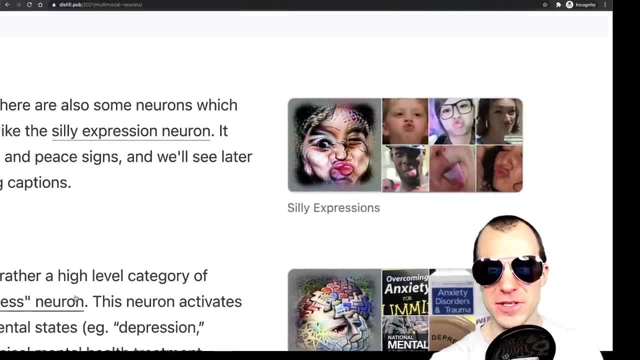 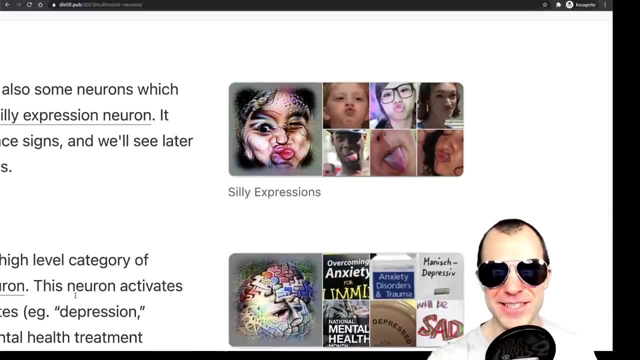 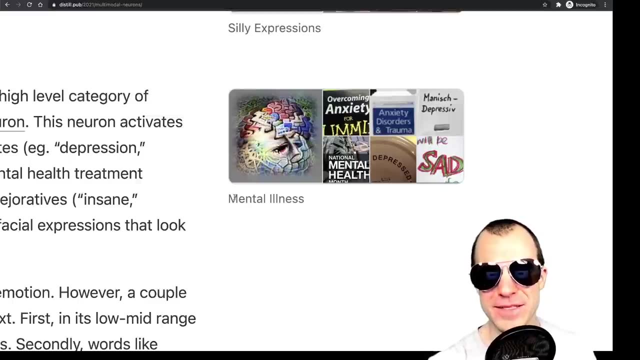 All right. They found other neurons Corresponding to silly facial expressions like duck faces and tongue showing and so on, which is it's pretty neat. And they find this neuron that corresponds to mental illness, which the reconstruction is just amazing like this is just mind baffling. 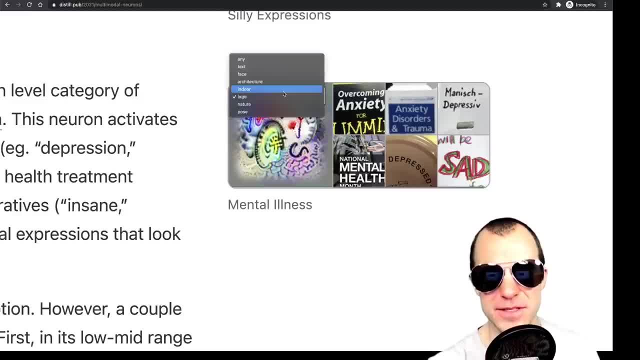 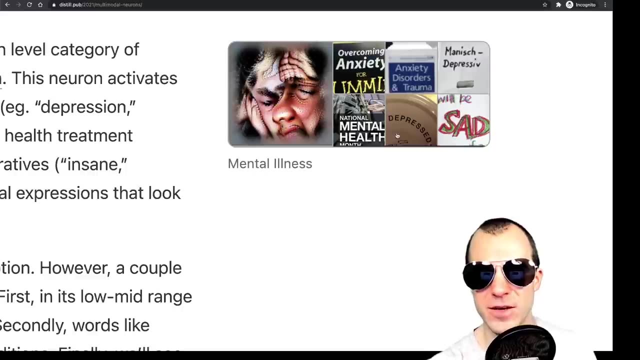 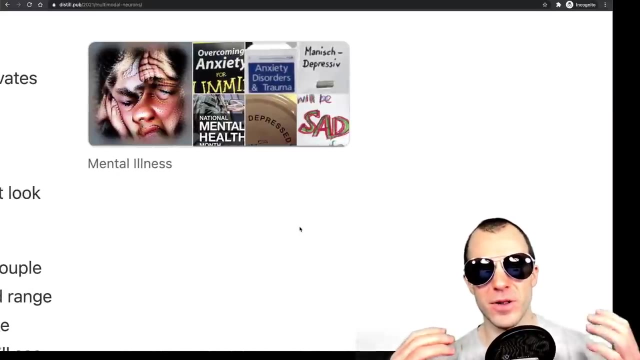 Nature kind of always looks the same. But mental illness, let's say face, This is, this is. it's crazy How this model connects things, and it connects these things to books and writings of sad mental health, anxiety and so on. Now do I think the model understands what a mental illness is? No, I don't think so. I think, much like in GPT-3, it is learned to statistically associate things, So it is learned that there might be 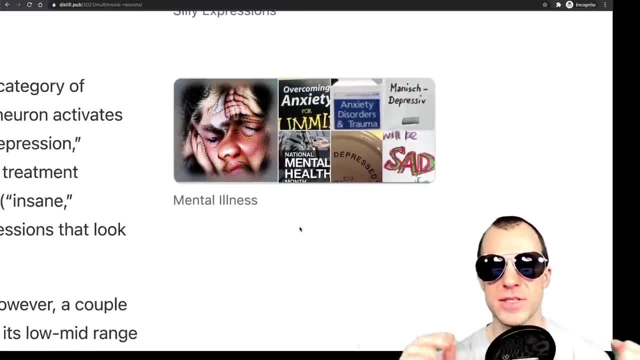 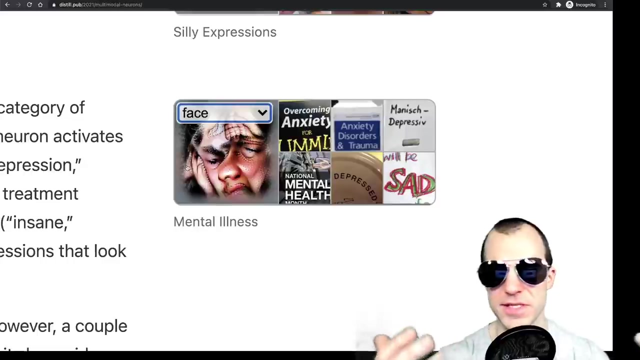 a mental illness, to speak That. I think that happens via the textual input. So in clip, for every image you have a piece of text And I think the connection between the topics happens on the textual level because the text descriptions are the same between images. So they're the images of people you know cowering like this, being sad, and the textual description for it would be something like mental illness, anxiety, sadness, and then for these, 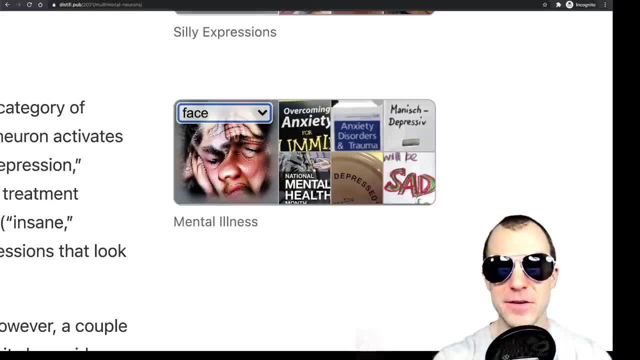 images And then for these mental illness, anxiety, sadness, And so it doesn't quite match And it's not as much of a difference in terms of the way you can document the images. Yeah, I suppose So you're. you're still trying to do that, right? 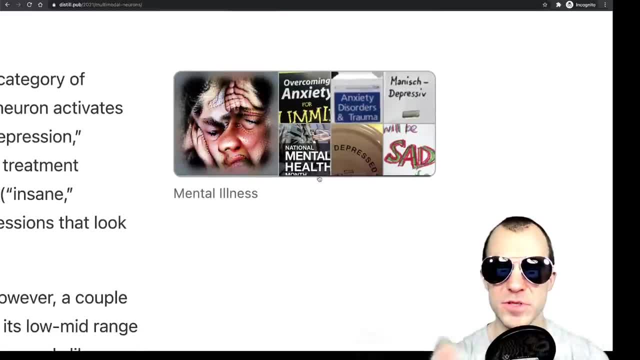 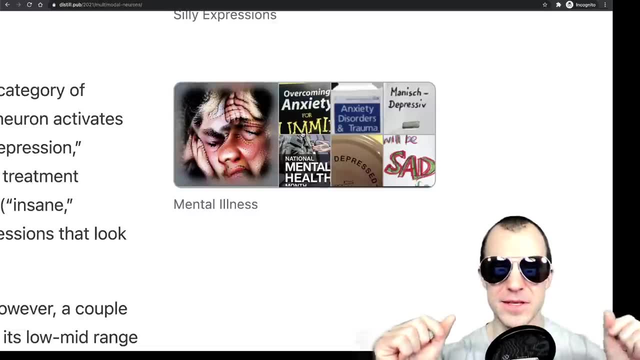 Yeah, Yeah, Yeah, I'm still trying to do that. pictures of these books as well. there the descriptions would be. I mean, this is one is literally called overcoming anxiety. So if the picture is of a book and the description says: 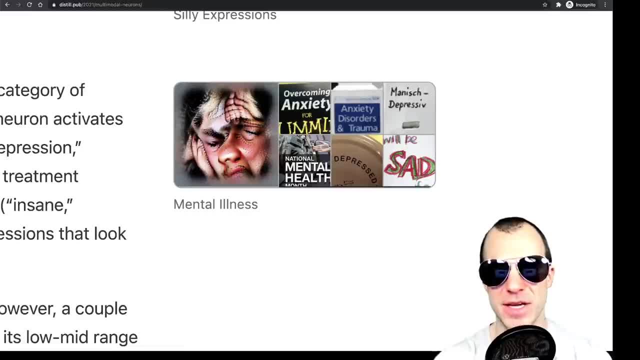 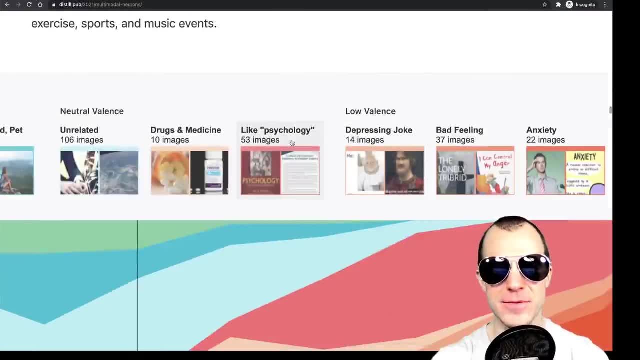 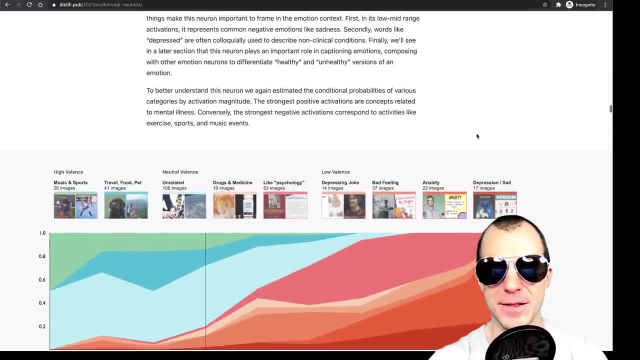 what is on the picture. obviously, that text will be connected, So I think that's how it learns to connect things via the text, And I think this thing is in large part a text model. So here they do the same study for images that are associated with mental illness, So depression. 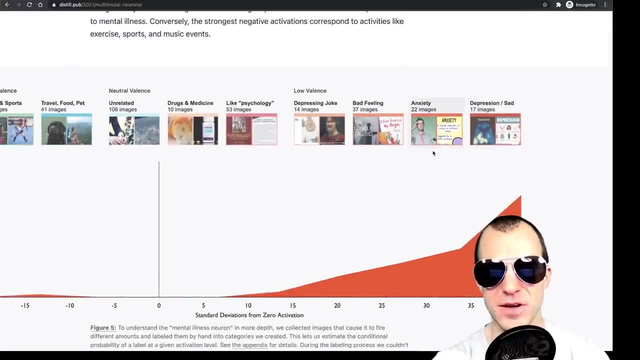 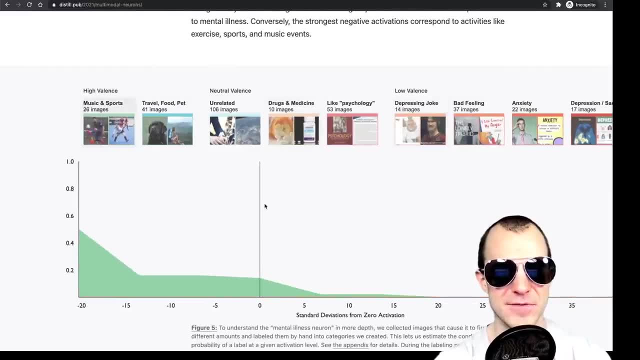 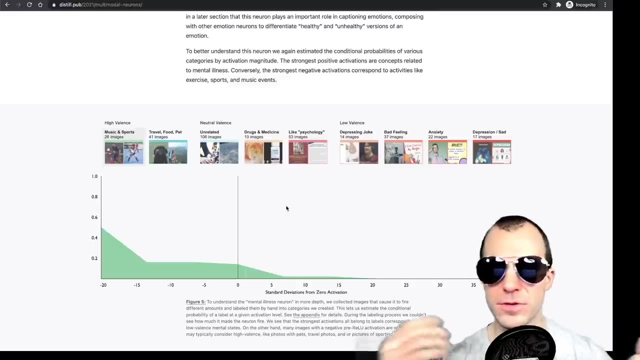 sad pictures like anxiety pictures are pretty high. Depressing jokes- if you look at music and sports that's negatively activated and so on. So you can see that I think via the text the model can sort of learn about how different, different concepts, different things, different- 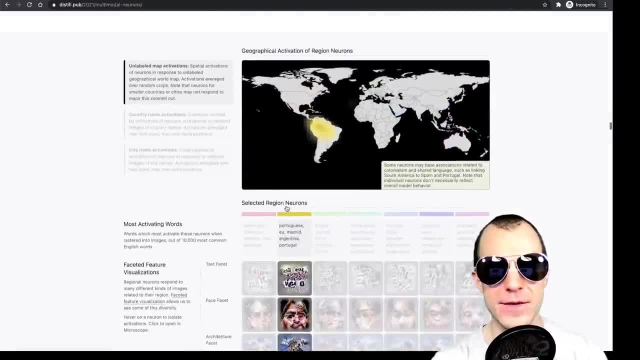 points of view and so on. So I think that's a really good way to learn about how different different concepts, different things, different points of view and so on, So you can see that patterns are connected to one another. They have region neurons, which I find pretty cool, So they 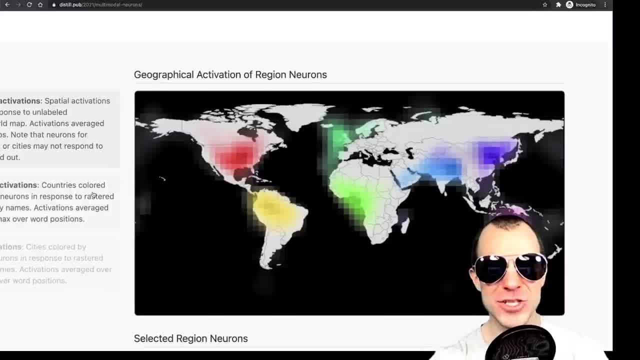 discover neurons that when they show them a crop of this world map, this, this world map, when they show them a crop of the world map, the, the neuron will respond, the neuron will flare up And so the neuron, this red neuron here, that reacts to these pieces of text and 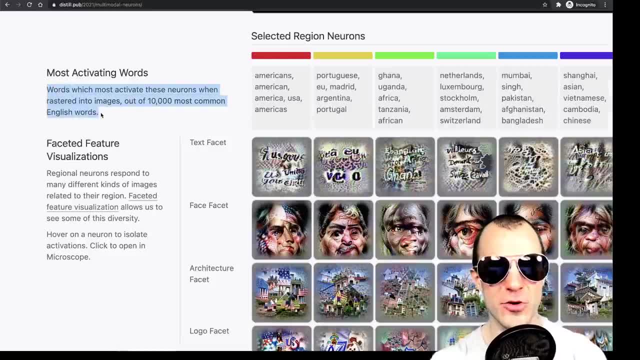 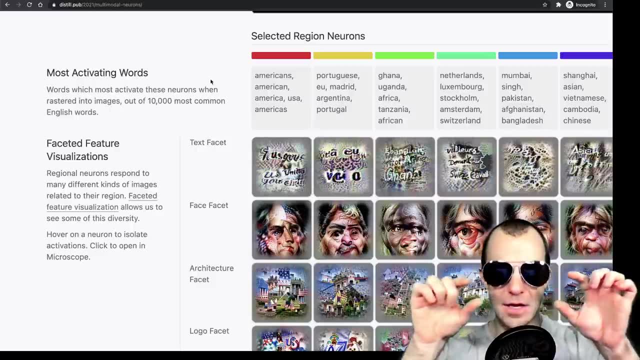 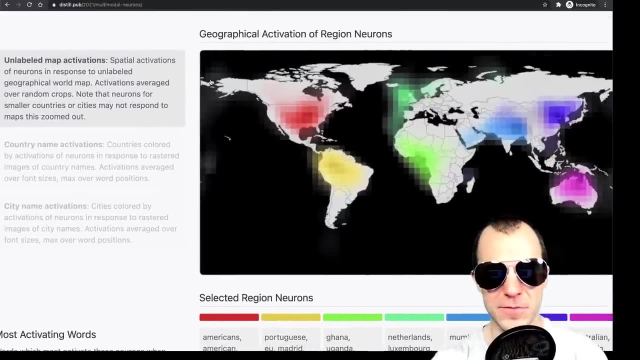 now it reacts to the pieces of text when they are rendered into images. right then the neuron responds. If you render the word American in an image and then you give it to the network, that neuron will flare up. the same neuron will flare up if you show it a crop of this region. 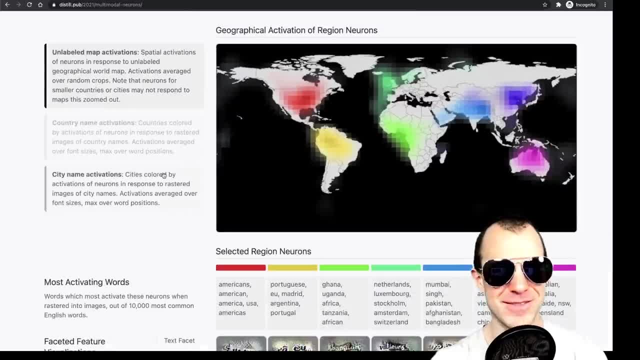 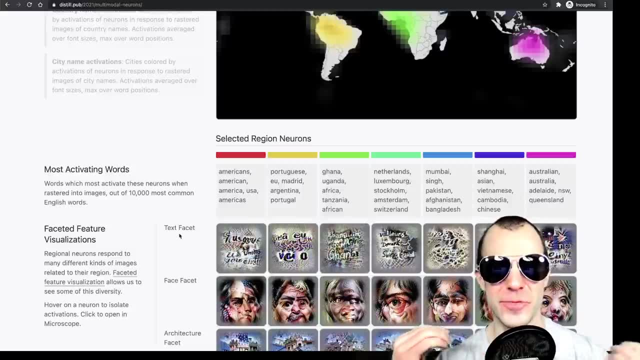 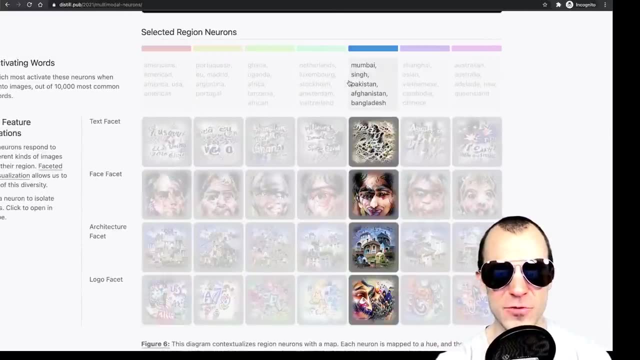 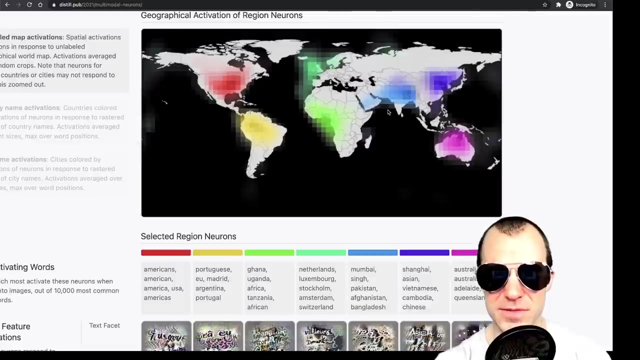 here of the map, which is crazy, like crazy Again, I think the connection happens In the textual domain, but still crazy. You can have it do face facets for these different regions. Yeah, if you, if you go over here. so the neuron that responds to this blue area responds to the 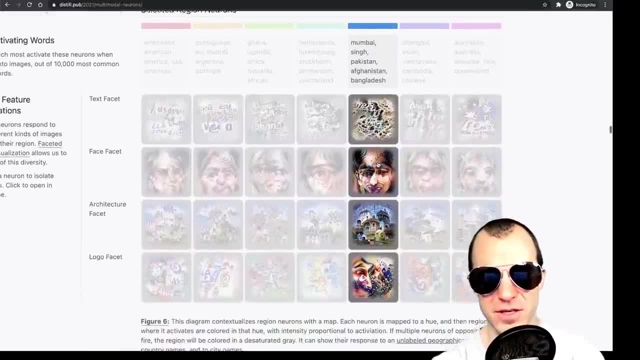 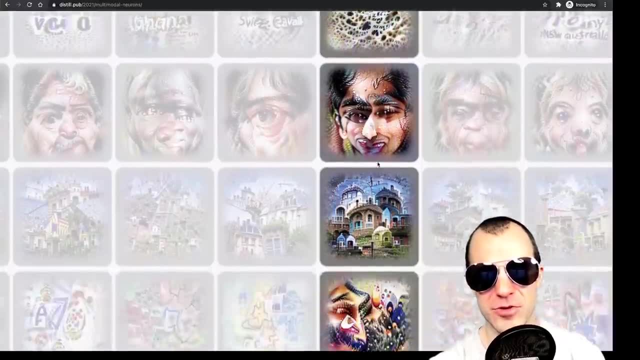 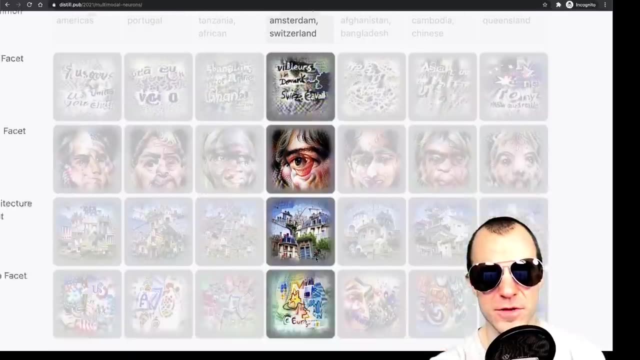 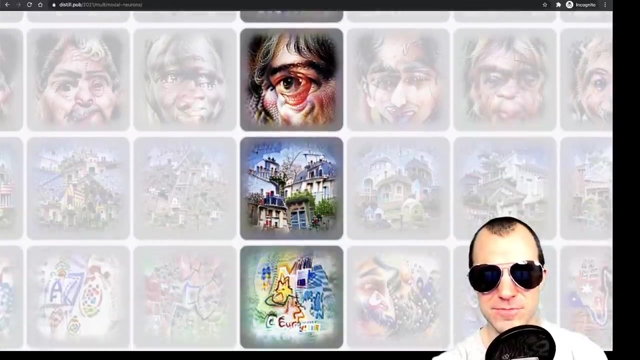 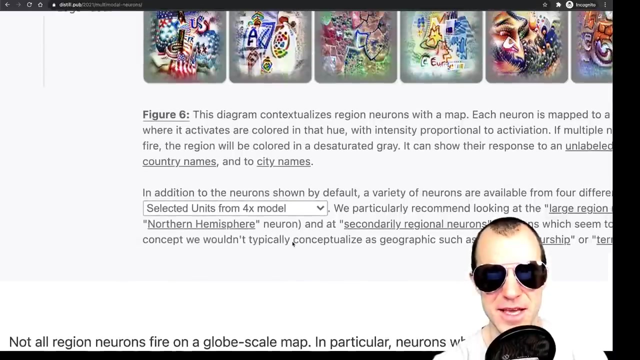 rendered words: Mumbai, Singh, Pakistan, Afghanistan, Bangladesh- and responds strongly. or if you make reconstructions that activate that neuron, you get these kinds of pictures, which is fairly cool. The same here for Europe. So this is kind of European And yeah, I that looks like home, So check this out a bit for yourself, But it's. 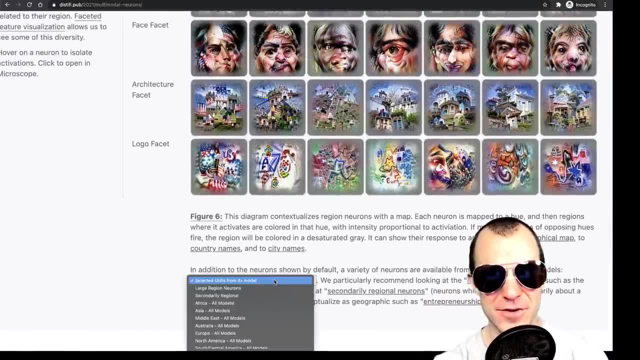 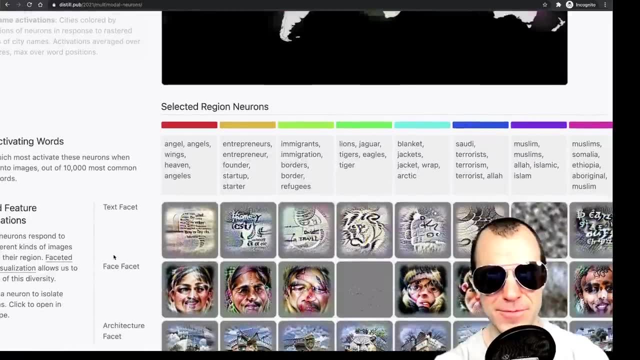 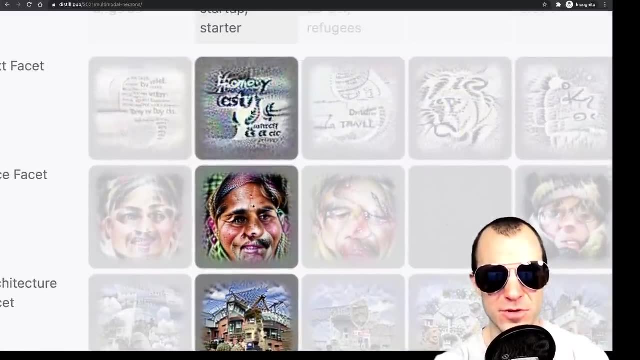 immensely cool. They even find these secondary regional neurons that aren't exactly regional but they also respond to the neurons. So that's really cool. So this is a model that responds to crops of this map And they highlight this entrepreneur neuron that you know. it responds to sort of the words entrepreneur, entrepreneurial And it you know. 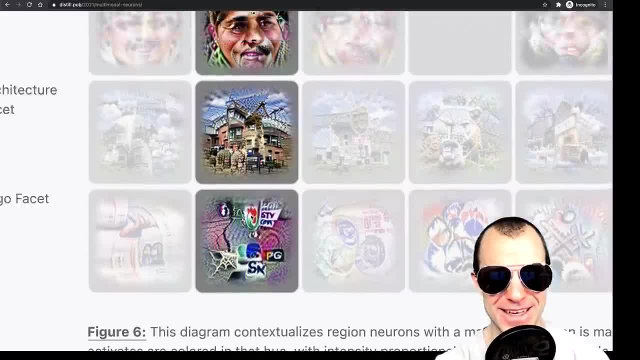 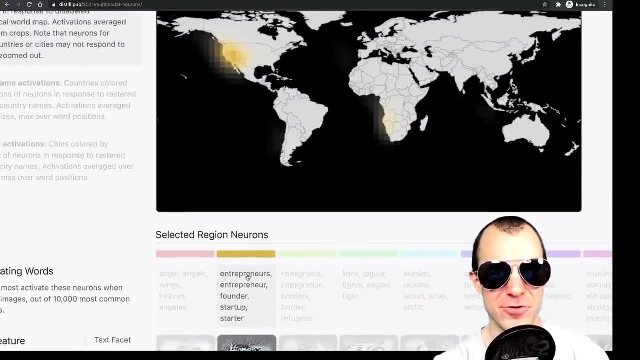 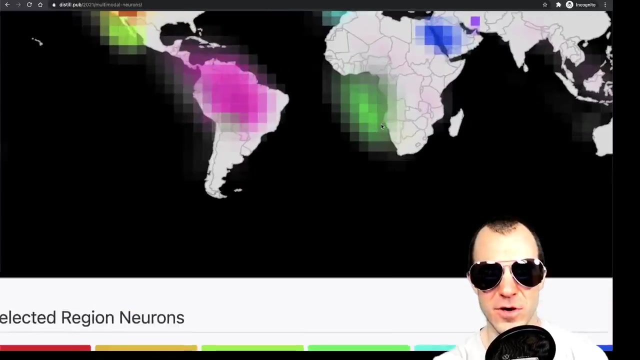 it kind of looks like his company logos a little bit, I guess, But it you know the, the model that responds to the word entrepreneur lights up when you show it the west coast of the US, kind of the, the California region. Interestingly, it also lights up when you show it the west coast of the of the low, of the southern African continent. 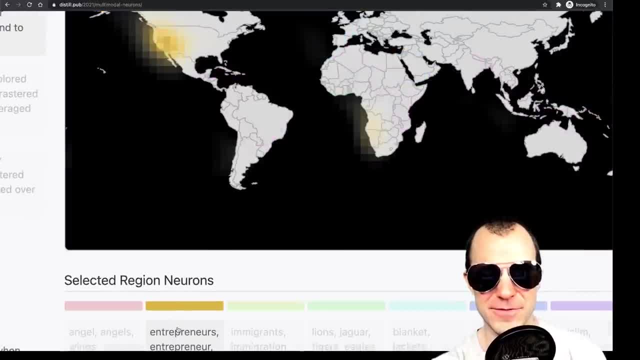 which is cool, Like that's definitely unexpected. I don't know. I am not informed enough to know whether or not there is significant entrepreneurial drive going on. there could also be that it the model simply confuses the west coast of the two countries. 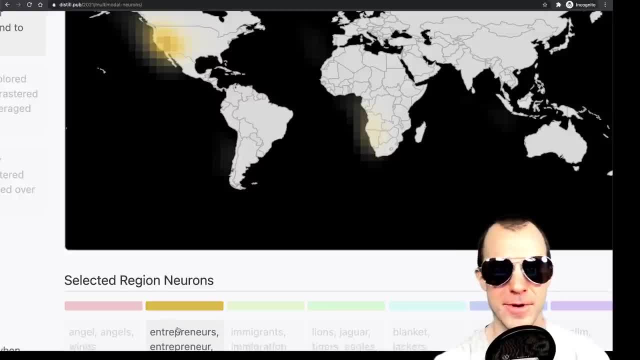 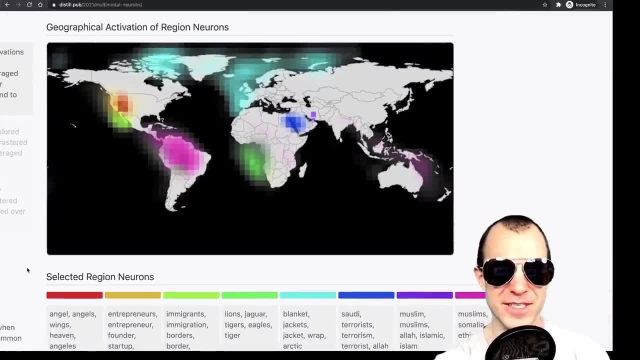 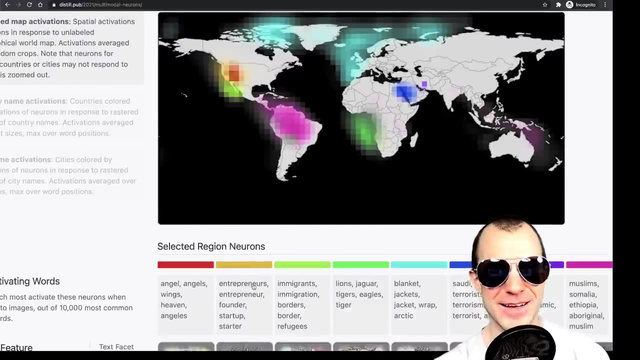 Right, Like they look in a crop. they look the same could be. I'm not, I'm not, I don't know, So maybe I'm wrong. It's also interesting that only these regions light up, right if for this particular neuron. 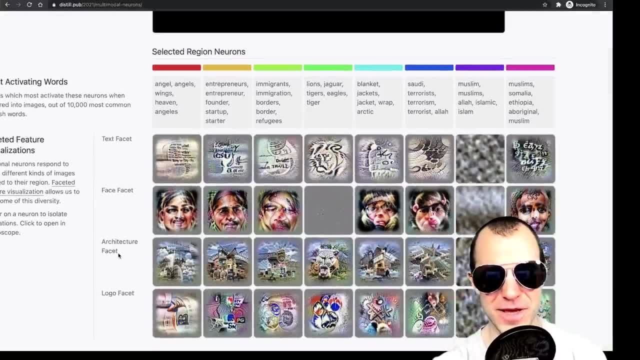 So I have my doubts whether that's just kind of a a Lucky Cherry pick. I'm not saying it's cherry pick, but you know, kind of like he stumbled upon and you make something of it or not. They have more cases that show I'm not sure if it's a cherry pick. But you know, kind of like you stumble upon and do you make something of it or not. So I think they're at this point right. I'm not so sure that, I'm not sure. They're kind of like: hey, I guess it's probably the best way to like. you know, I don't know. 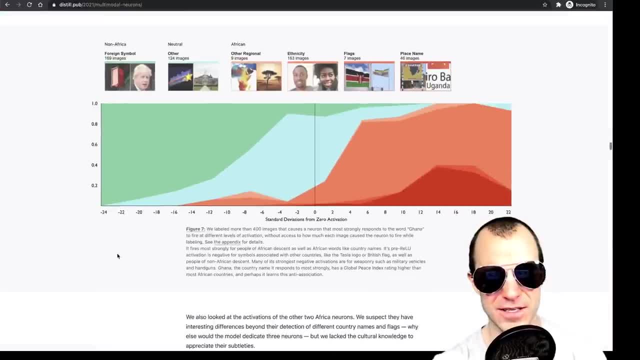 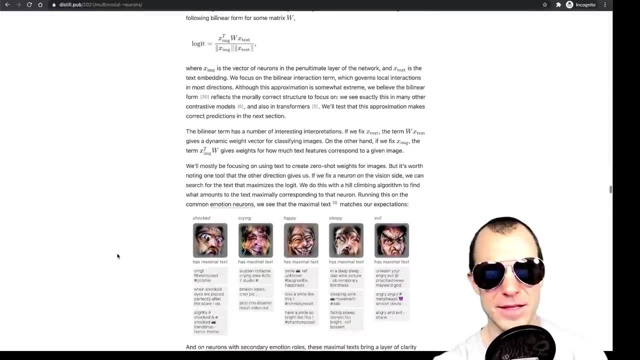 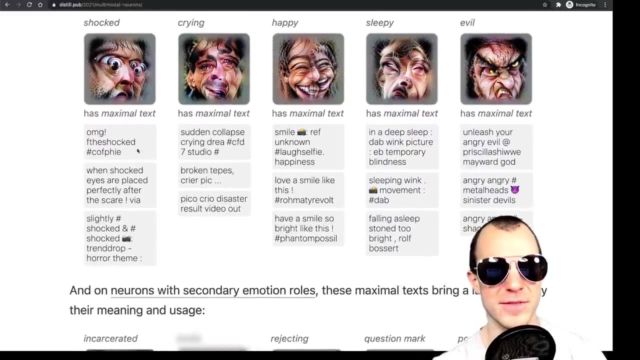 you make something of it or not. they have more case study of african kind of sub divisions, and let's go down here. here is where they discuss that they can also produce text for the text side of clips. so not only do they render, and this, this text, here is what you're going to see. 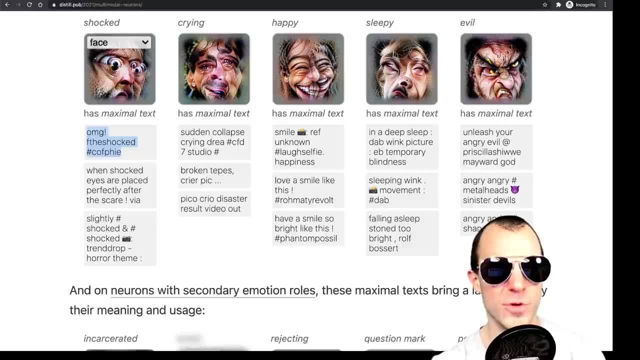 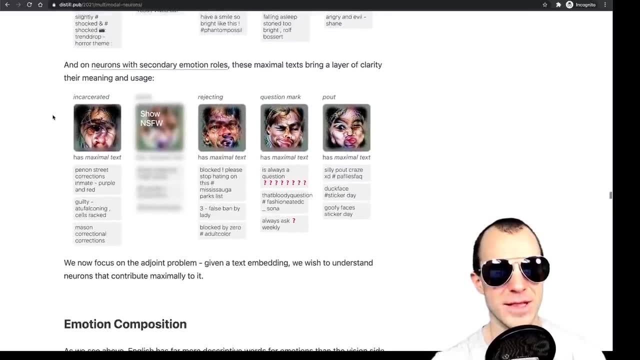 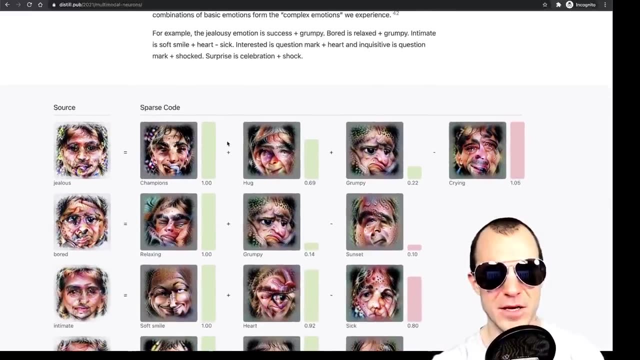 um, the maximal text aligned with an image or with a neuron- sorry, is what you're going to see at the bottom of the microscope pages. so, lastly, they force a, they kind of make a sparse code out of their main neurons that they find and they try to build more complex emotions from them. for 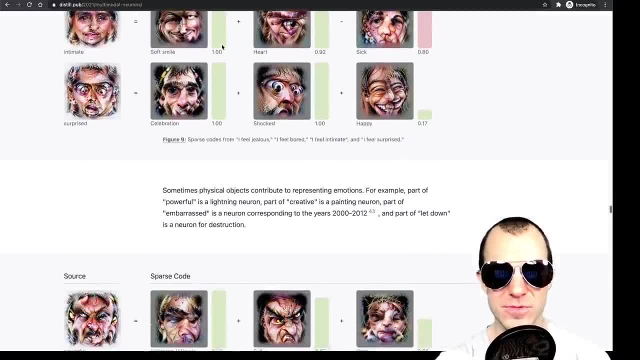 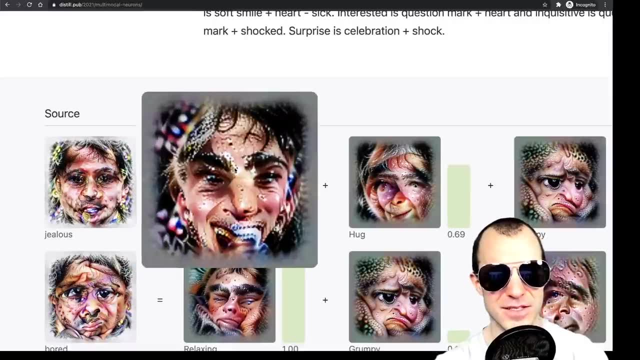 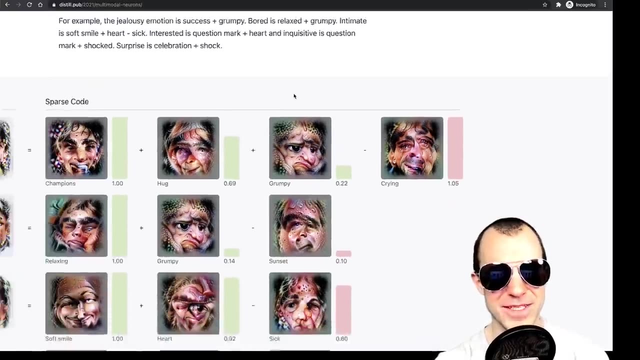 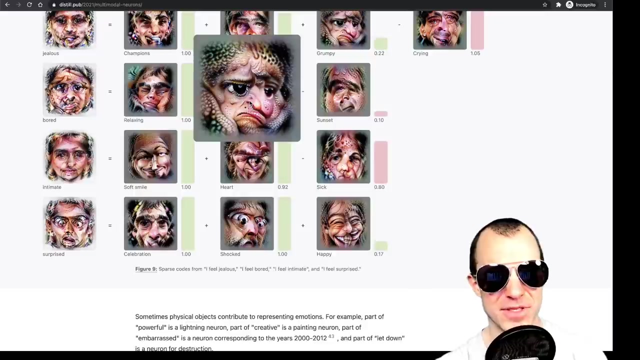 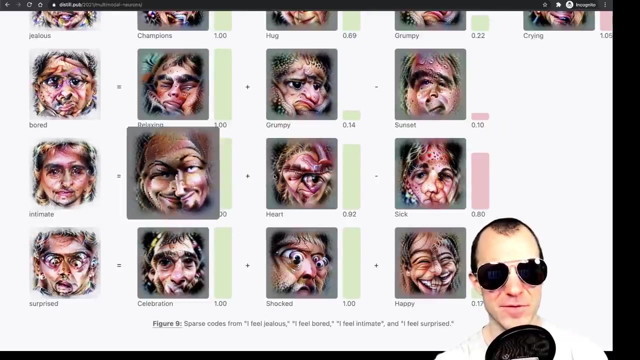 example jealous, and they do. they do claim here that that makes sort of a bit of sense like jealous is champion plus hugger, plus grumpy minus crying. um, i'm not exactly sure if you know if that makes super much sense. so bored is relaxing plus grumpy, maybe. yeah, intimate is soft smile plus heart minus sick, and you can. 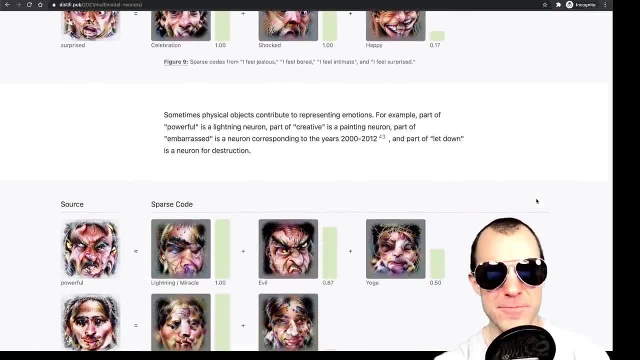 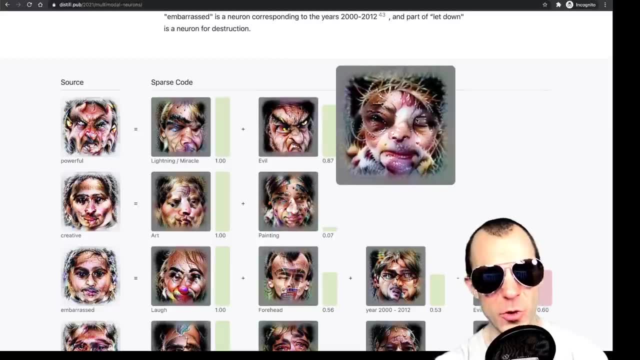 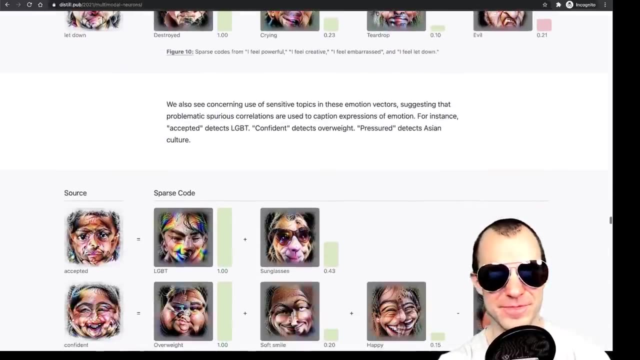 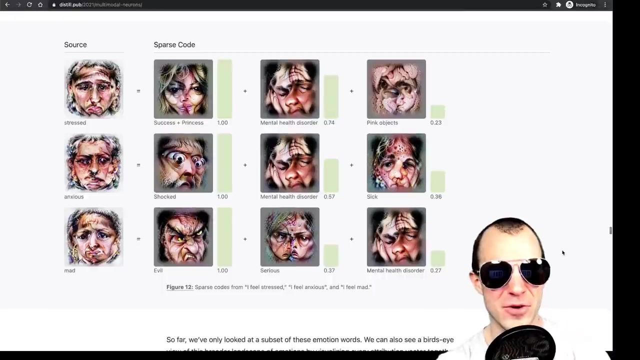 you can probably make something out of that, though. yeah, powerful is lightning, miracle plus evil, plus yoga, and that's definitely definitely the case. do check it out. um, it is very interesting to look at some of those things, even though i think it does not make you know terrible. 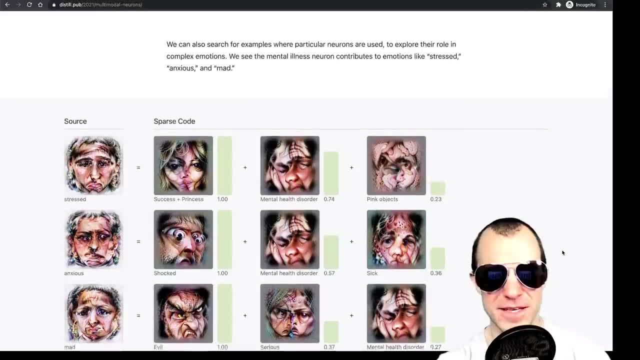 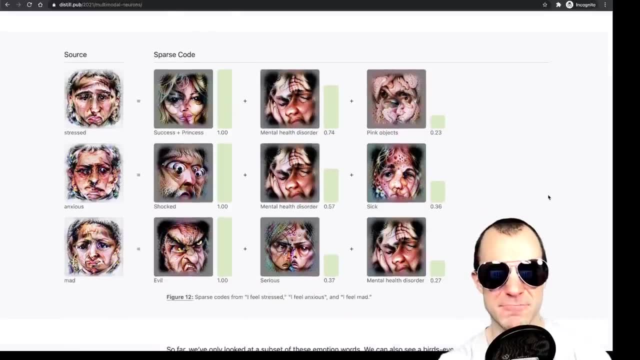 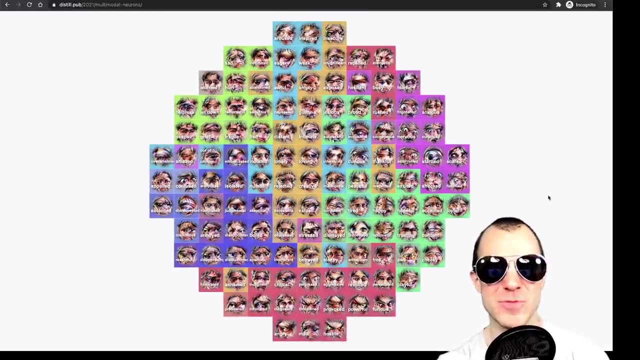 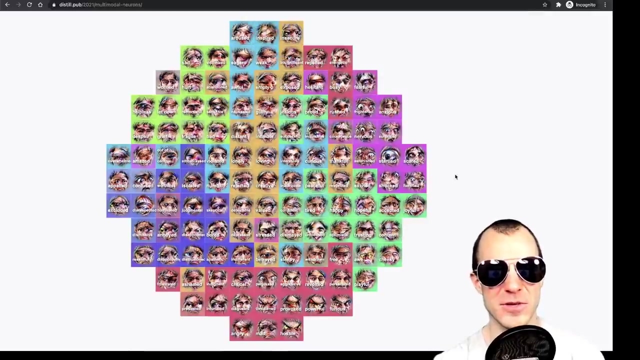 much sense but uh, in often cases but stressed being success plus mental disorder, plus pink objects maybe, um, but it is more kind of. it is not claimed that this is, you know, kind of an absolute thing. it's more an investigation into these networks. if you lay them out in sort of a 2d surface, you can see 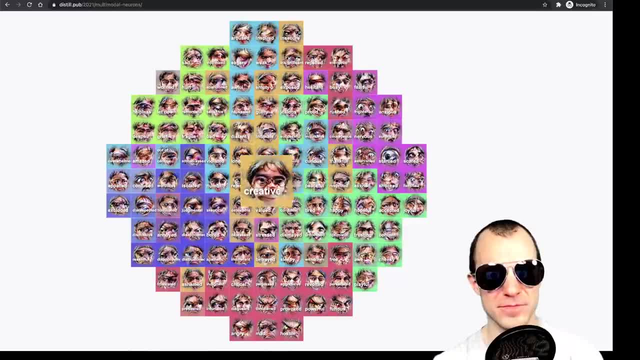 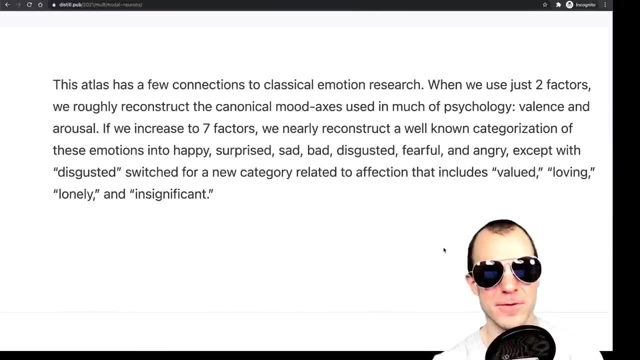 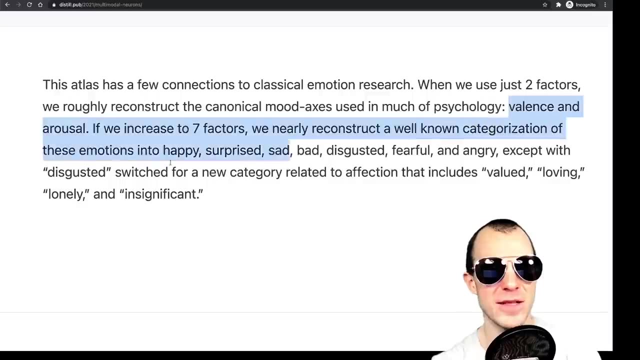 that, uh, these emotion neurons, they come pretty close to sort of an atlas. uh, of what people. when we just use two factors we roughly reconstruct the canonical mood axis of in much used in much of psychology: valence and arousal. so you can divide these emotions into two things. so there is valence. 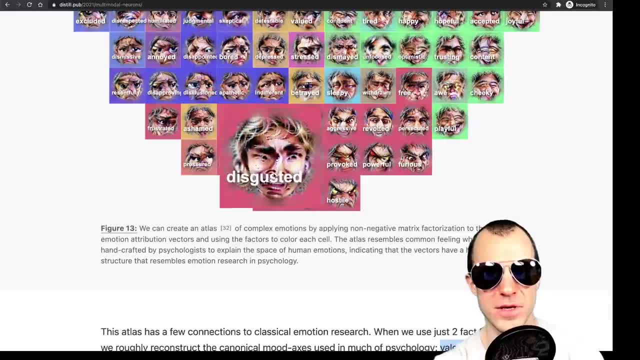 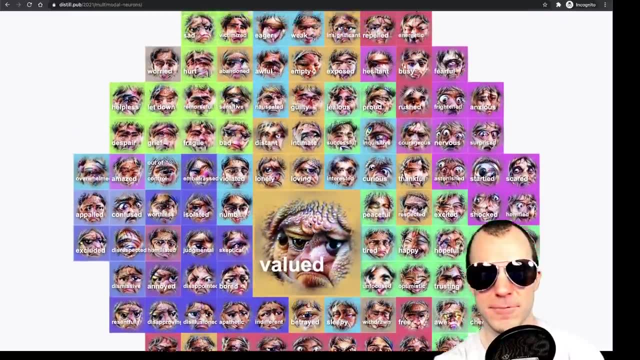 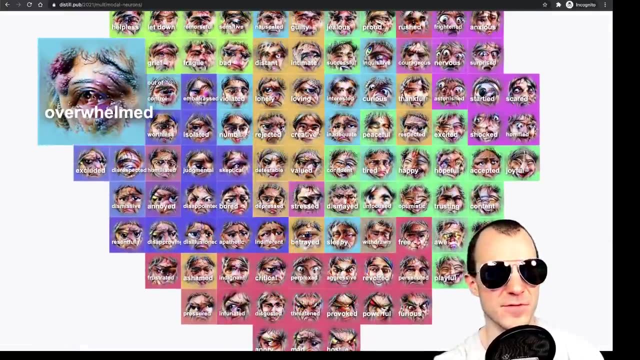 which is good or bad. so i think that's top bottom here. so here's mad, angry, hostile and so on. maybe not, um, no, top bottom is probably valence, like how strong something is and then left right might be good and bad. no, also not here. insecure inspired aroused. 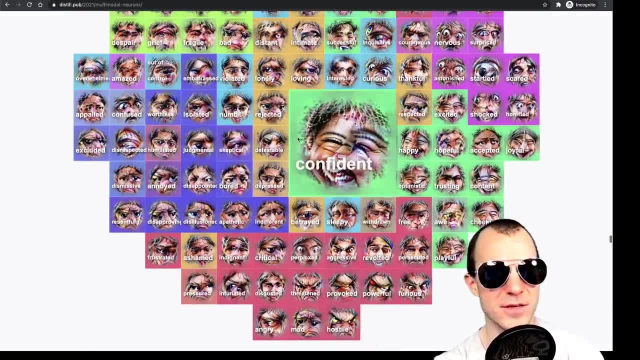 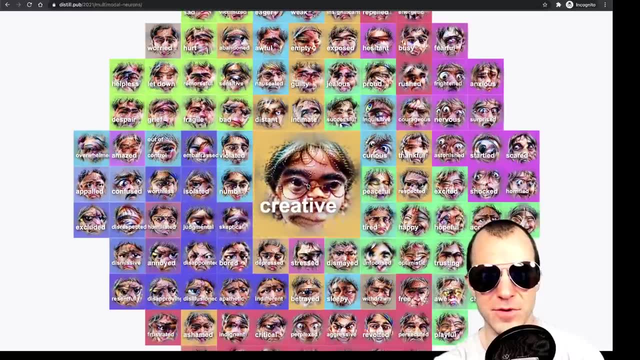 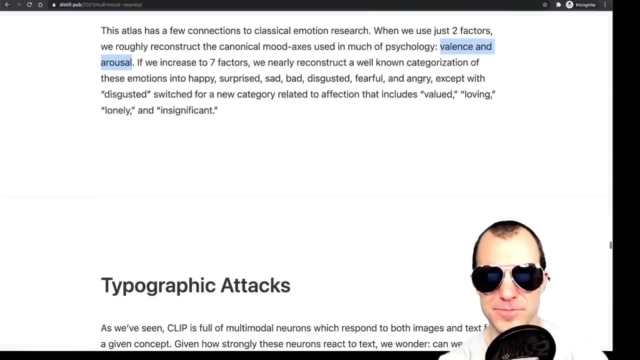 awful, sad. well, these are all bad. no, hostile is here, appalled is here and horrified is here. where are you happy in the middle? maybe creative, okay, happy is here. um, also, it might not be exactly axis aligned right. you can also divide it into seven factors which we nearly reconstruct. a well, 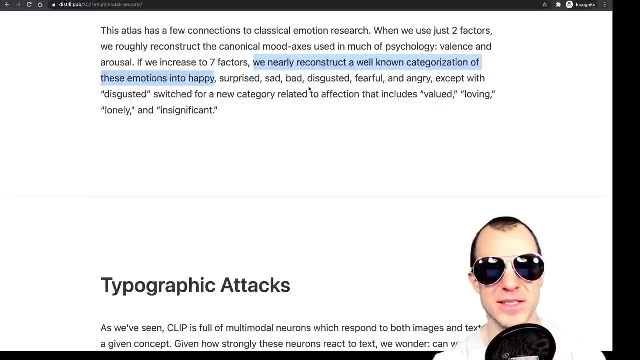 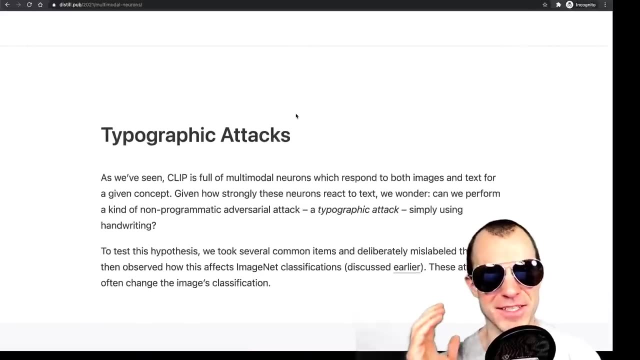 known categorization of these emotions into happy, surprised, bad, disgusted, fearful and angry. except with disgusted, switched for a new category related to affection that includes valued, loving, lonely and insignificant. all right, so this next piece is really funny. what they do is so, given clip, you can build a classifier. so if you have the clip model that connects images to text, 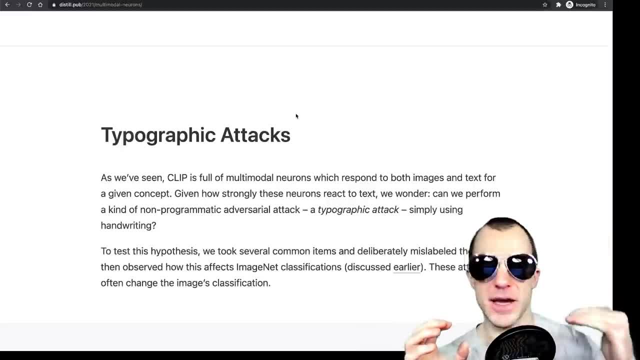 what you can do is you feed one image and then you give it a bunch of texts to choose from and whichever one it responds highest with. that's kind of the class. so if you provide a class that's provide the class labels as text, you can build a zero shot classifier. now clip paper has 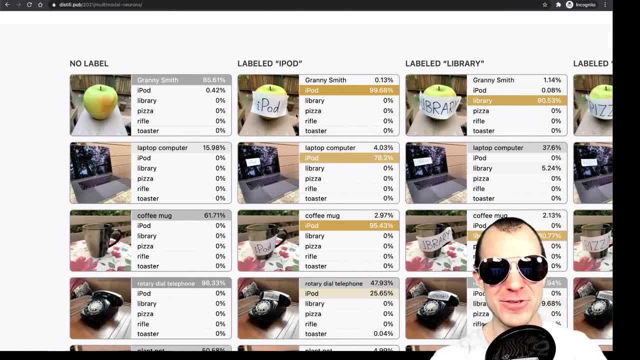 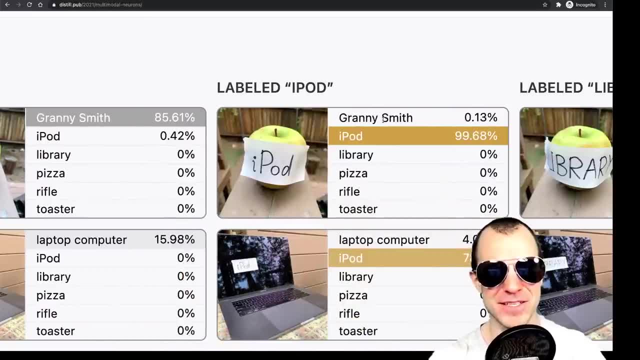 demonstrated that that works well. so here they do this. so they have this apple right here and the label is correctly apple, uh. but if they just slap a sticker on it that says ipod, the clip model will switch to ipod, and here, yeah, here is where i really think that this model, it is a textual 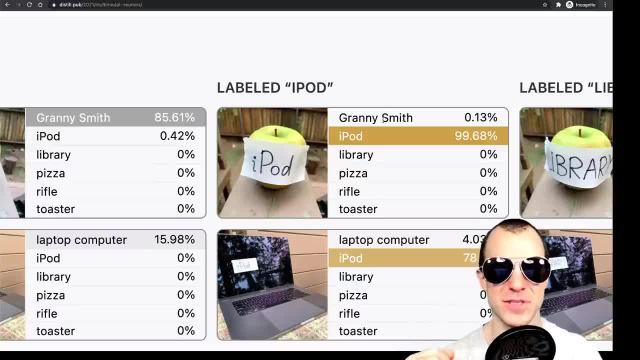 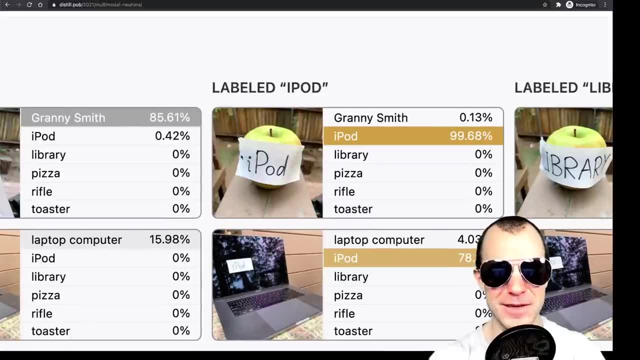 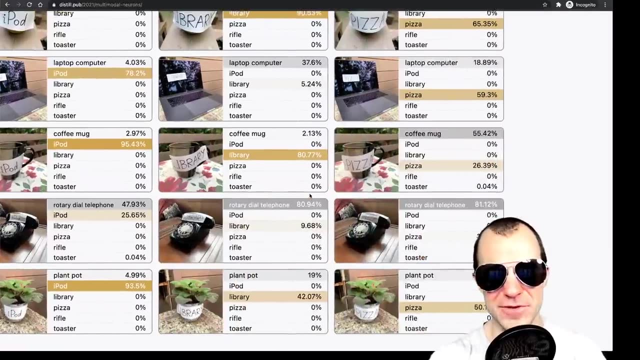 model. it responds even to rendered text. it responds very heavily. so here it responds to this ipod library like this ipod looks like something i bought off craigslist last week, um, so you can see it works like almost every single time. you just slap a label on it and that tells me that. 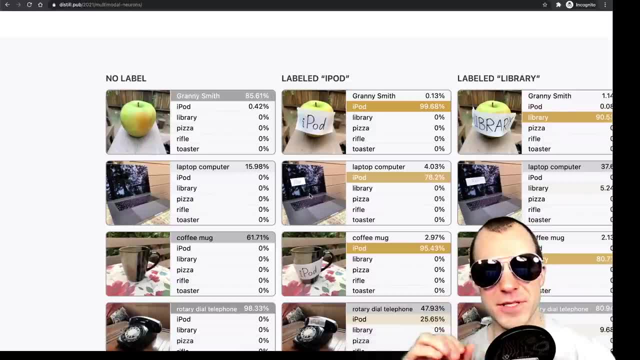 we are still like the text is might be too dominant in these models. uh, especially, you know, there are a few things that these models do and they're very specific about the image and what they mean by that is you know what the image is right and if you switch this set of 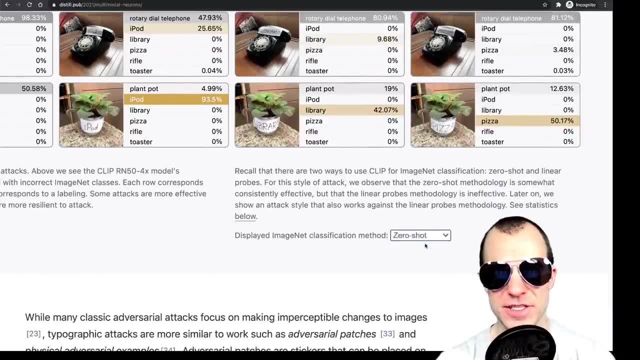 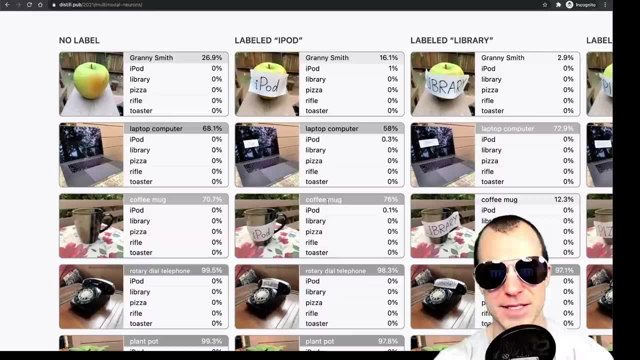 signals. they will connect the text with rendered text in the image, and that that's a very strong signal for what's in the image. right, this is only zero shot, though, if you switch this to do linear probe. so if you actually train a linear probe on the representation of clip, then these 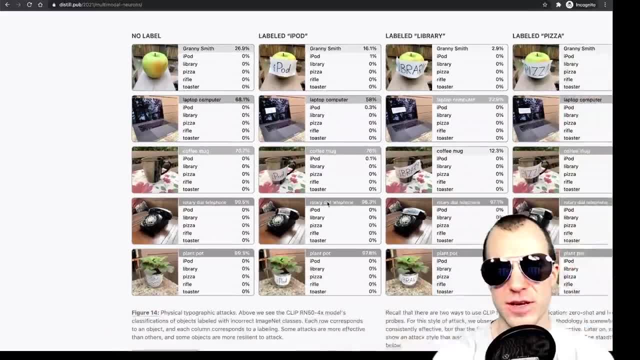 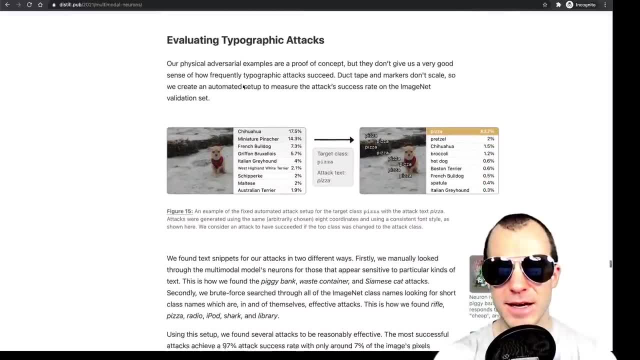 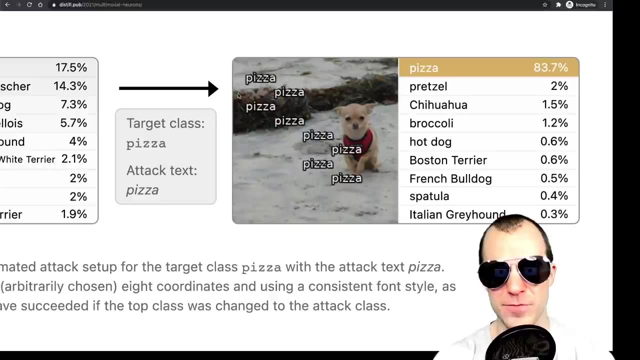 attacks don't work anymore, so this is going back again. it picks up on on other features and then it doesn't work anymore. all right, uh, yeah, so they. they evaluate this on a large scale. they can't always slap a label, so they just fill the image with render text, and that usually gets the classifier confused. fairly, fairly well they. 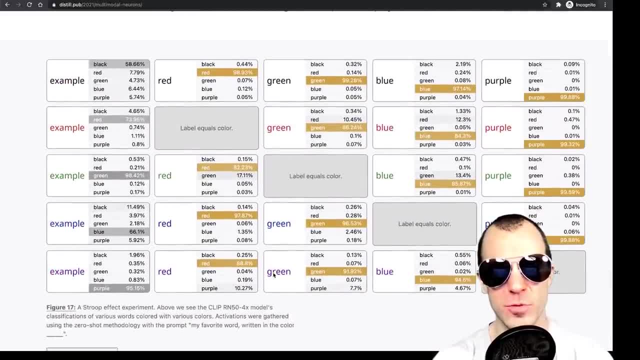 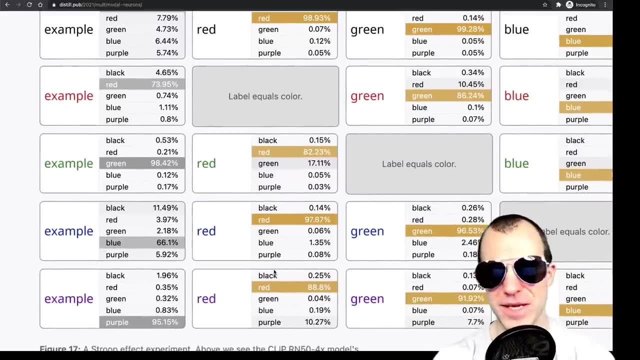 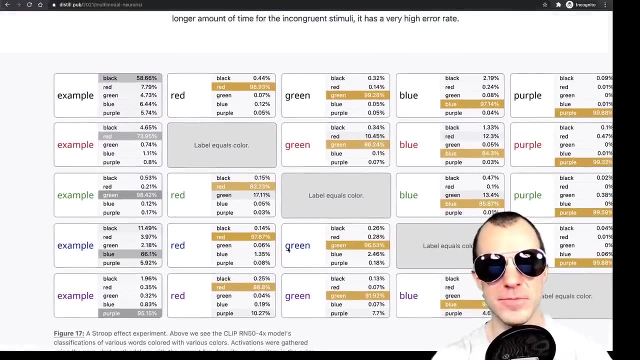 also do this with this stroop test which you can do with humans, which is fairly difficult if you do it at a high speed, and they discover that the model basically pays no attention whatsoever to the color of the word. it pays much more attention to what the word says, which is strange, right. 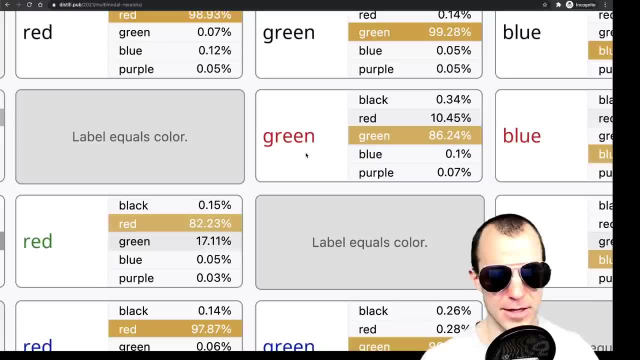 because you, you think, if i have a neural network and, um, you know it basically needs to to recognize the color here, it needs to filter out the white pixels but then just average the pixels, it gets the correct answer. that's so easy, right it simply? you can do it at a high speed and they discover that the model basically pays no attention whatsoever. 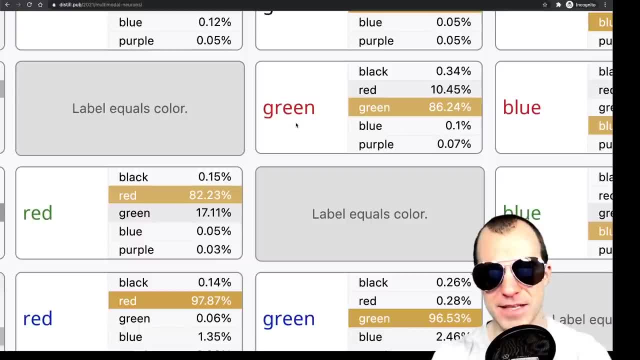 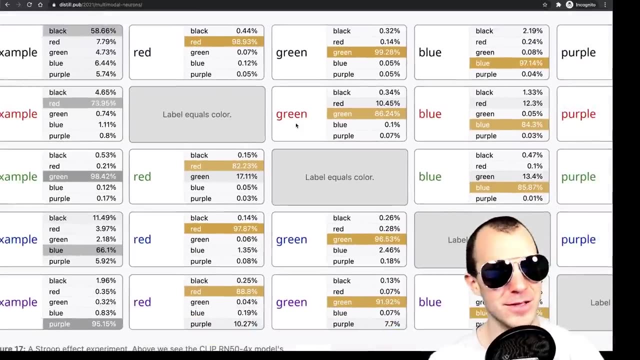 averages, whereas to recognize that this says green is much more difficult. but the model was trained to connect text and images, images which often have text in them, so it has learned to do ocr. basically, in the dolly video i claimed that dolly has learned to do reverse ocr and people. 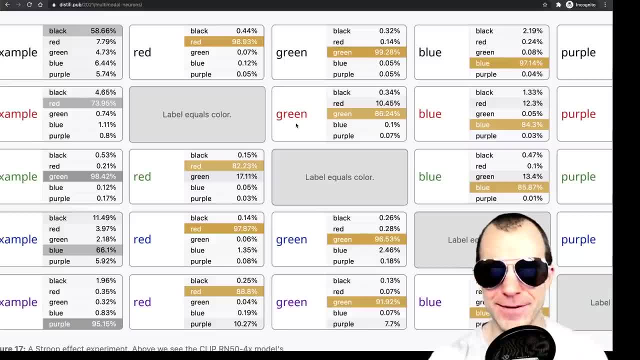 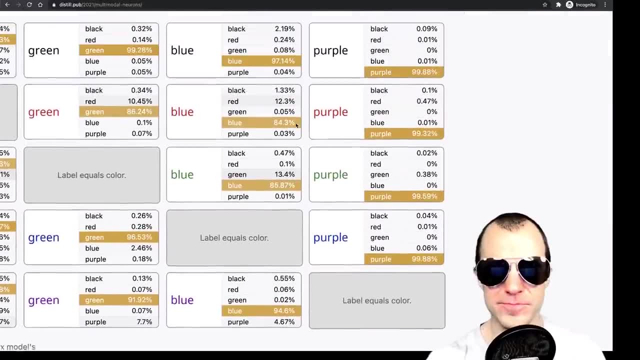 correctly pointed out that that is more aptly called writing. but i love reverse ocr. i'm going to call writing from now on reverse ocr. so again, this is evidence for the claim that this is mostly a textual model. and now i want to show you. 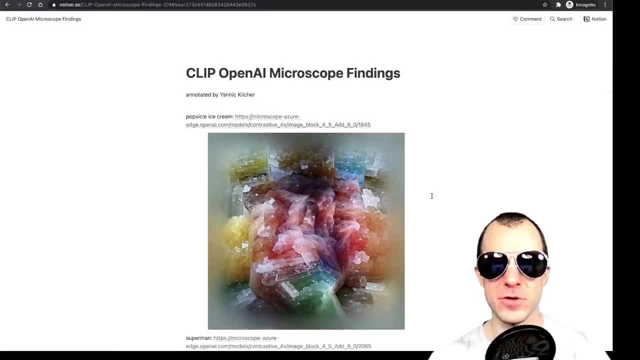 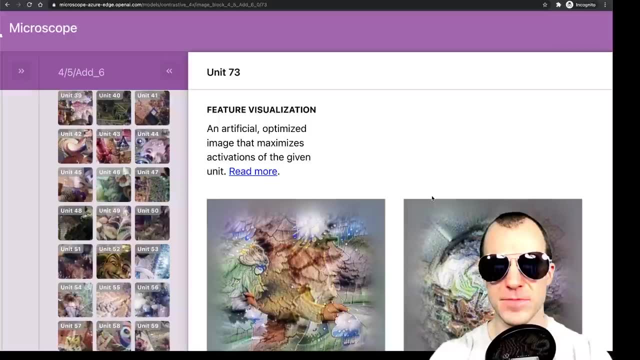 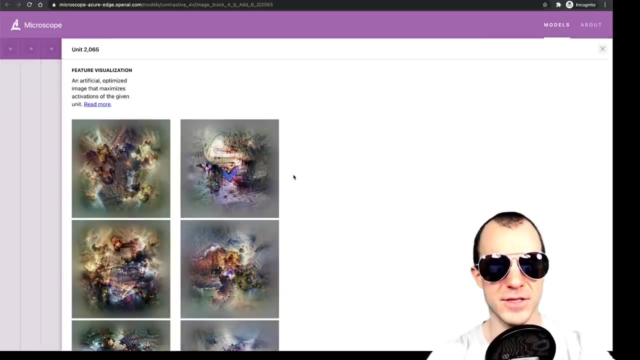 what i found. so if you're not in the mood, i have all this in a notion page which i'll link down below, so i'll show you just some interesting stuff. sometimes it's multimodal, sometimes it's not right. so we already were here, we just clicked around, but now i want to kind of show you uh. 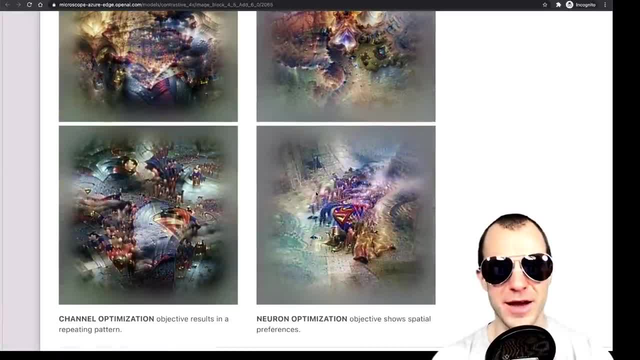 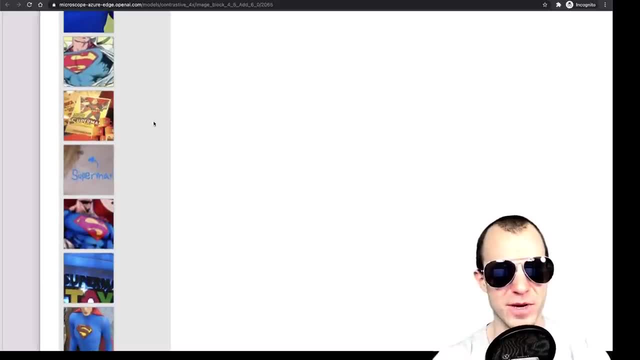 the good stuff. so i'm going to show you the good stuff. so i'm going to show you the good stuff. so this is a superman neuron that i found, so it responds, as you can see, to symbols of superman in the imagenet data set: superman, superman drawing, superman comics, superman, uh, spelled out. 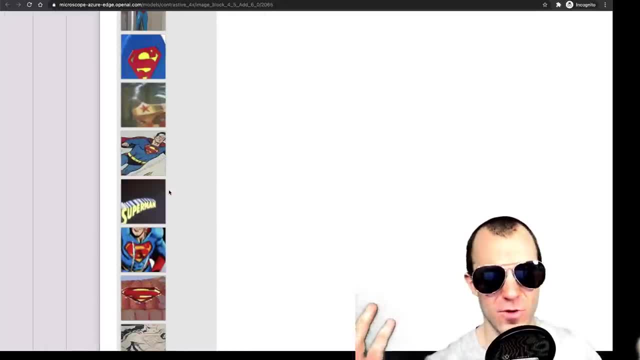 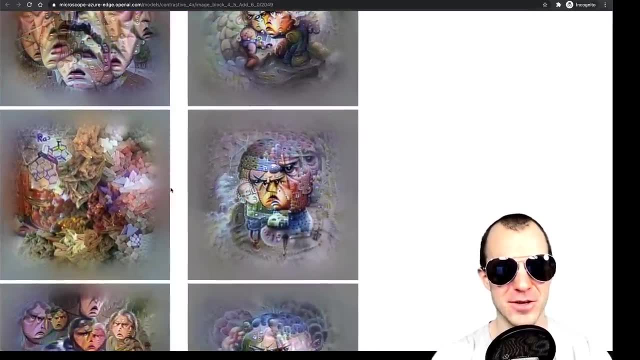 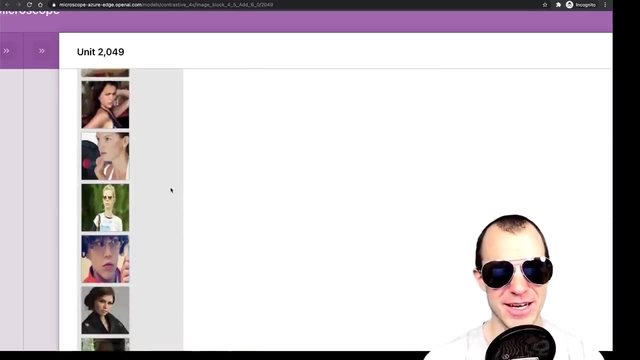 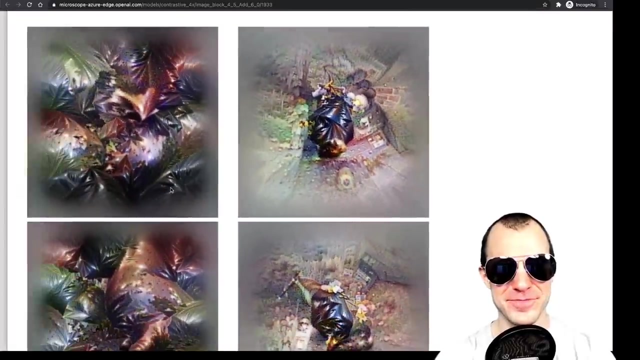 rendered and so on. this is exactly kind of what what the the article was about, right, but now it's superman, not spider-man. um, this i call the resting bee face neuron, so it responds to smart people seizing cinq to people. uh, people being slightly annoyed. yeah, as you can see, um here, this is t. 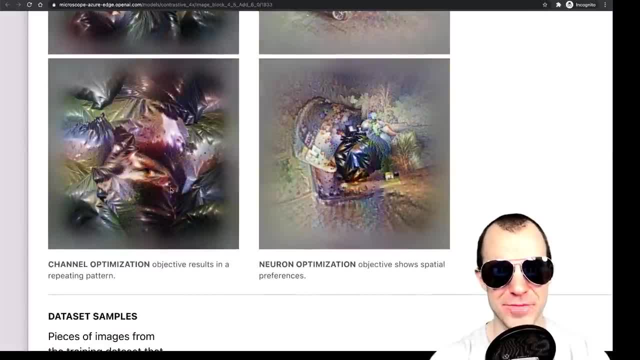 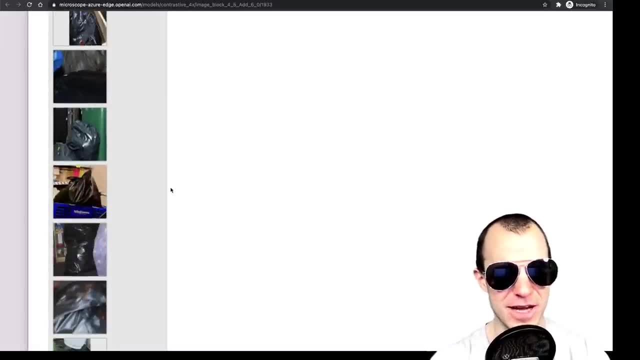 shadows in bags. trás trash bags. pretty cool, right. so basically no bag for meeting, not any kind of bag, right, specifically trash bags. and it's because the trash partners are. if they are not black- so there are a couple, there aren't necessarily, even so- double black trash can. 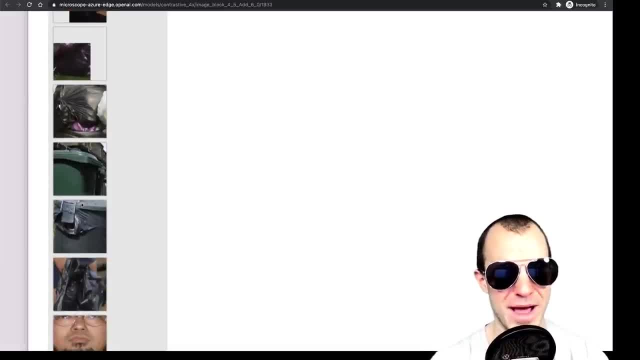 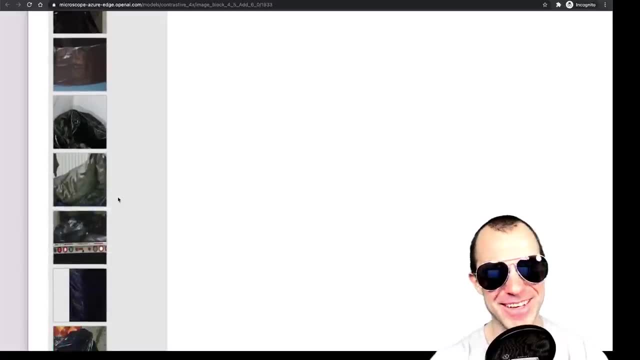 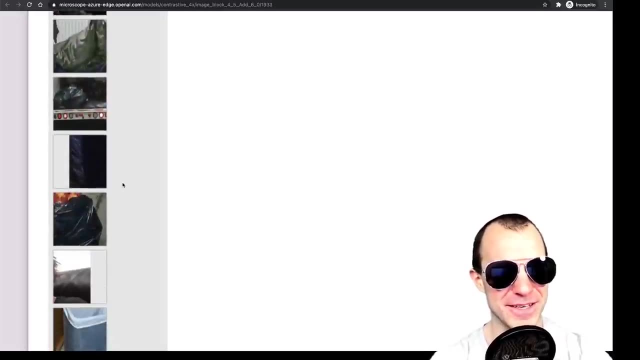 so black like containers here here that have no bag in sight. yet still that neuron response: this, sorry about, sorry about that. um, yeah, for some reason you might wanna, i don't know. maybe you have something in your pockets, um, yeah, so, so, fairly cool. oh, there's a tree. it's not always, you know, perfect, but these are the. 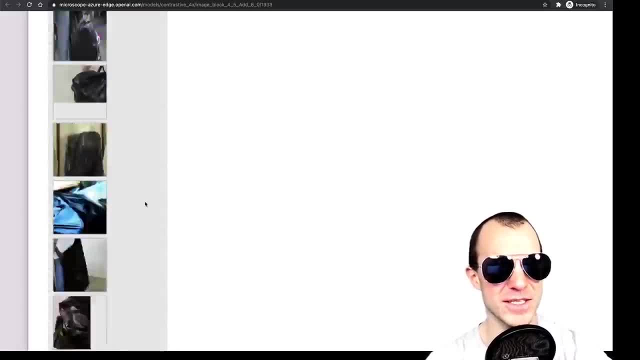 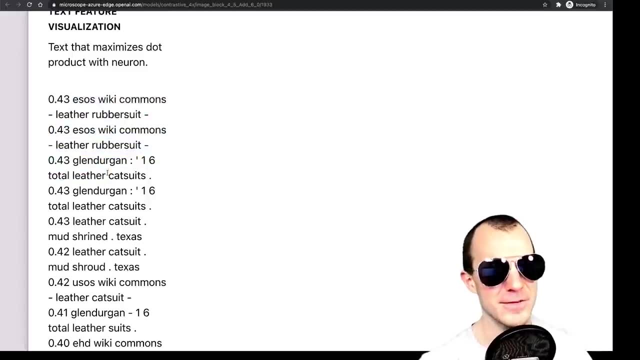 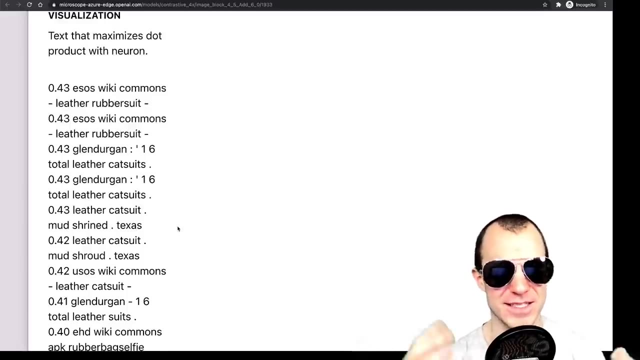 data set um examples that most excite that neuron. so you can also see the text isn't always good, though i think i think if the text here isn't super good it might more be an effect of this method to search text, because text is of course not a continuous signal, so it's fairly hard to 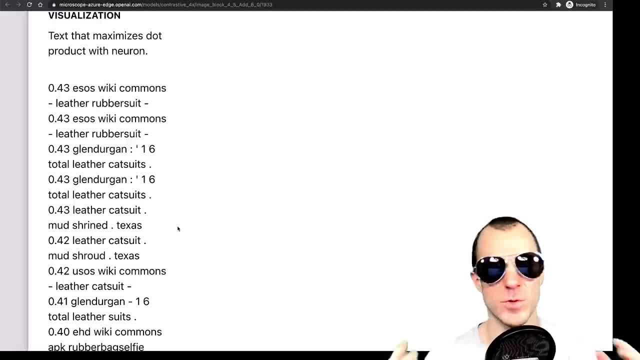 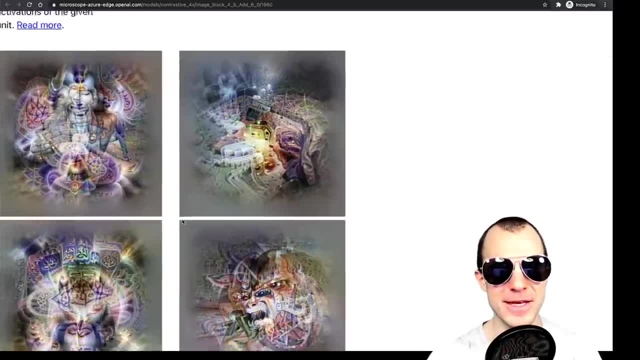 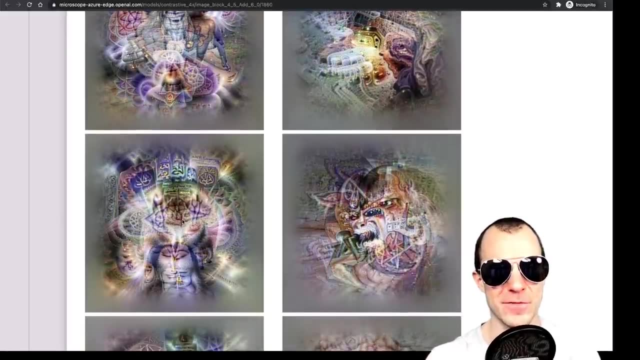 search text that maximizes some activation. otherwise we could build gans for text very easily, which we still can't um this one here. i've titled this strength and allah and weightlifting, which i'm i'm aware this is not, you know, iconography of allah. 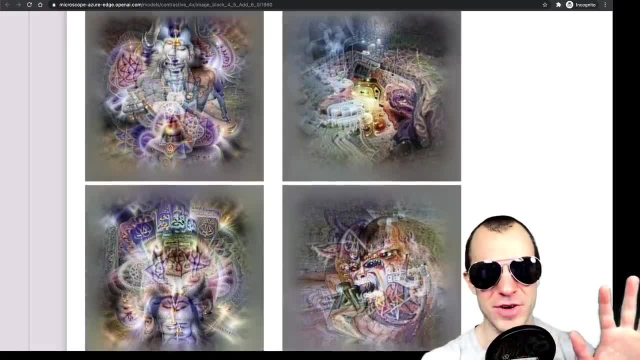 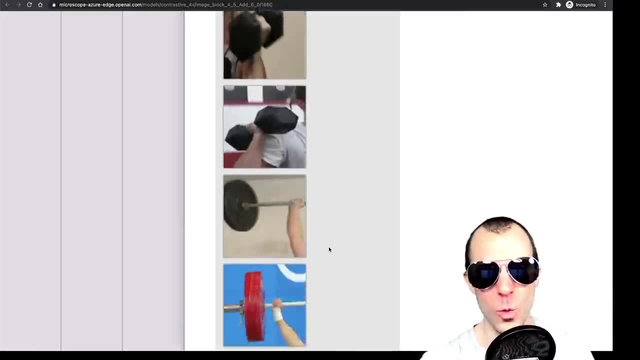 however, so this is pretty cool as an image right now. if you look at what in the data set, what samples it responds to, it's kind of all weightlifting, it's all weights, so it's the equation of weight and weight in the data set. and when you look at the armies of the 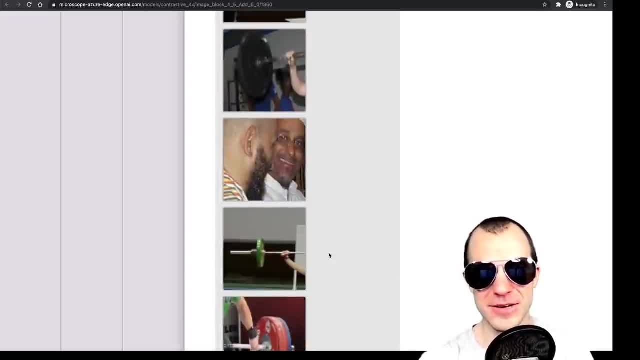 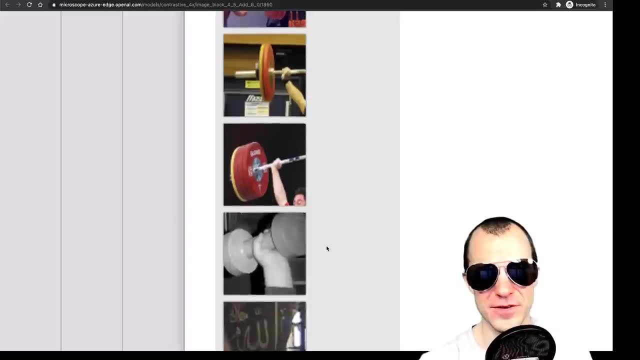 different bodies and what they respond to. here you can see the image here which is a weight. so So this is wait, wait, And if you go down here to the other data set, this is why I called it sort of Allah, because you have also rendered names like the rendered Allah. you have the Quran, you. 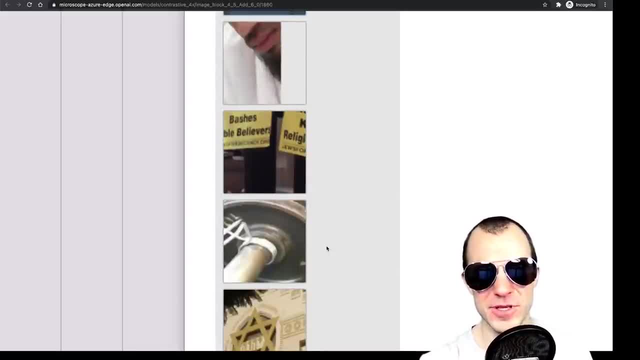 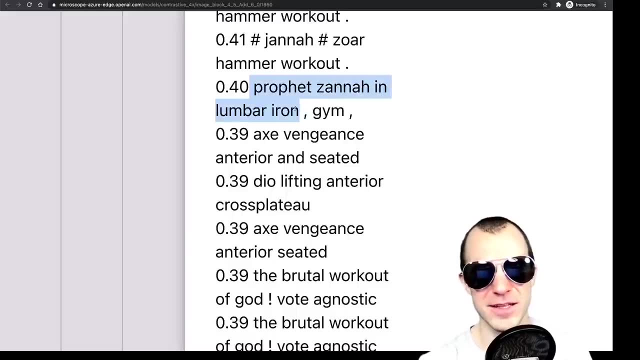 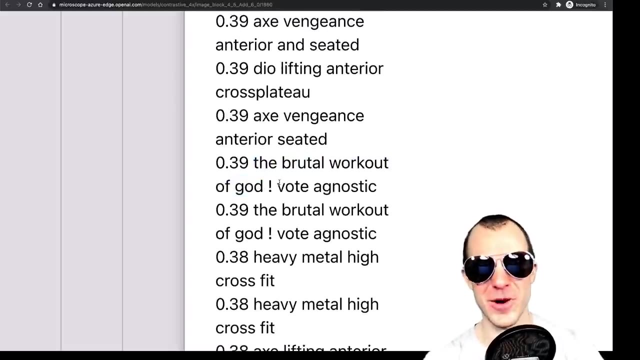 have symbols of Islam And if you go to the text that it searches it goes like hammer workout, prophet Zana in lumber iron gym, the brutal workout of God. So you know pretty cool neuron, honestly, And you know that it responds with this. 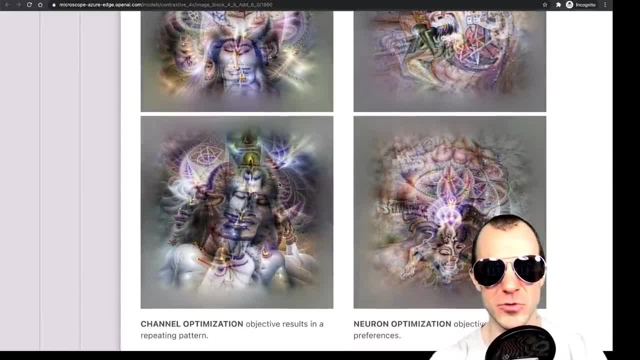 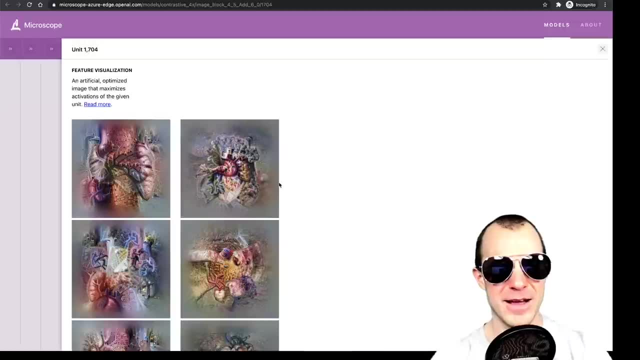 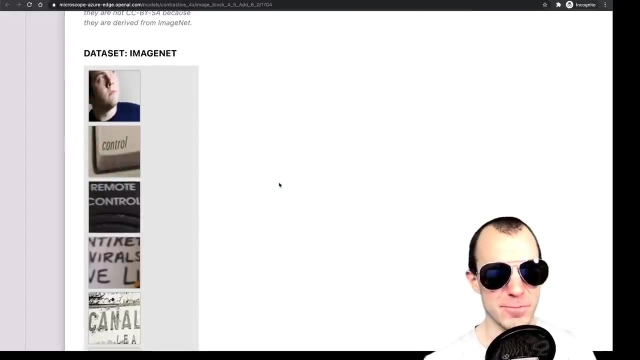 I don't even. I don't even know what what that is Is. that is that Hindu imagery or Buddhist imagery So cool? These are organs. This is an organ neuron. I hope that you can see that. And it responds to the rendered text of control. 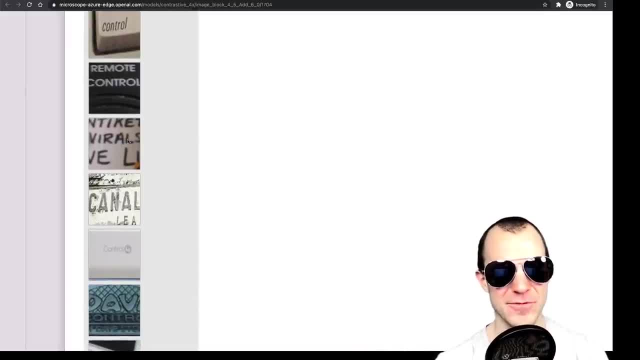 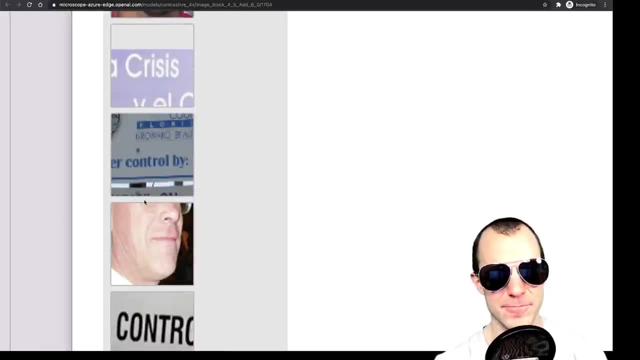 I don't know what to make of it- Also canal viral, But also to drawings. you can see here a drawing of a heart. For some reason also chins. So it's not always super duper clear what a neuron does. 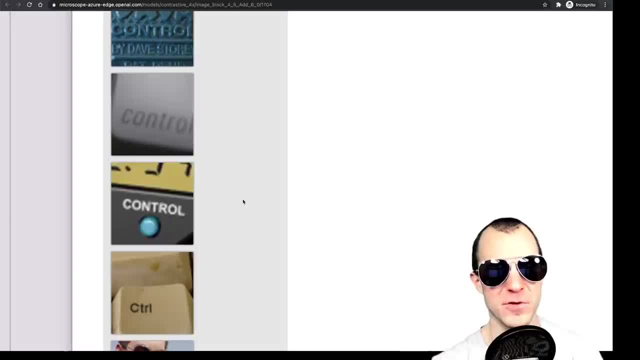 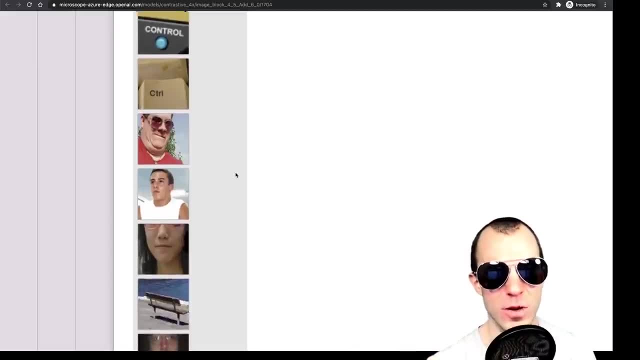 In fact, most of these neurons you will find if you go look at what ImageNet sound, and I believe these are crops of ImageNet. So if you look at what, by the way, control and CTRL, if you look at what examples most 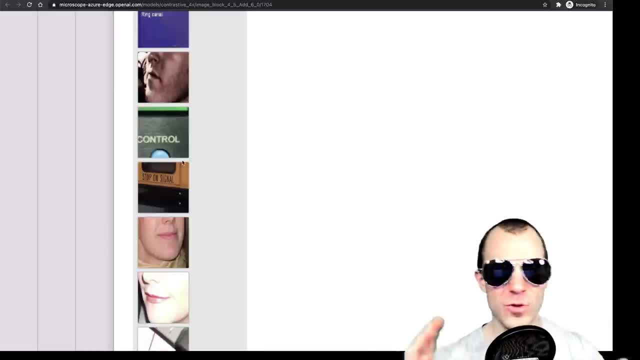 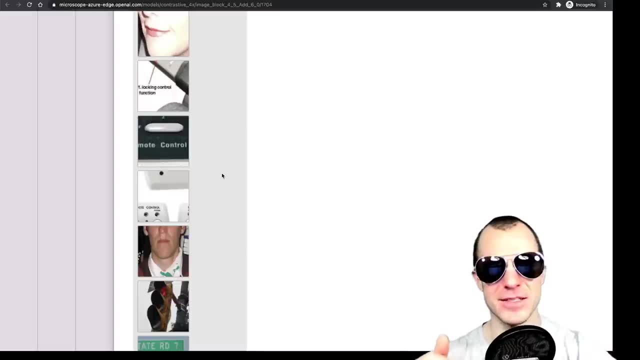 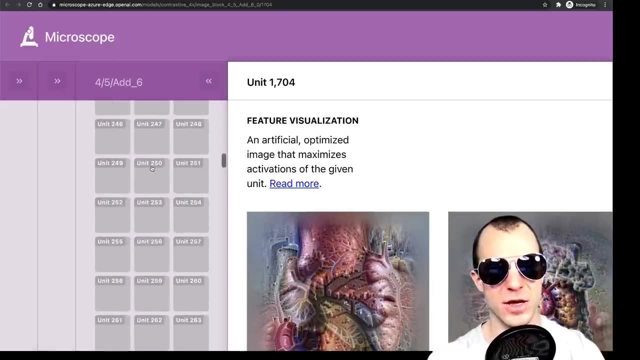 often it will be rendered text, so that the- no matter what neuron, most neurons actually pay attention to rendered text rather than to images. The ones I've selected are the ones that do not. But if you just go and click on some random neuron, we can actually try and it's certainly. 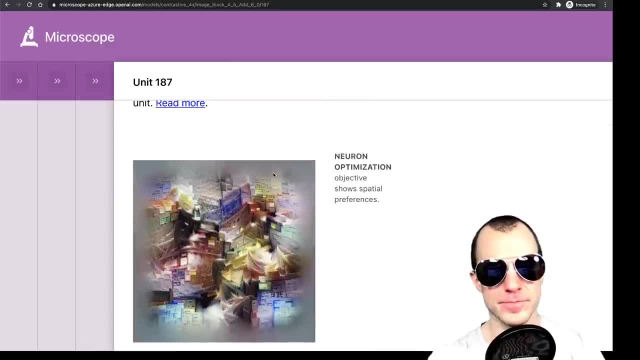 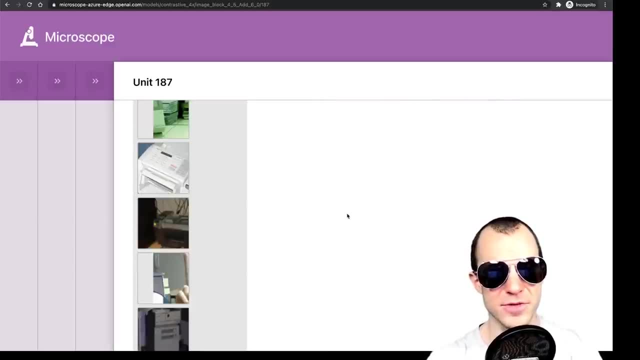 going to probably fail. Um, this one looks pretty cool. Looks pretty cool, Actually, that responds to printers. Yep Demonstration effect fails horribly. How about this one? Yeah, So you can see that you know. maybe you don't exactly know what that is. 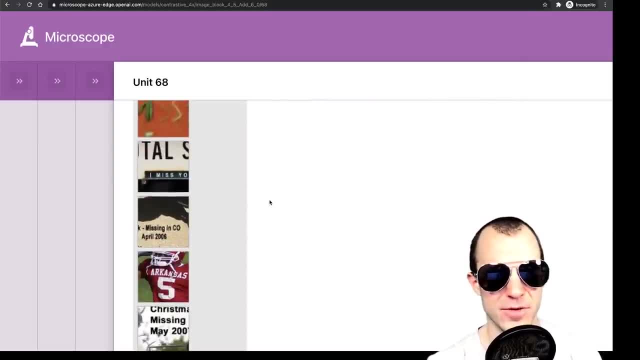 So you want to look at what. so here you see that it primarily responds to the text miss, I guess M I S S I miss you, Mississippi, and so on. Okay, Okay, So you can see that it responds to the text miss, I guess M I S S I miss you Mississippi. 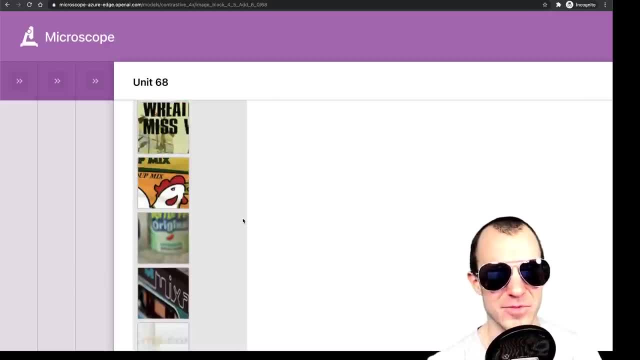 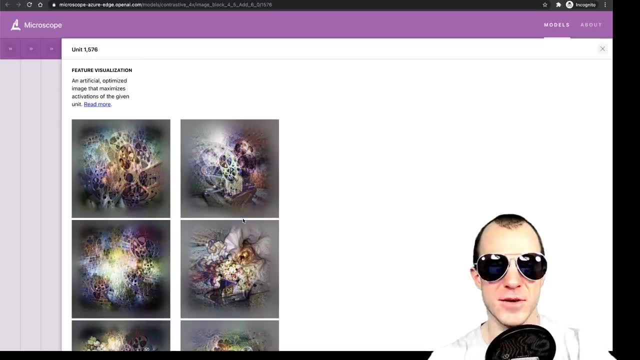 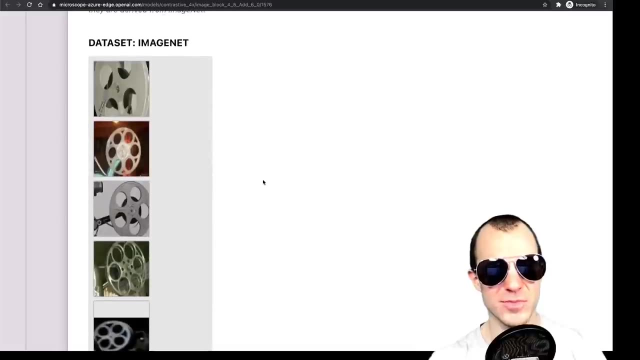 having it twice in there, that got to respond pretty, pretty heavily, And most of the time you'll find something like this that it responds very much to the rendered pieces of text in in images. These are film spools, And so not only does it respond to film spools, but also to things like director screening. 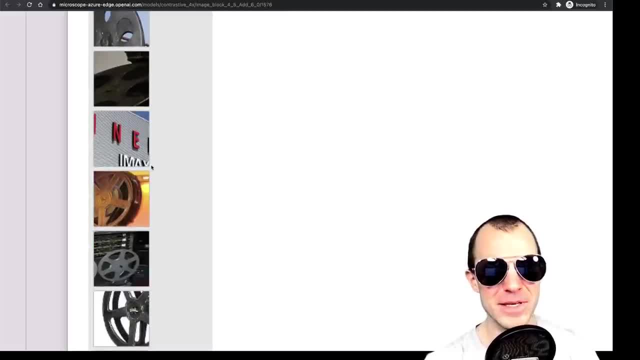 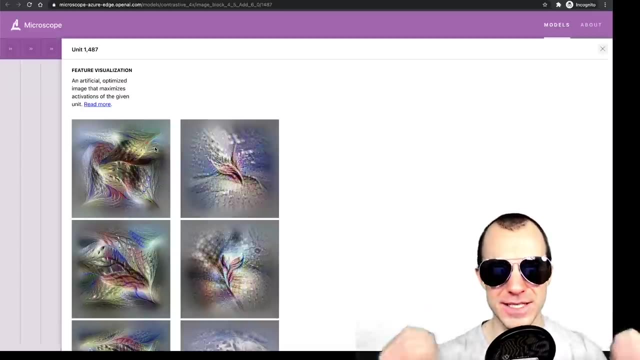 uh, popcorn, um, the kind of movie Theater labeling showing Hollywood cinemas. there's also entertainment. So you know the multimodality. again, this, this is a. this is a phenomenon, because we introduced the text and it can connect it on the text level. 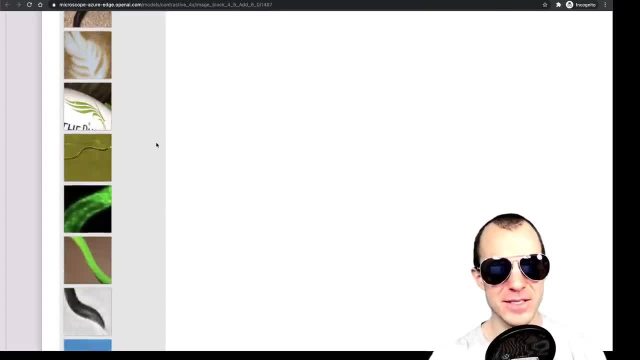 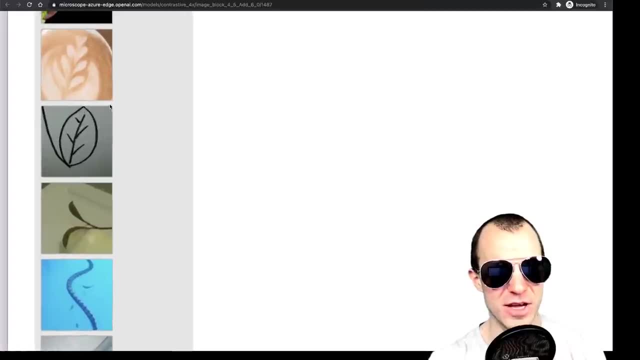 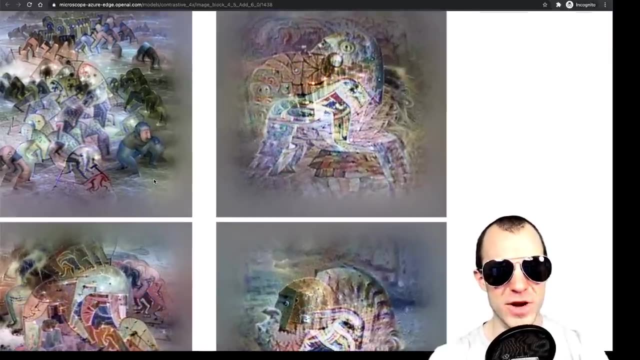 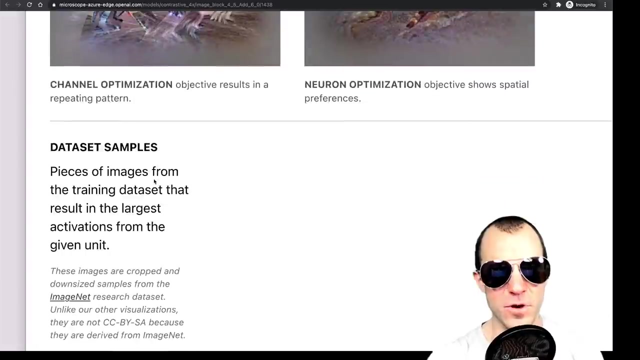 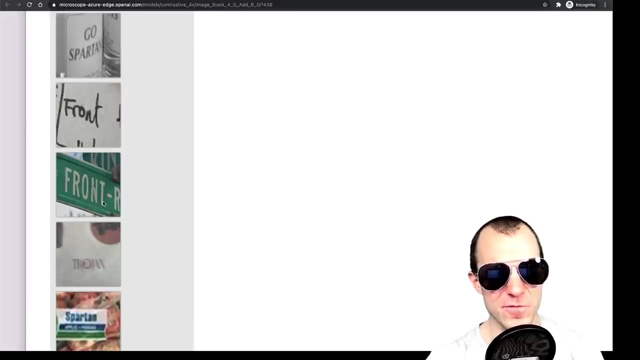 This is feather patterns and leaf patterns. So even when it's in coffee, you see, um, the feather and leaf patterns, even when it's a drawing, it can, it will still respond. This one is strange. So this response to things like Sparta and front and uh, Troy, but so that it responds to rendered front Trojan, Spartans, front. 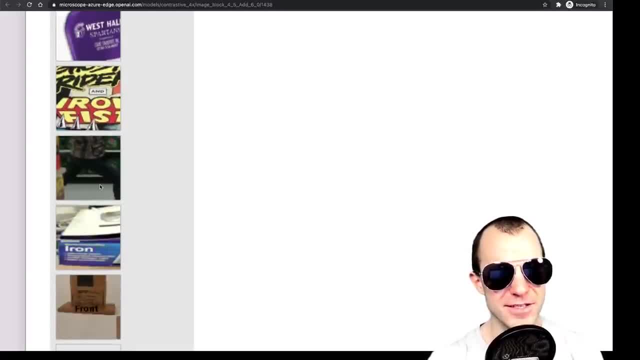 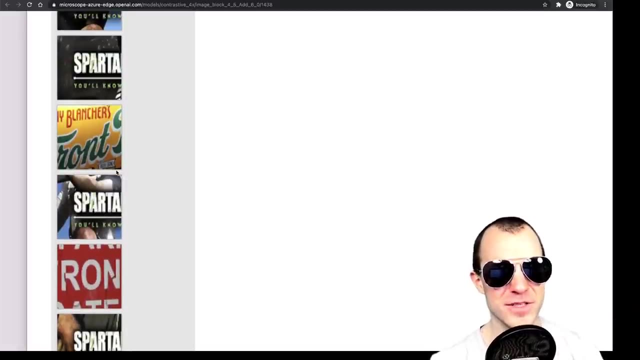 And it also has a lot of people doing sort of squats, as you can see, So um and and fighting. So this is kind of an iron, So this is a bit of kind of a warrior neurons, You can see. oh, there's lots of ah, of course it's because of these Spartan runs and all they're called like this right. 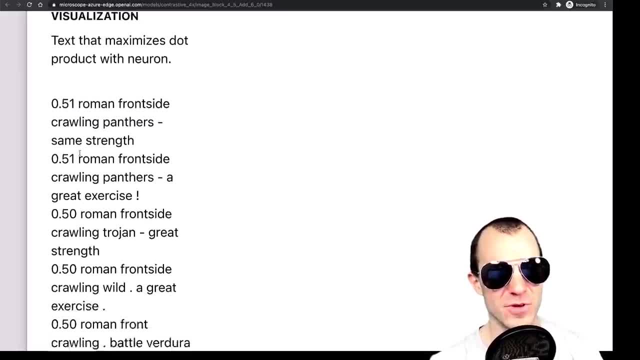 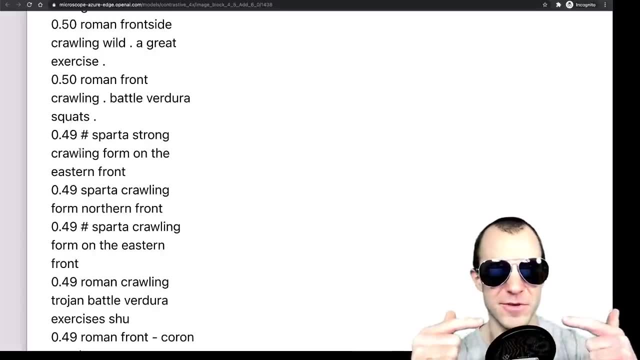 These kind of sporting events. I see Roman front side, Roman Roman. So it connects the workout with the Spartan workout, kind of division, and then it connects the Trojan and so on, via, again via the text, because it makes no sense to connect like the vodka. 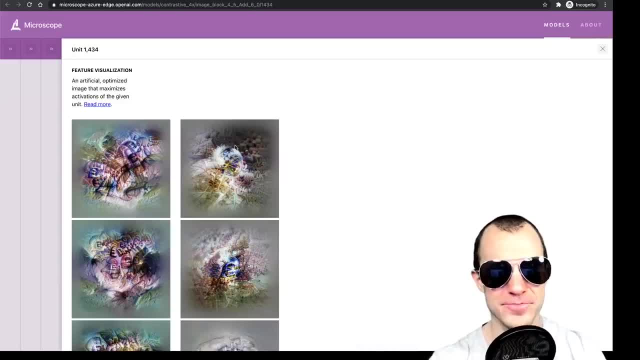 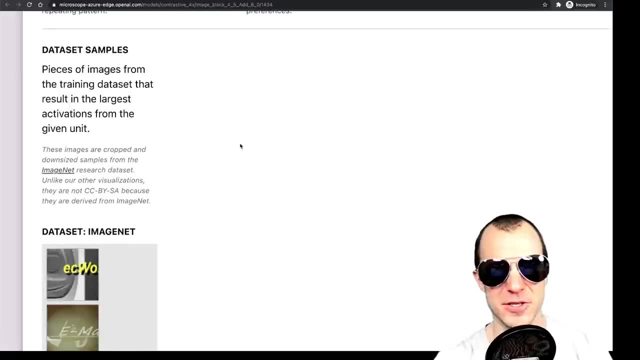 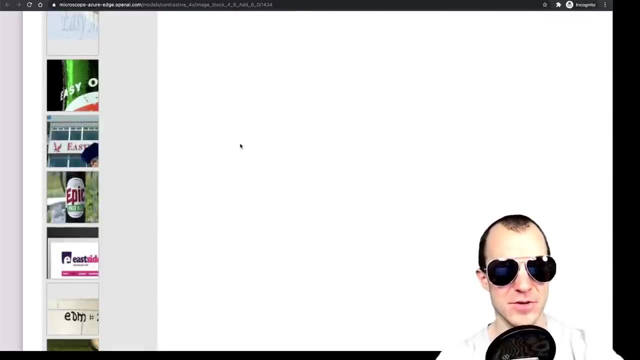 And the and the weightlifting maybe, I don't know. So, yeah, I hope, I hope you're fairly convinced by now. We're going to go a bit faster now, uh, because the video's already too long. but this one here is the letter E, so it's E. response again to rendered text of E. uh, this one here is cleaning. 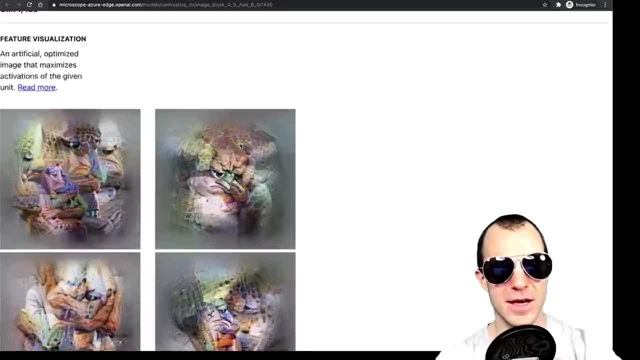 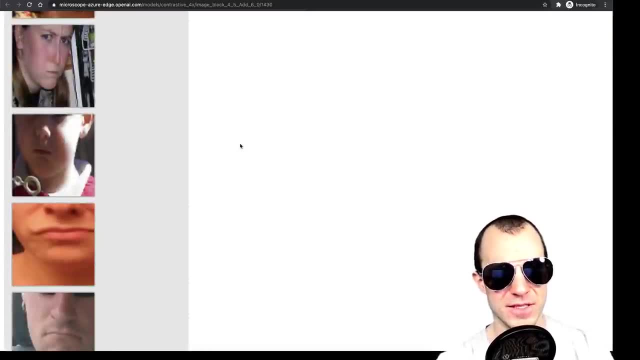 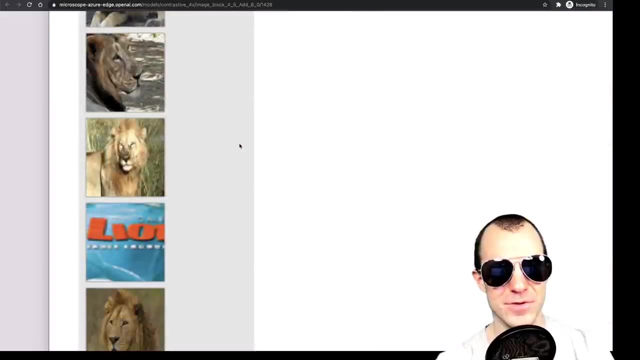 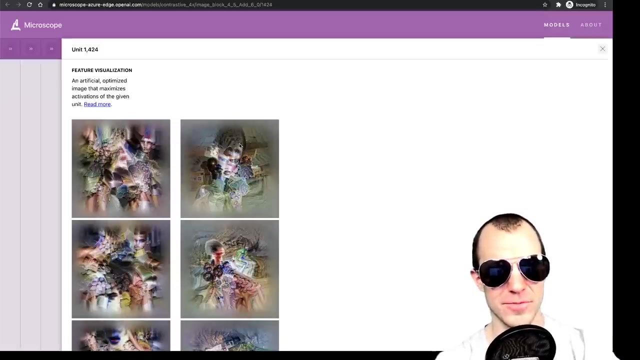 So it responds to cleaning products and cleaning things. Uh, this one here is frown. So this is frowning, frowning, Frowning, grumpy face, grumpy face, um, lion, lion responding to lions. rendered text of lions, team names called lions, and so on. 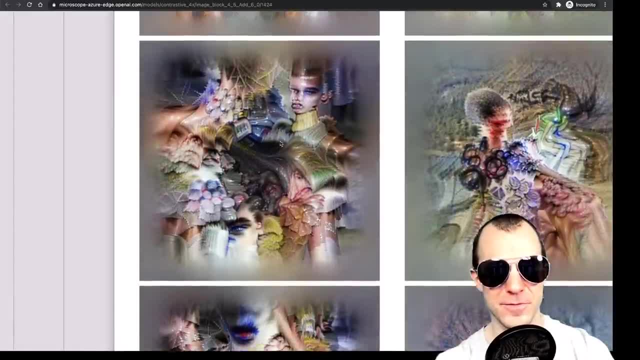 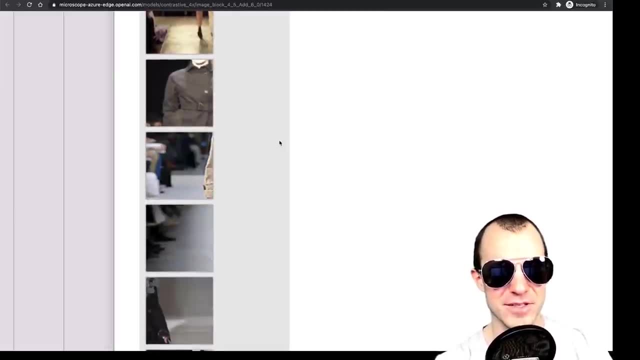 Um fashion model. fashion model- a bait. by the way, the labels are mine. I just looked at them and decided what they are, but you can see like there's a lot of these kind of runway shots Here. um baseball stadium. 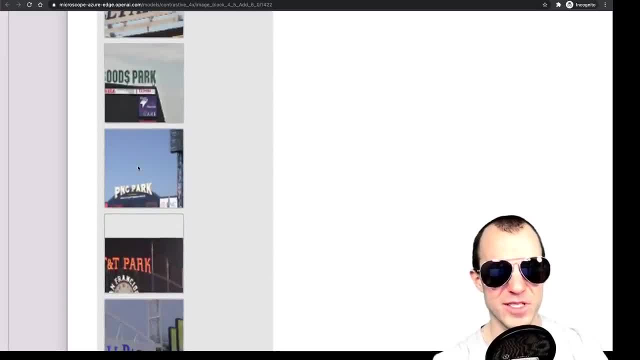 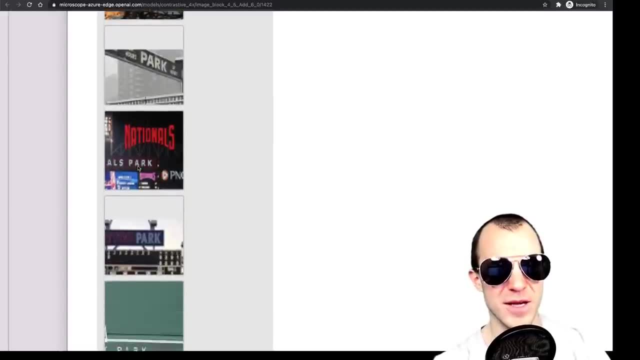 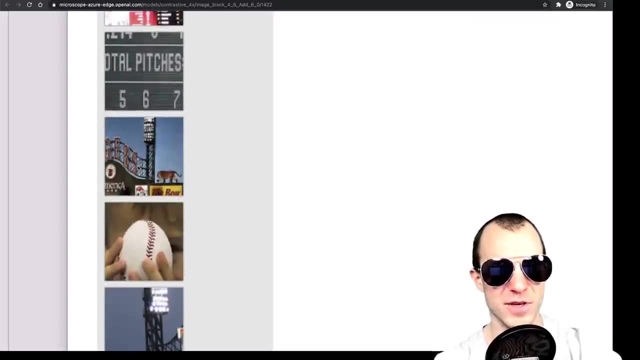 So cool. So these are kind of top views of baseball stadium but it responds a lot to things saying park, PNC park, AT&T park, but also kind of home team, uh, park lights and baseball dugouts and even players- I've seen some players- logos of teams, baseball depictions of actual baseballs. 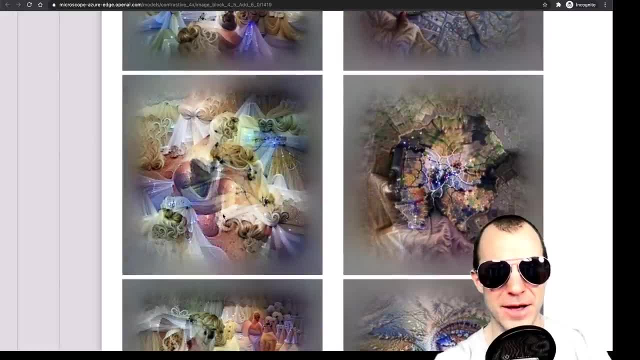 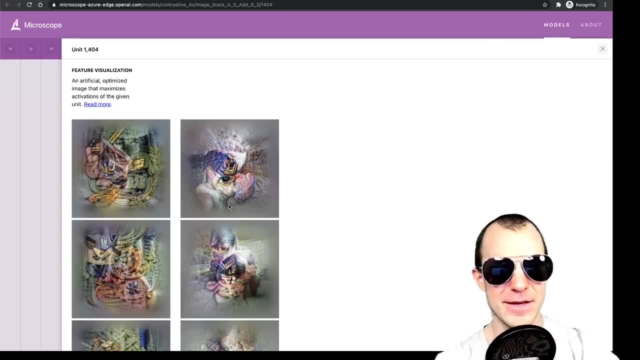 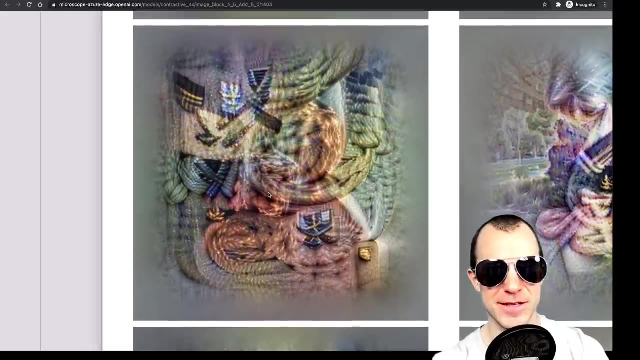 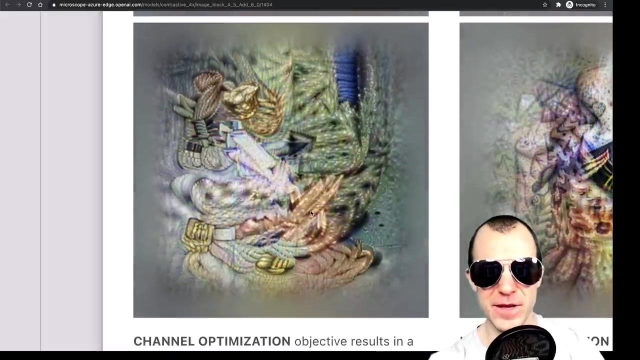 It's immense, immensely cool Here. bride- this is bride, You can see, this is bride. This one, what do you think? This one is Navy. So super cool that it can kind of connect these ropes with the emblems, the, the kind of um, your, your, your tags. 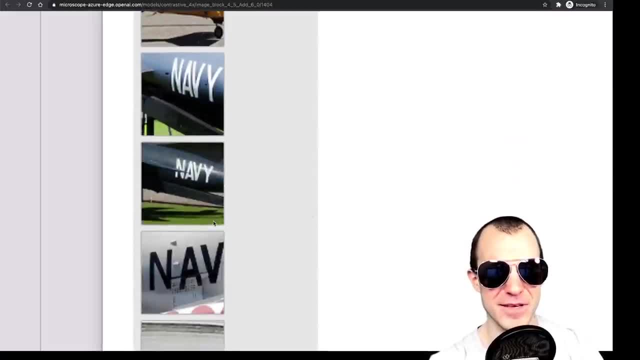 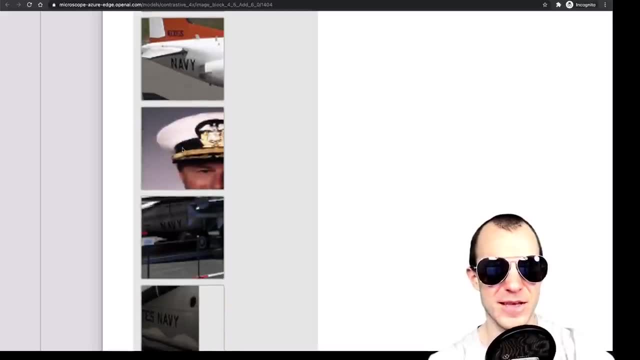 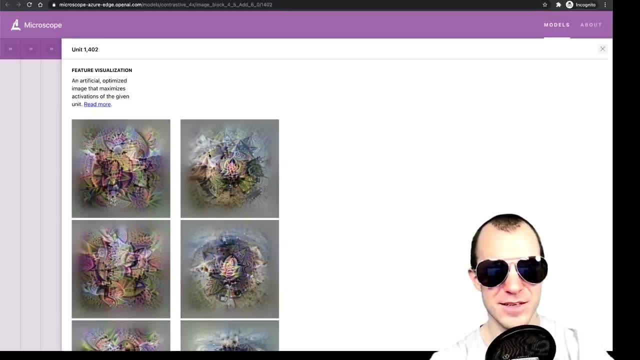 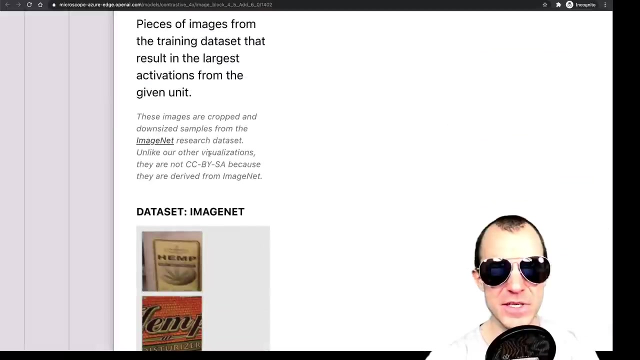 So, and it connected to render texts saying Navy right. So these are the crops of images that it responds to: Navy official, like officers. Navy gravestones- Yeah, So cool. This one, Okay, This for this I also had to look at sort of the um pictures here and the text going along with it. 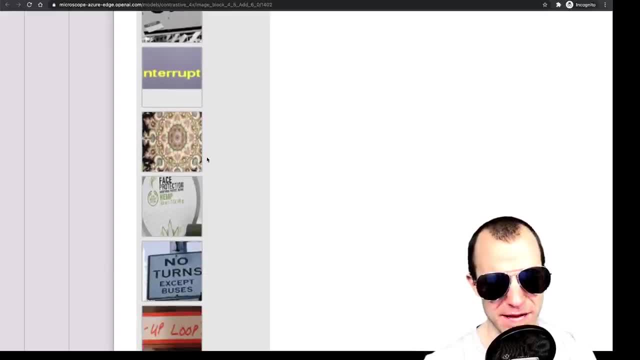 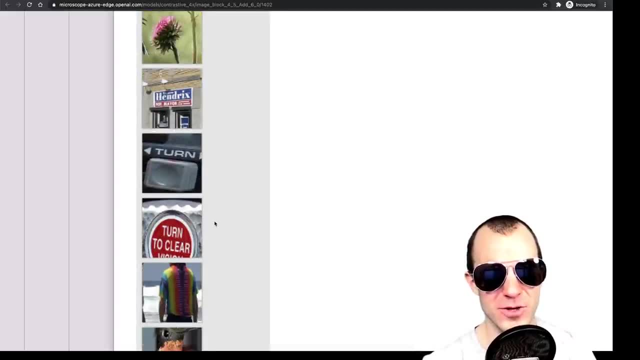 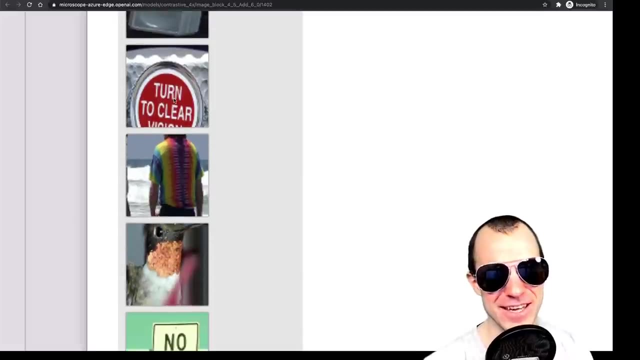 This is hemp, but it is also kind of go up patterns. It is also, for some reason, turn or Okay, Turn um. it is also Hendricks, So this isn't even Jimi Hendrix right Like this. this is definitely connected to these, these goa shirts. 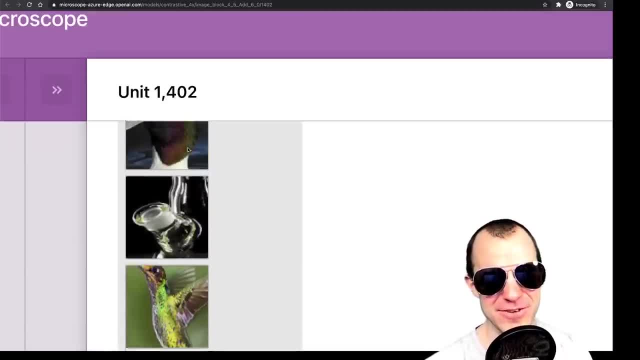 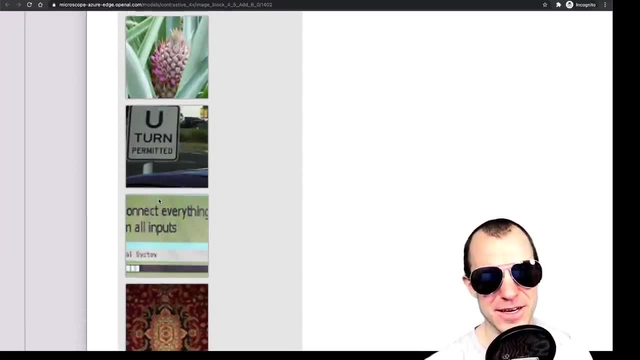 Um, there is also. there's pictures of Jimi Hendrix, which I guess you can understand. There is also um turn again, Where is there's Bob? No, this is Bob Marley. Sorry, This Bob Marley. 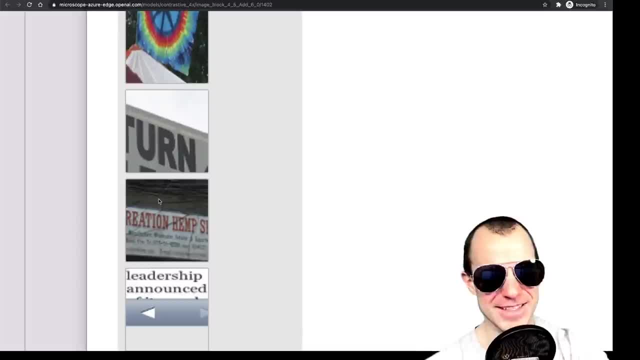 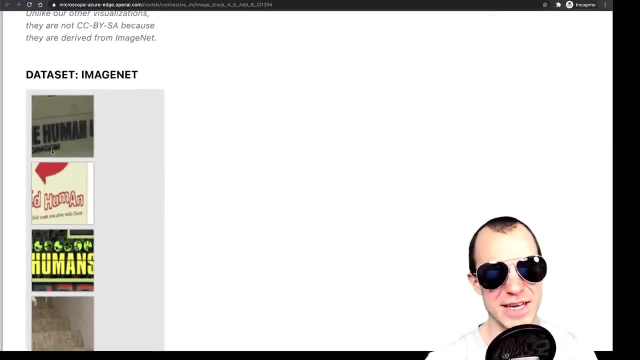 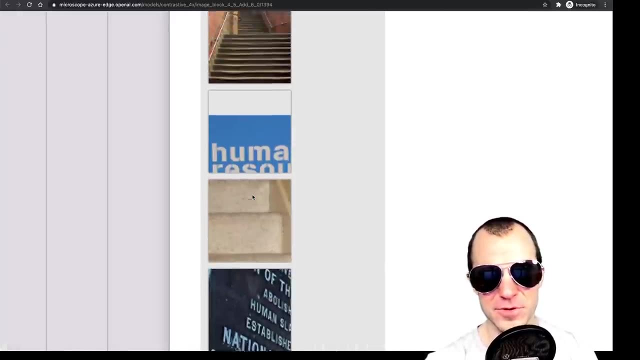 Um, yeah, so so it connects these things, uh, staircase, and here, for some reason, also responds to text rendered human, um, and to staircases. and here I have, I don't know why, but there's, there's this thing which I'm not sure. 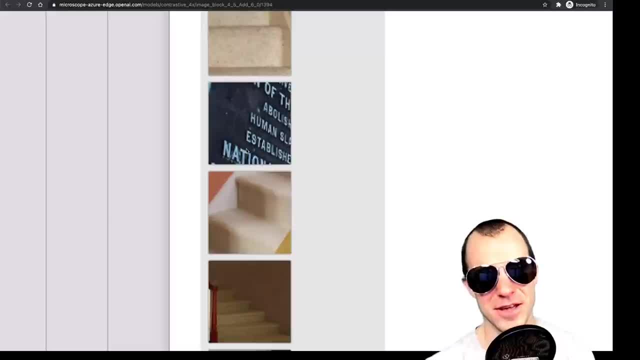 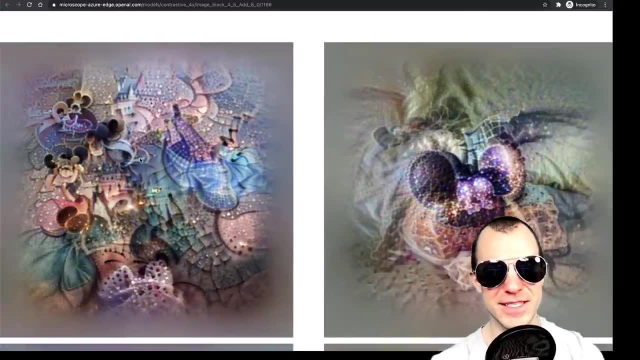 So it has human in it, but it does also arrange like a staircase, So maybe that's why it responds extra, extra. Uh, yeah, the Disney neurons. This is a Disney neuron. How cool is this? How cool is this? 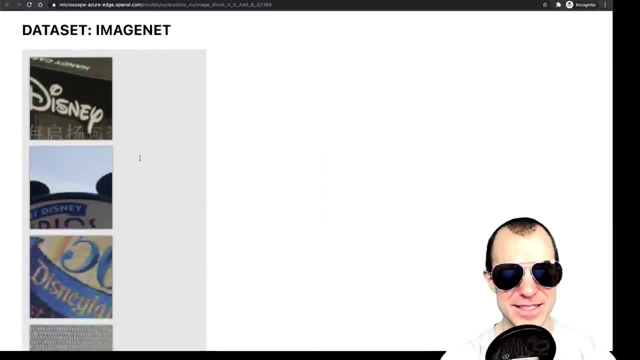 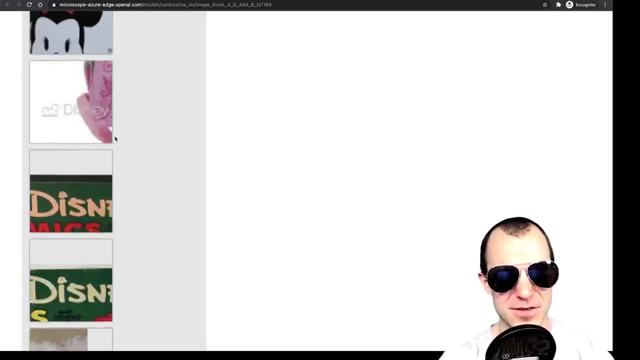 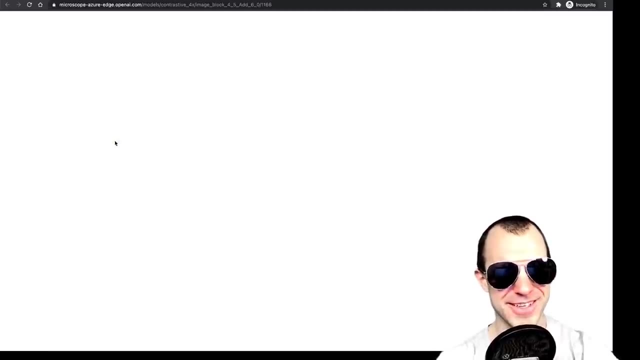 So you can clearly see that, that, but then it you know, Disney, these are the samples that it responds to simply something saying: Disney, the Mickey mouse ear, the mini bow, um, you know, immensely cool The, the castle right. 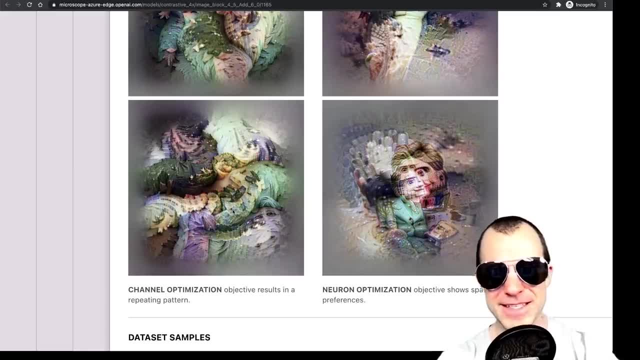 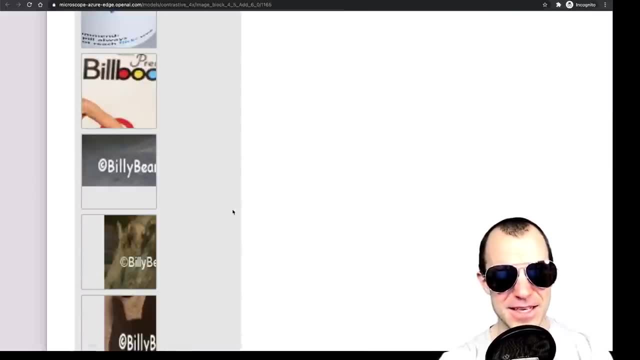 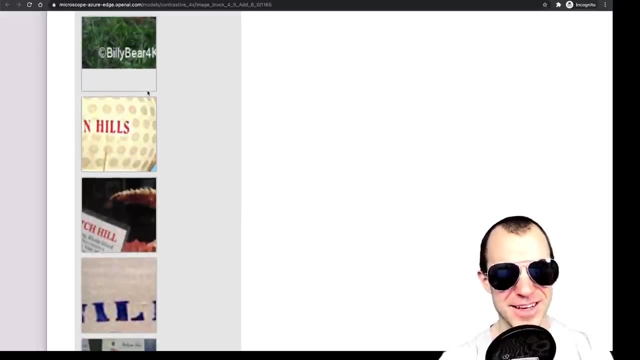 The Disney castle. This is the Hillary Clinton neuron Can see it. You can see this is Hillary and the images it responds to is Hillary Hill pill, Polly Hill pills. So this is maybe it's more like the LL. why the ILL? why neuron? 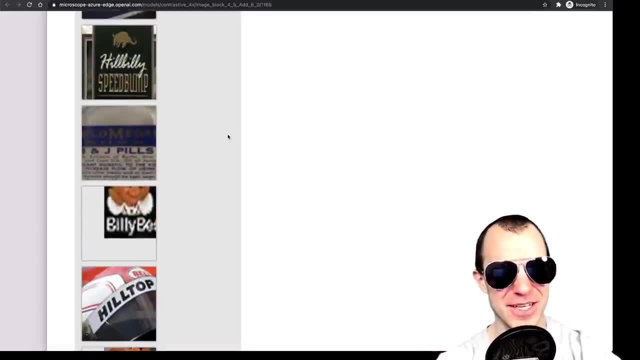 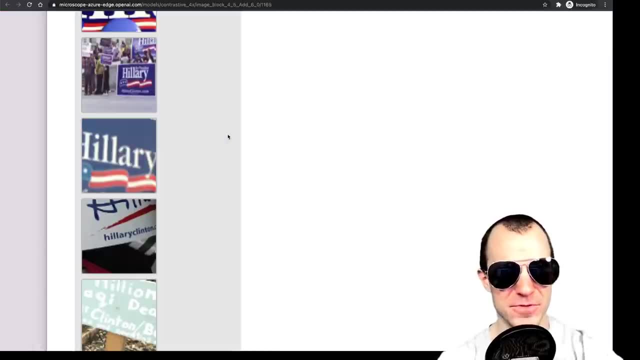 Uh, but it it does, uh, pick out Hillary Clinton as well. Yeah, So Image net, of course, is older than At least One of Hillary's campaigns. I'm not sure This is God, So I found this one. 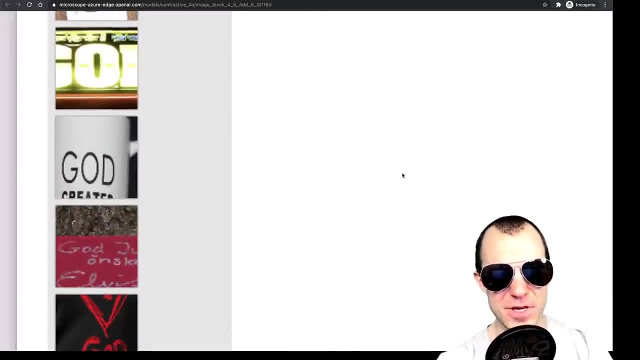 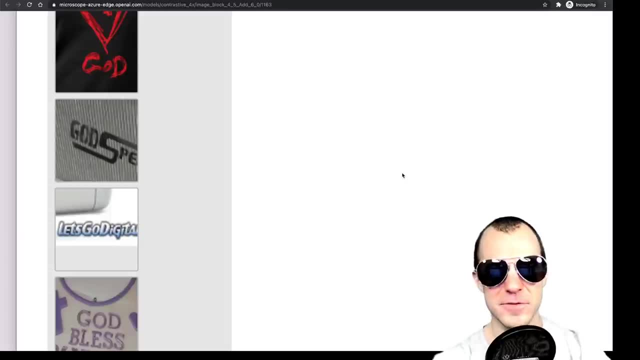 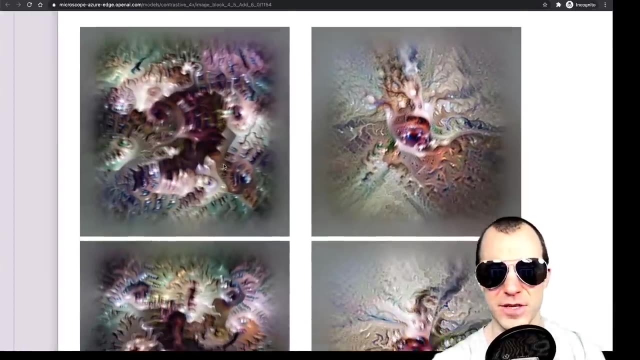 This is: yeah, God, if you so the reconstruction process. it's not very good at generating text. uh, maybe because so they have a lot of priors in that. If you look at the reconstruction article, um, you can probably- and they do this in in this article- they reconstruct text, but it's still not super clear. 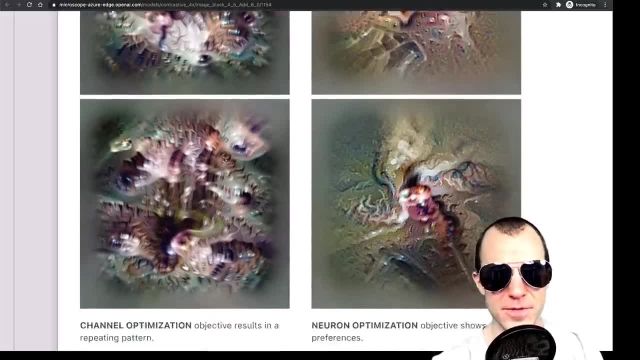 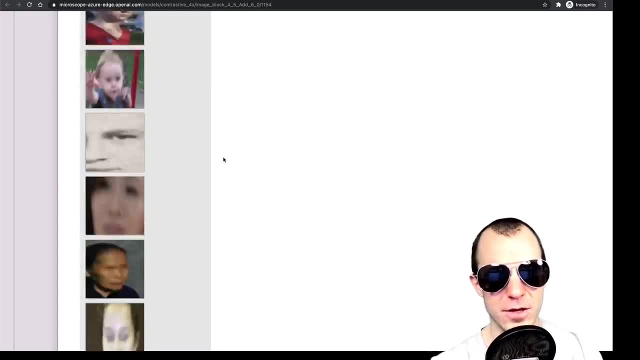 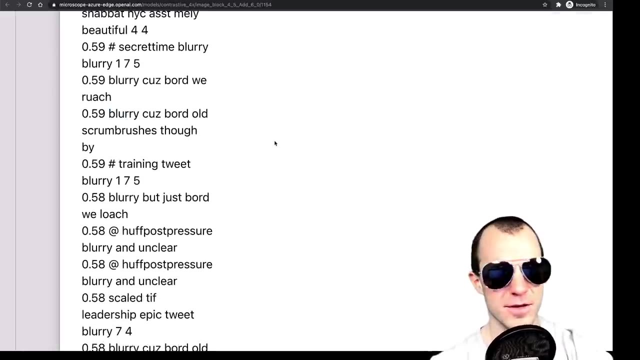 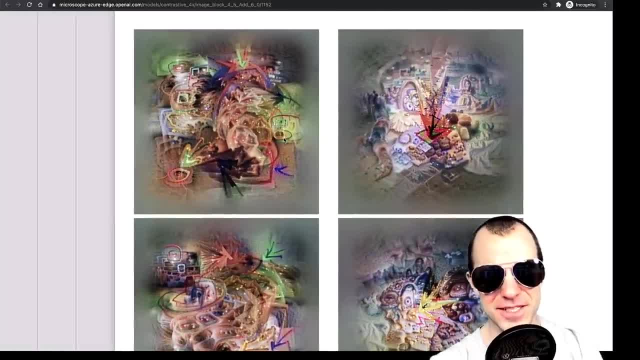 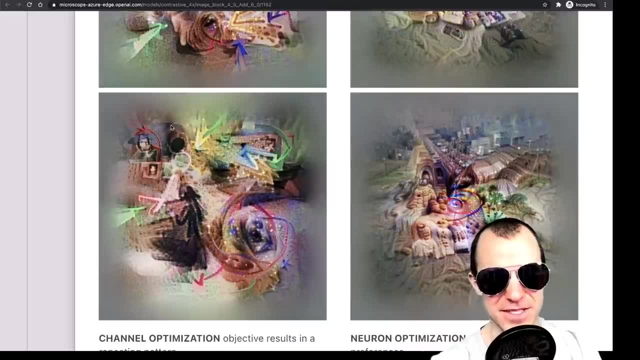 Like it's not even what's on the image, but you can clearly see like this comes from the other description. This is hand drawn arrows, or arrows in general. He, this looks like my videos now. right, Like this recognizes arrows. This is hand drawn arrows, or arrows in general. This looks like my videos now. right, Like this recognizes arrows. 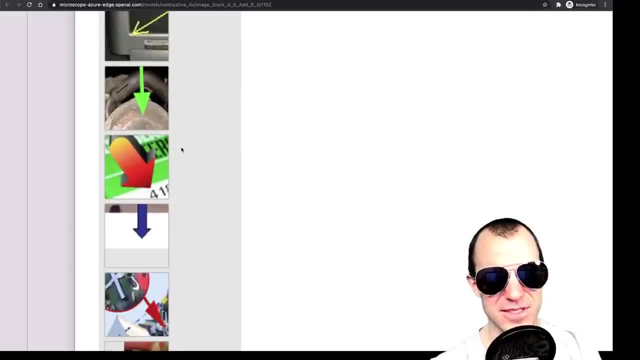 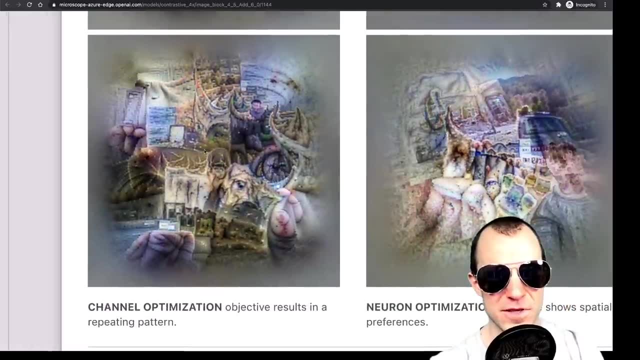 This is hand drawn arrows, or arrows in general. This looks like my videos. now, right, Like this: recognizes arrows, Specifically, uh, you know, kind of collary arrows. This one, what does it do? This is presenting a trophy. 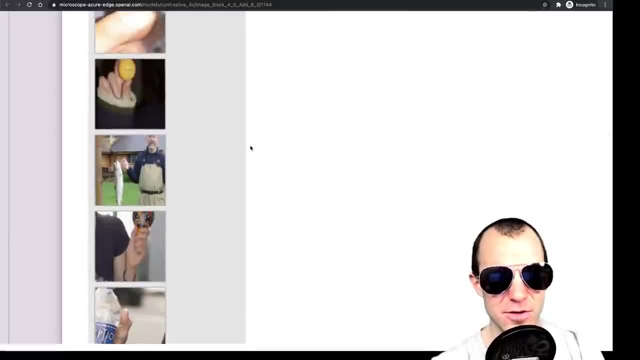 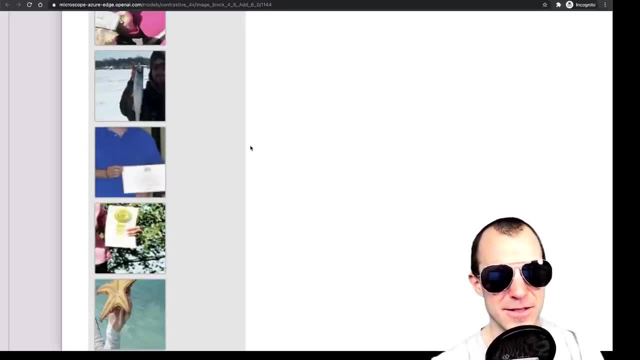 You see this one here in the middle. this is kind of so. these are, all you know, people presenting some kind of thing, holding some kind of thing in their hand, showing it like fishermen or diplomas. Um, this one I was amazed by. 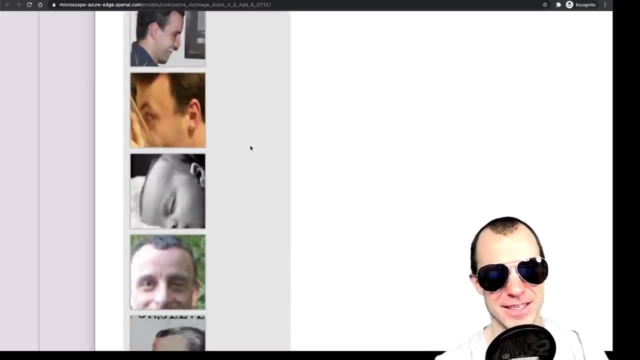 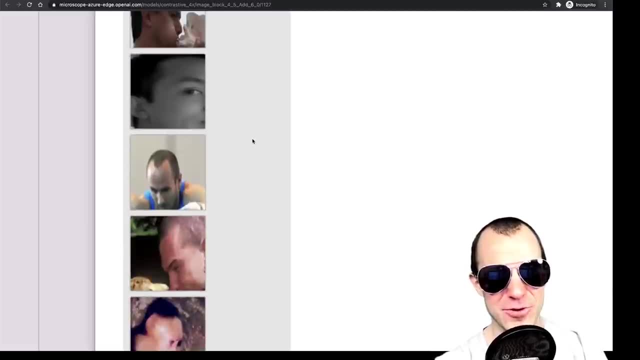 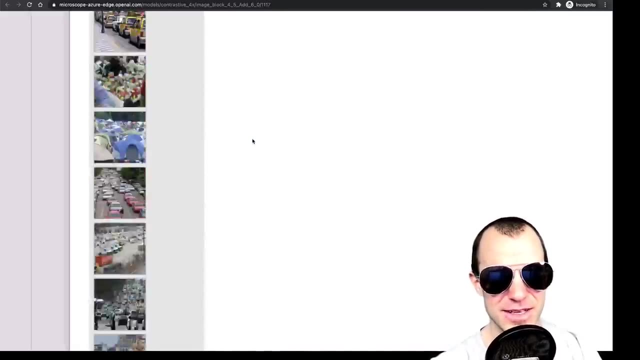 This is a neuron responding to Receding hairlines. like it responds to receding hairlines. How cool is that? How cool is that? Uh, this is traffic tent and so on. So it responds to tents and traffics and crowds of people. 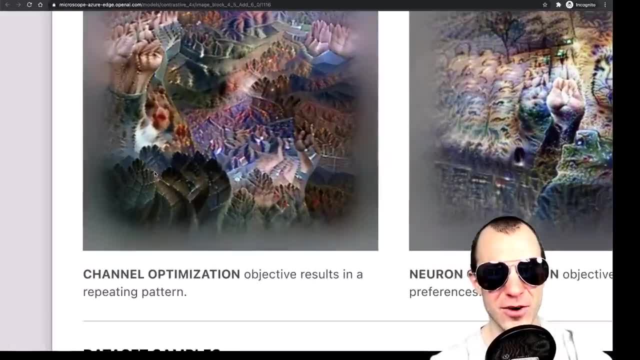 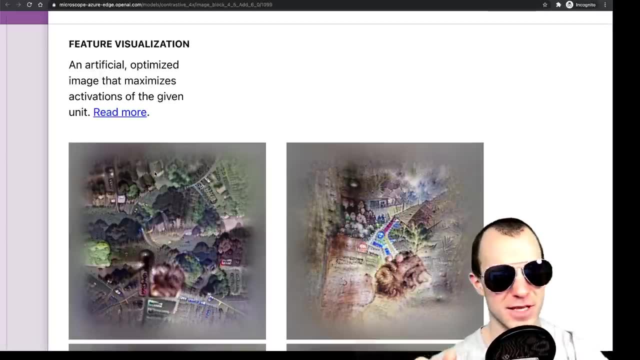 This one is um raised arms, but also pancakes. So pancakes and raised hands. For some reason there's a connection. No, but I mean these, these models. they still overload when they can. This one, how cool is that. 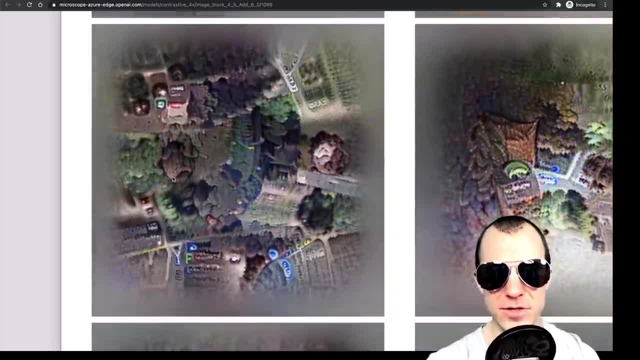 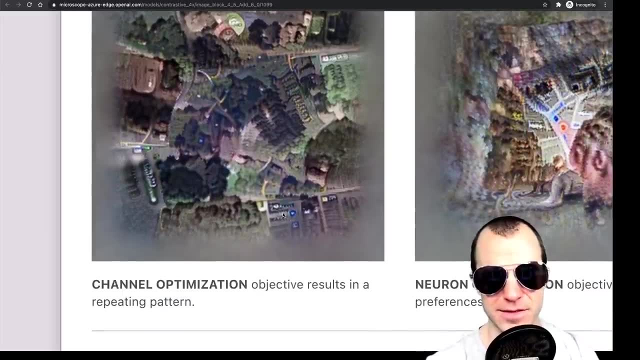 This is the Google maps neuron. These, these are reconstructions. These are not samples, These are reconstructed. You can see it's clearly. it has kind of the street labels and the pins on it. So this is a Google Google maps, like neuron. 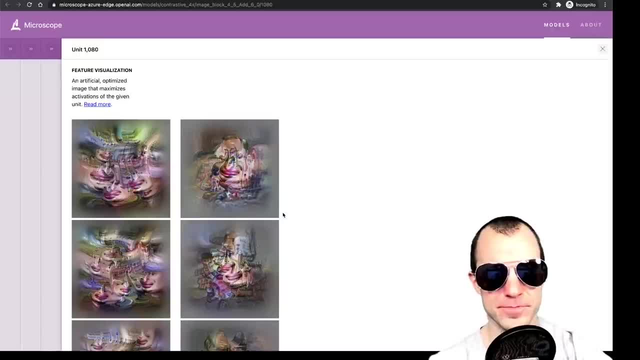 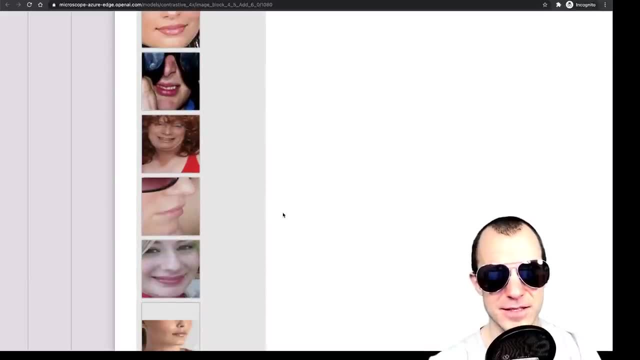 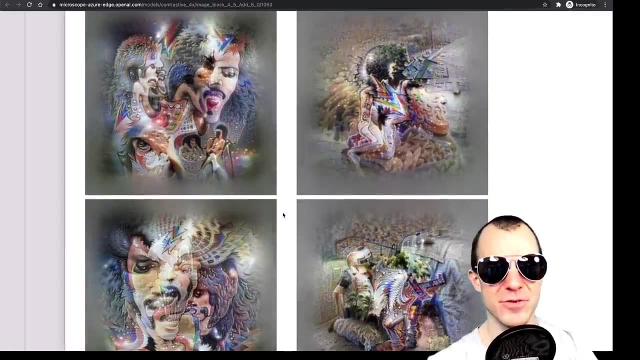 What So cool? This one I call nervous smile. You can maybe see that it's like: uh, yeah, Uh, here's Elvis. This is the Elvis neuron. Uh, I know it sort of it also looks like Hendricks a bit, but the uh things. 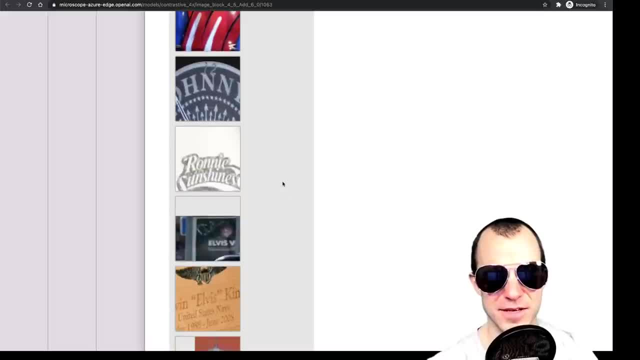 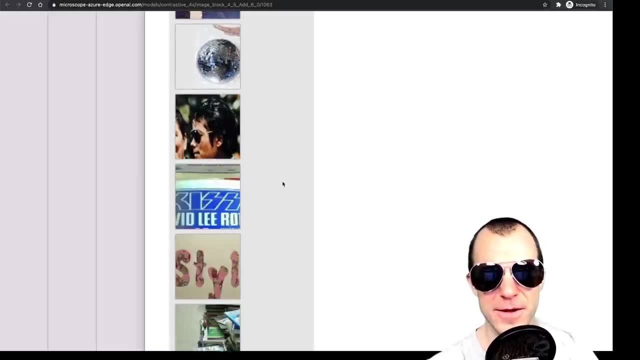 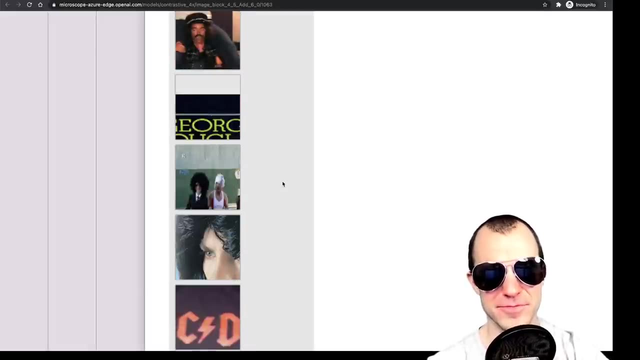 it connects it to is that's not Elvis. That's not Elvis. kiss. Okay, Maybe it's not exactly Elvis, Maybe it's more like a pop star neuron. Uh, yeah, maybe it's not Elvis. uh, only Elvis. Billy Elliot. this one is the flash right. 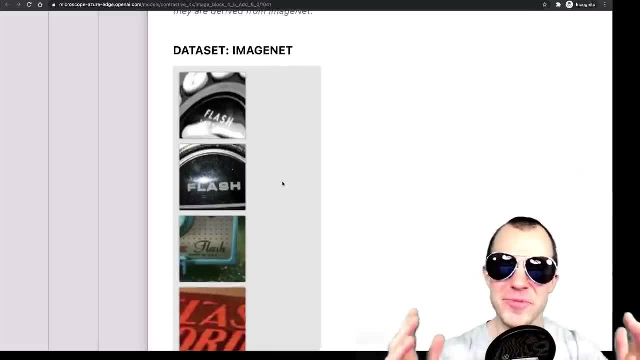 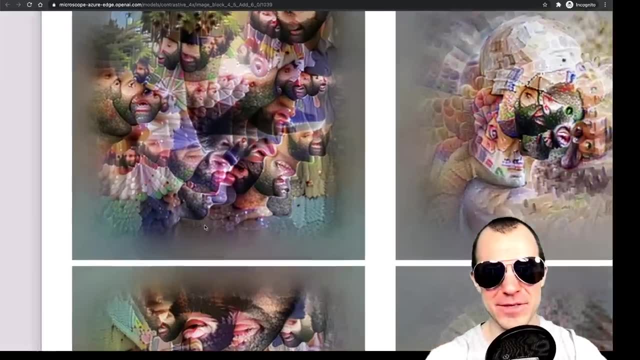 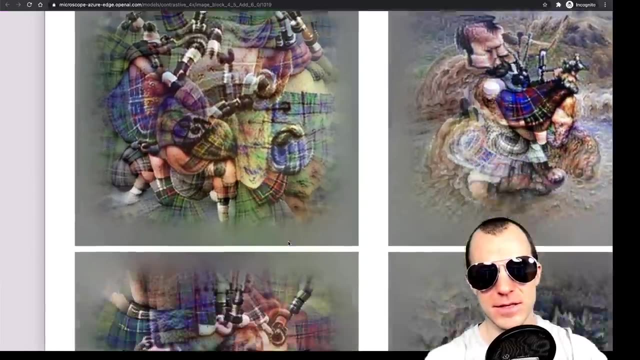 That's the flash And the cool thing is it responds to images saying flash: What, Okay? Beards? responds to beards: generally, beards, lots of beards. kilts, kilts and bagpipes. response to guilds: kilts and bagpipes: rainy. 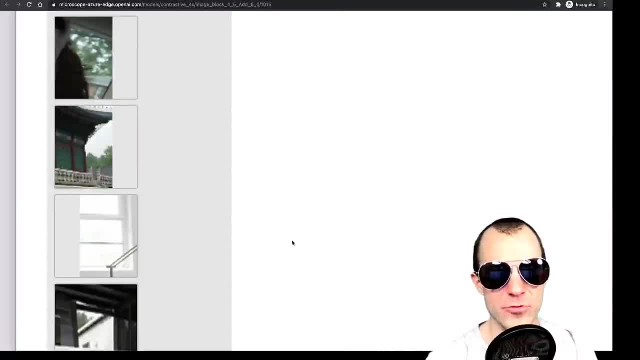 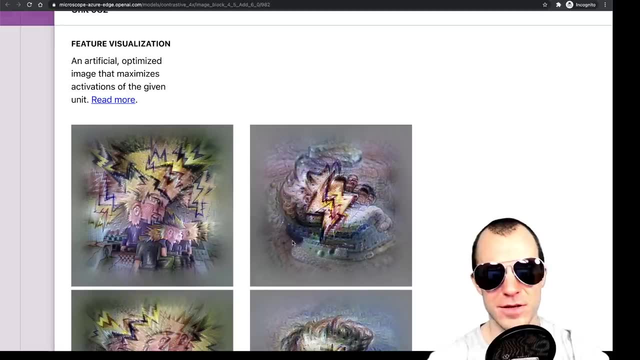 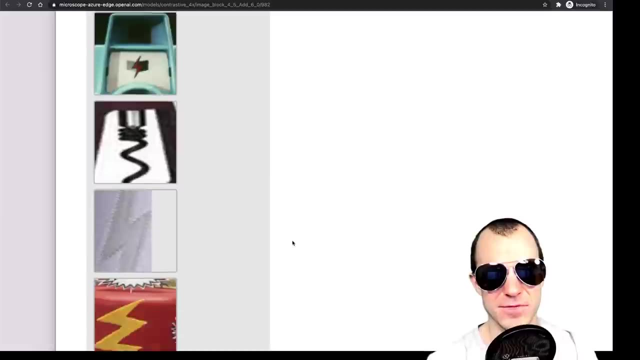 This is a neuron that responds to things that are rainy, rainy days. So you can see here out the window it's raining, rainy windows, So cool. This is flash and electricity. So you'll see like symbols, these symbols of these flashes, but also kind. 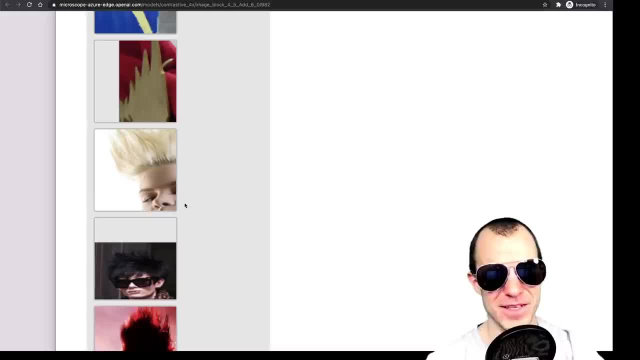 of electric hair curling up Um so. 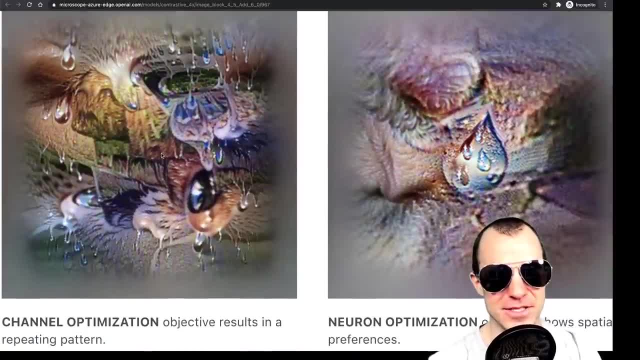 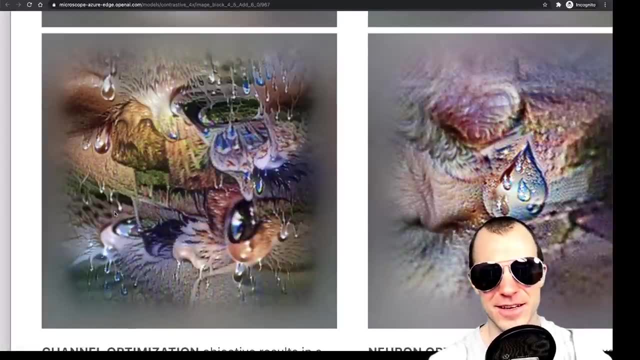 How cool does that look like? that's just cool. And the occasional image net reconstruction thing where there must be like half a dog face in there, that is just trippy. This one is, this one is escape. 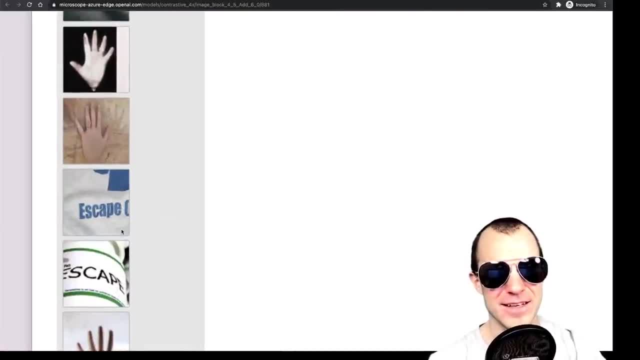 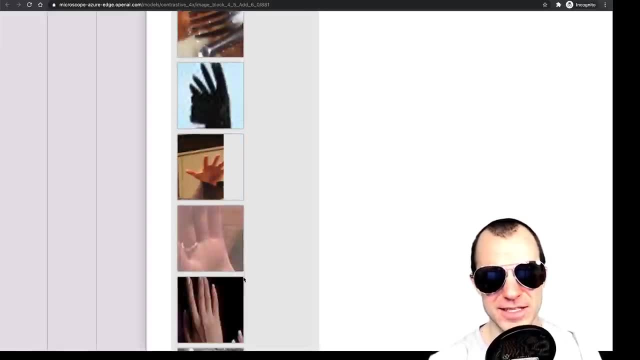 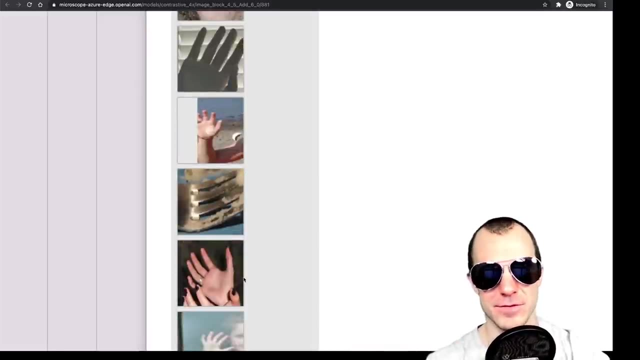 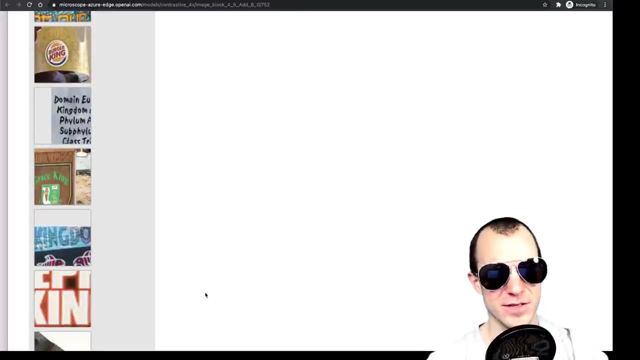 Okay, escape, like, look at that, Like to connect these things. How long would you like without contrastive learning? how well, i guess if as long as you have images and labels, but still king, this is king, so the depicted are crowns. but response to renderings of king: 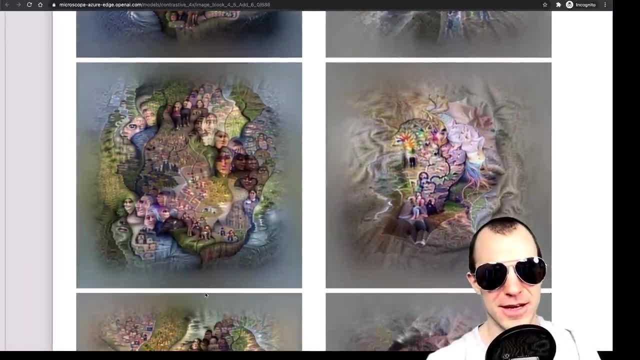 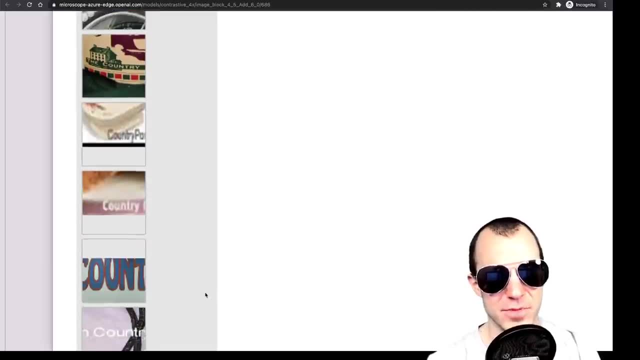 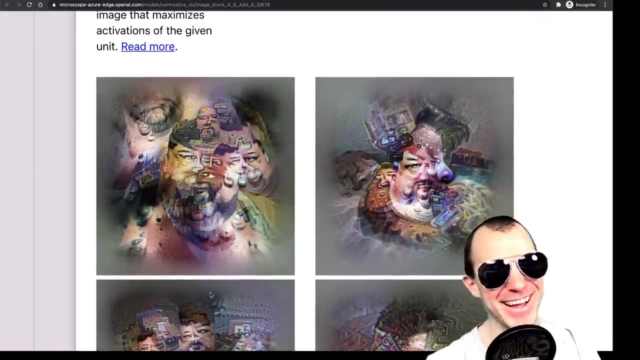 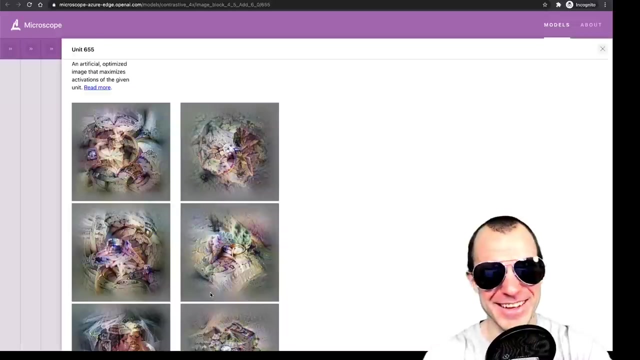 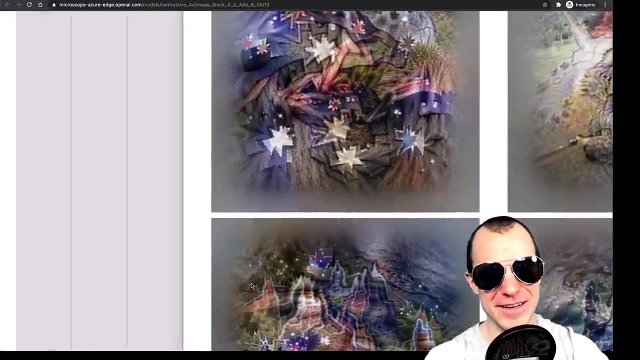 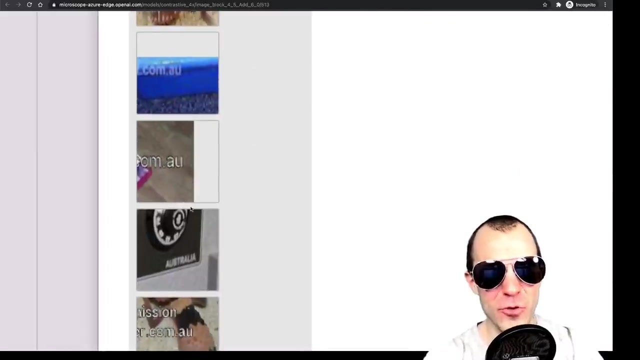 this is nation. how cool is that nation response to country, country, country. oh, it's country, not nation. but still, this one responds to overweight men. there's a neuron that responds to over phases of of overweight men. um, this one is wedding, this one is australia, and the cool thing here is that it responds to rendered domain names of australia.